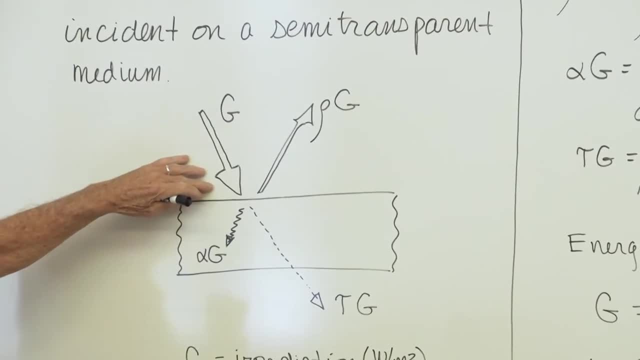 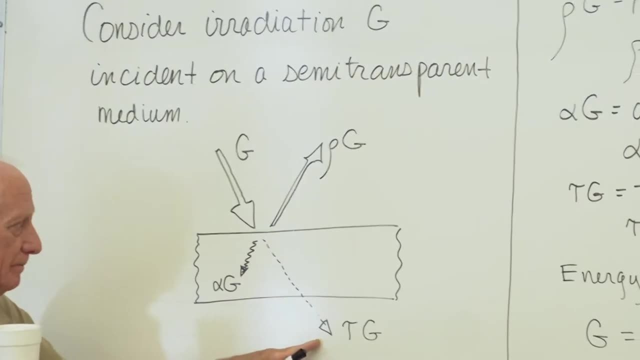 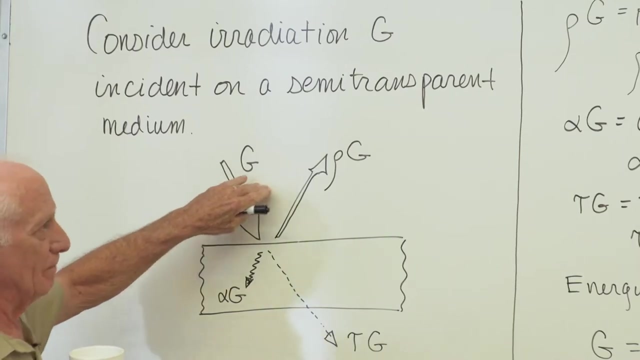 That incoming radiation strikes a surface. Some of that can be reflected- rho times G- Some of that can be transmitted all the way through the media and some may be absorbed- alpha times G. So we have incoming radiation. G can end up in three different possibilities. 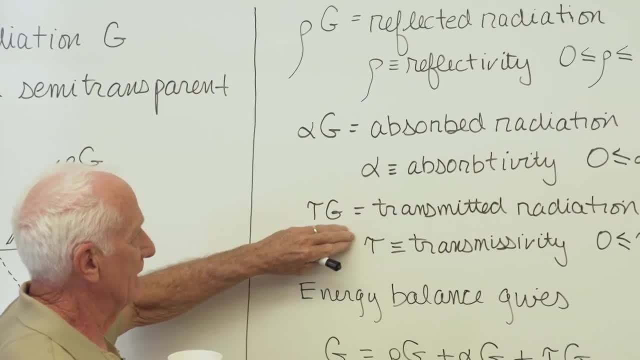 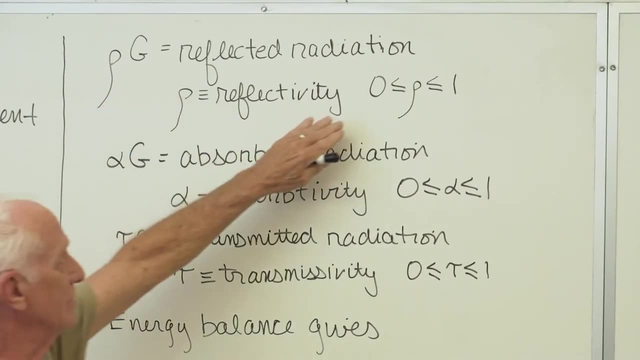 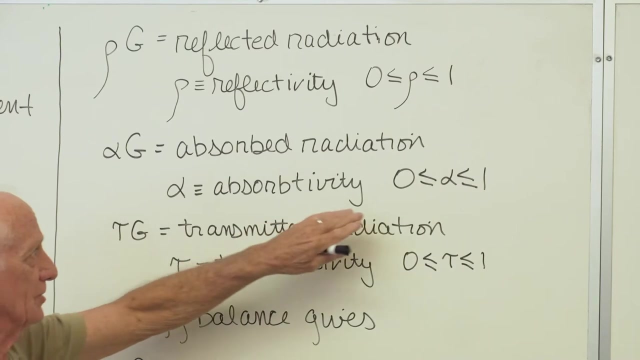 reflected, absorbed or transmitted Rho times G. rho is reflectivity dimensionless between zero and one. Absorbed alpha times G. alpha is absorptivity dimensionless between zero and one. Transmitted radiation tau times G. 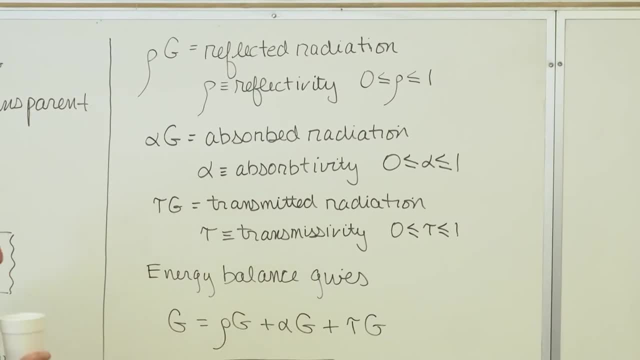 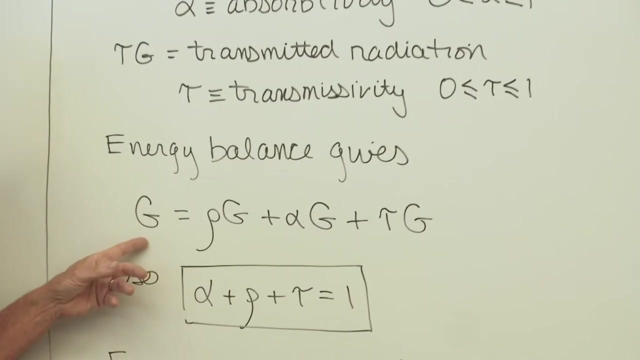 tau, transmissivity, dimensionless values between zero and one. We then write an energy balance on that surface: What comes in for steady-state goes out no generation. So we get incoming radiation G, called the irradiation equal the reflected. 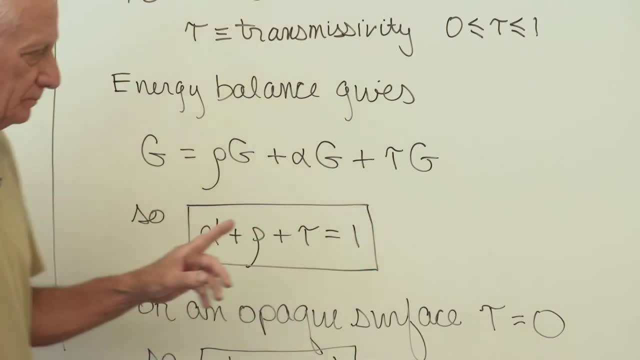 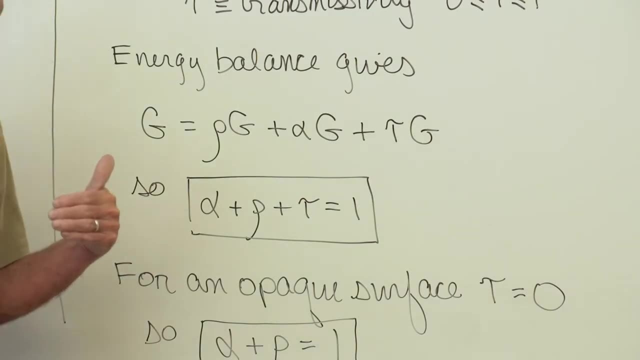 plus the absorbed plus the transmitted, Each term contains G. divide through by G, We end up with a relationship between three surface properties: alpha plus rho plus tau, equal one If the surface is opaque. the word opaque means the transmissivity is zero. 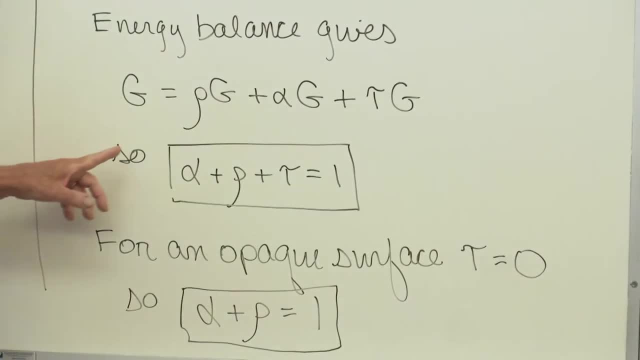 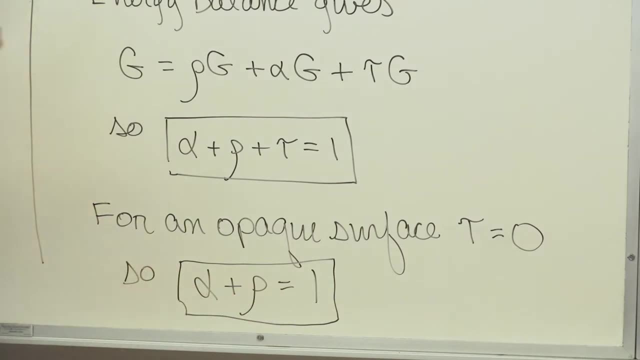 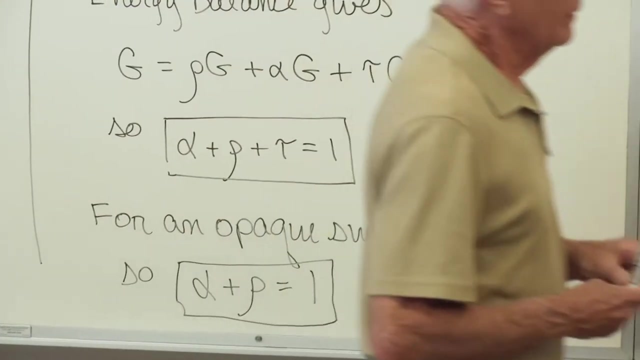 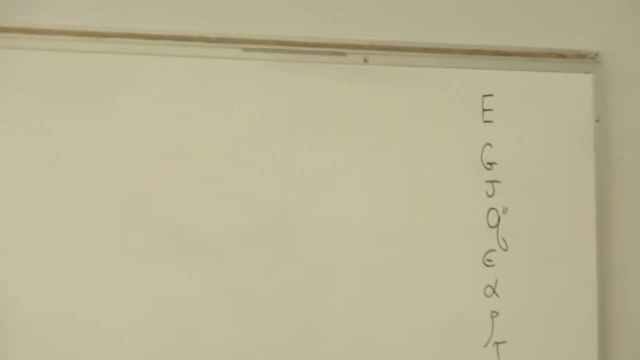 nothing gets through. If the surface is opaque, tau is zero, he goes out. so alpha plus rho equal one. These two equations of course relate surface properties. Yeah, there they are Now. so far. here are some of the properties. 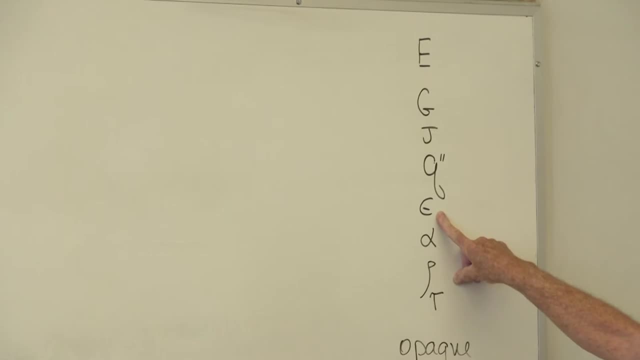 The emissivity epsilon dimensionless between zero and one. If it's one black body, Alpha, rho, tau, Opaque surface tau equals zero. Emissive power capital E G. irradiation capital G Okay. 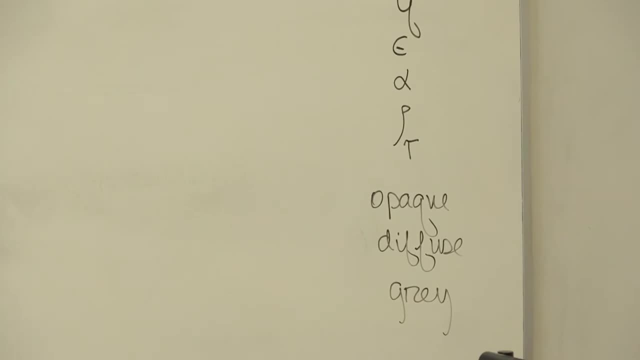 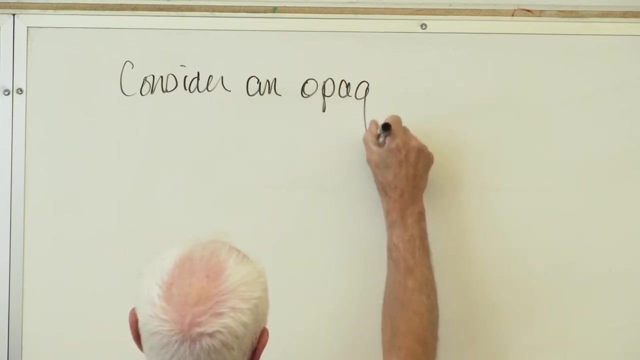 Okay, Now we take a look at J, So we're going to look at capital J. To do that, we'll look at a surface. So here's our surface Now. first of all, the surface can emit radiation, Okay. 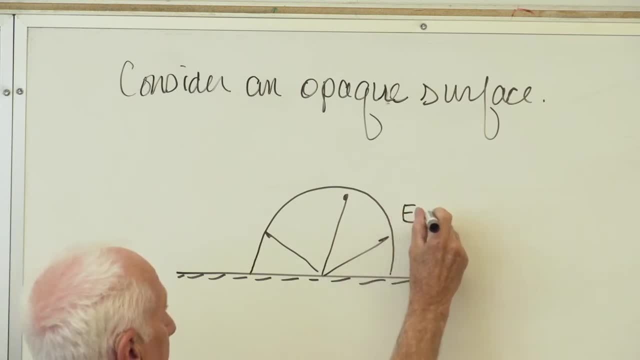 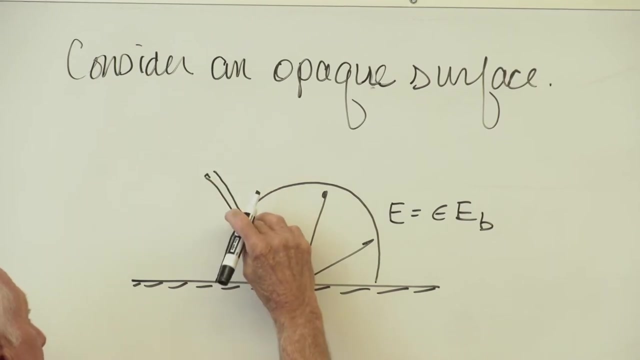 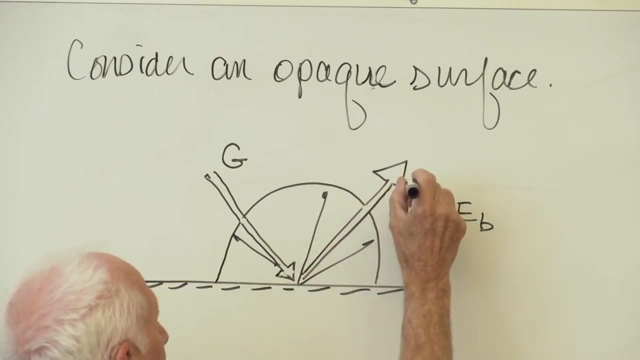 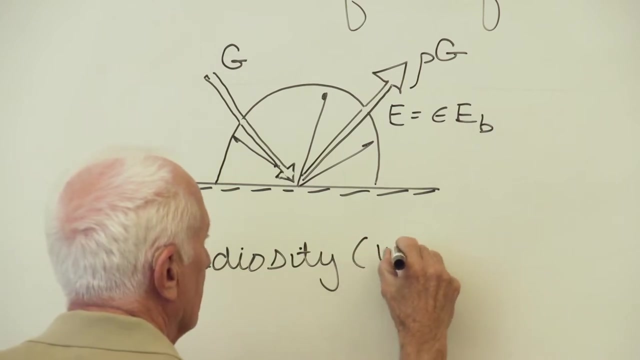 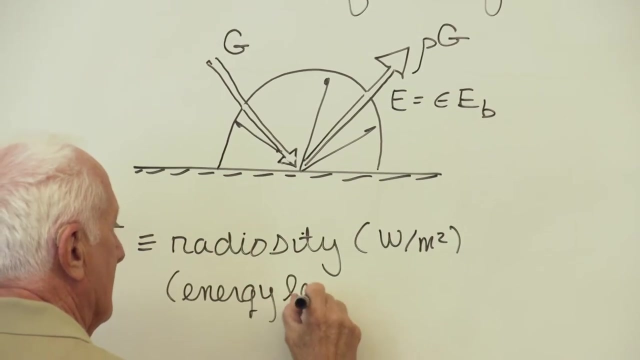 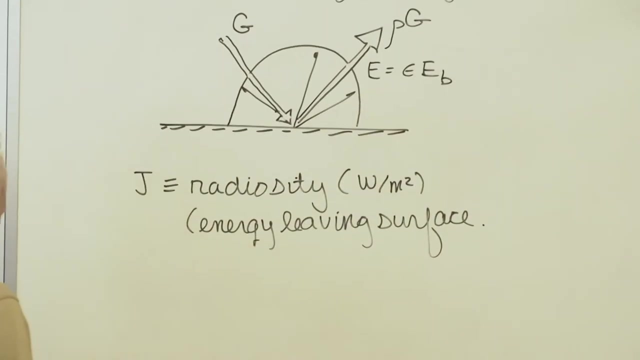 This radiation is E, which is epsilon E b. Now a surface can also reflect some incoming radiation. G comes in. this amount goes out: J radiosity, watts per square meter energy leaving surface. There's a picture. 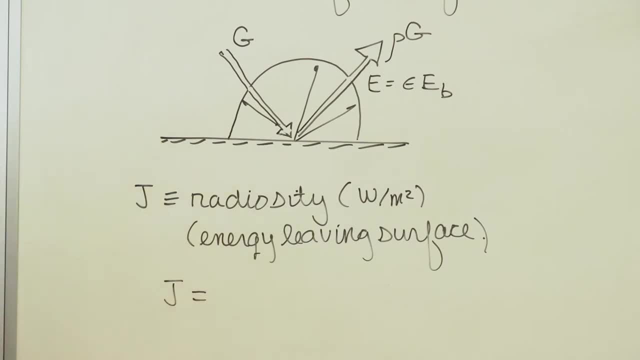 so pretty straightforward. First of all, energy can be emitted by the surface due to its temperature. Okay, Epsilon E b. Second of all, energy, energy can be leaving the surface due to reflection. Okay, row G, So there's J. 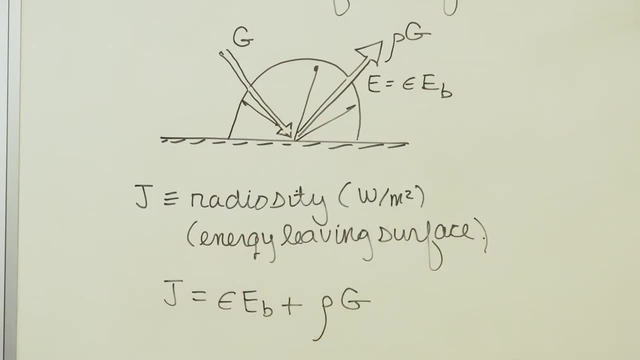 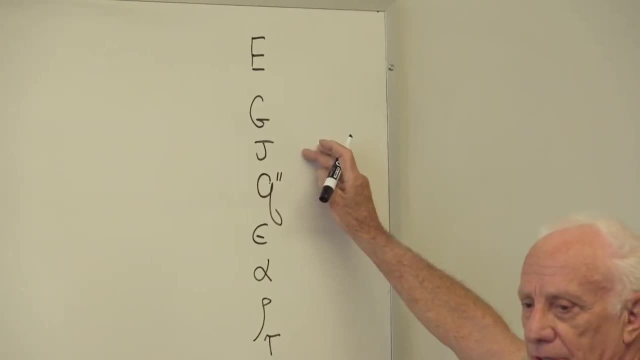 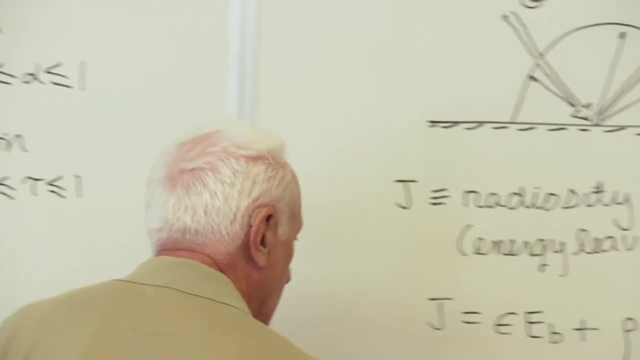 Now J radiosity. So add one more capital letter over here We now have capital E, capital G, capital J. They're all watts per square meter. They mean all different things, of course. Now we add another one, Q, double prime. 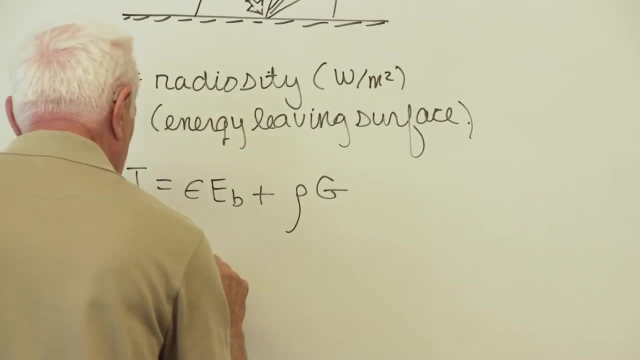 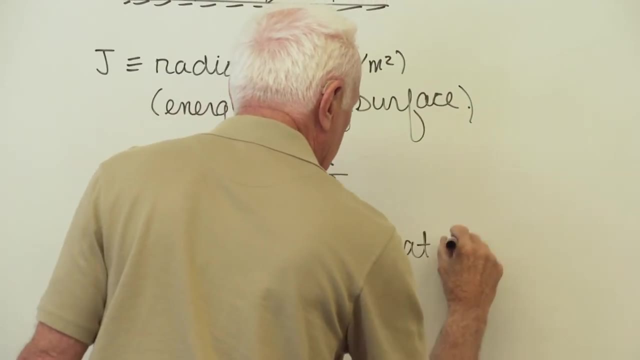 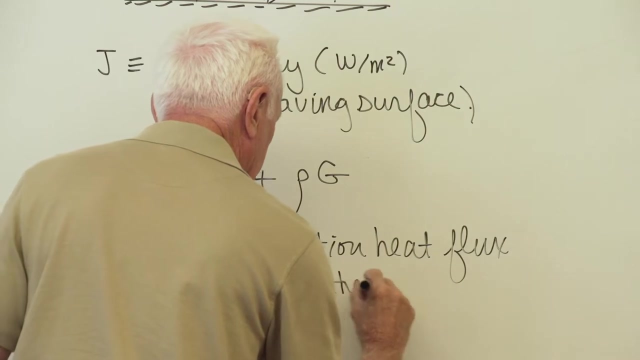 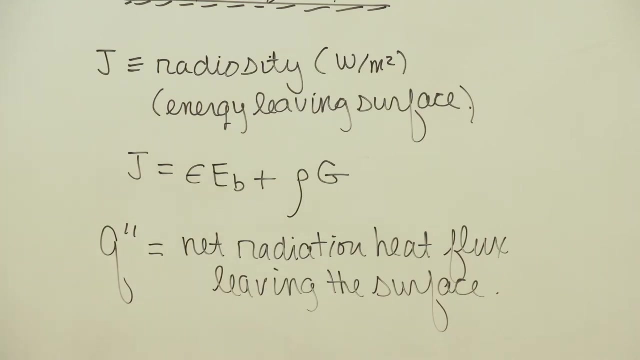 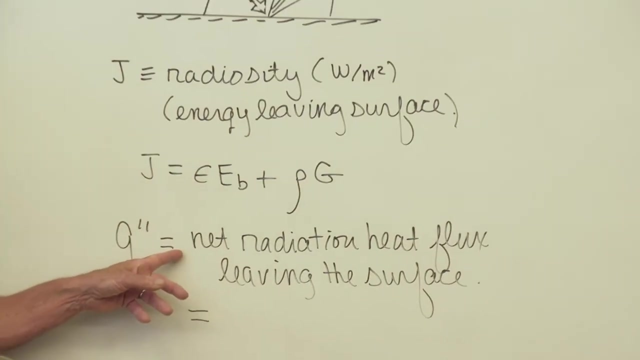 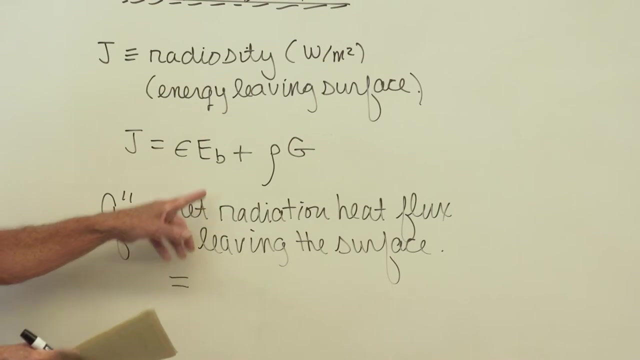 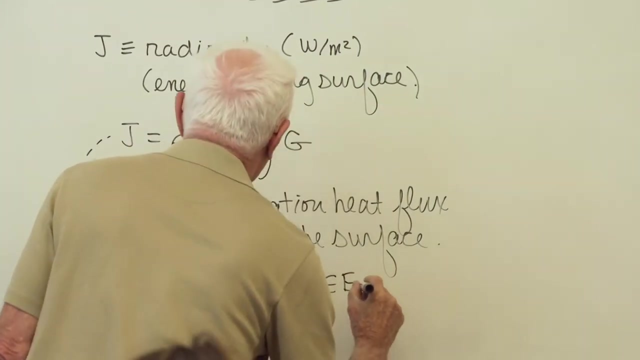 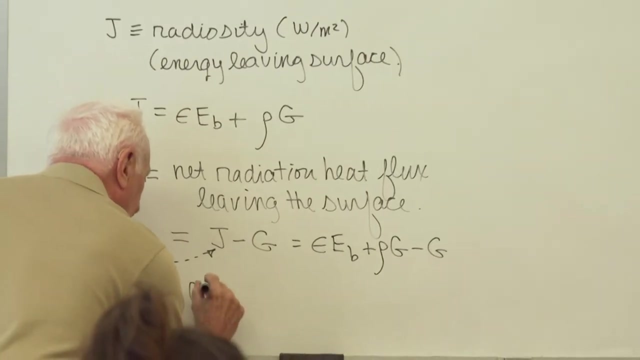 The net radiation, heat flux. leaving a surface Net means subtract something. Leaving net means subtract, Leaving minus entering. Here's the picture: Leaving J Coming in G. There it is Put in for that J, this Q double prime. 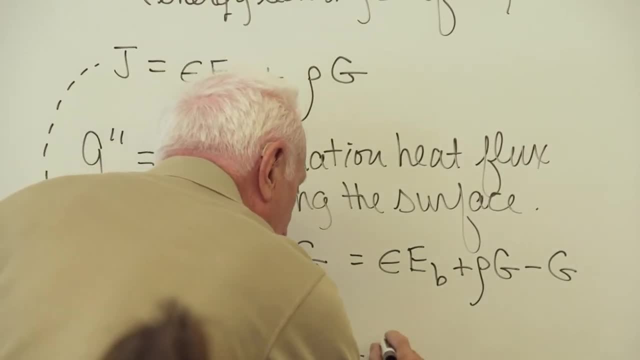 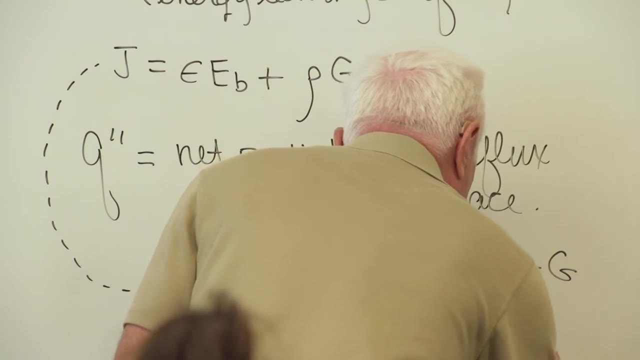 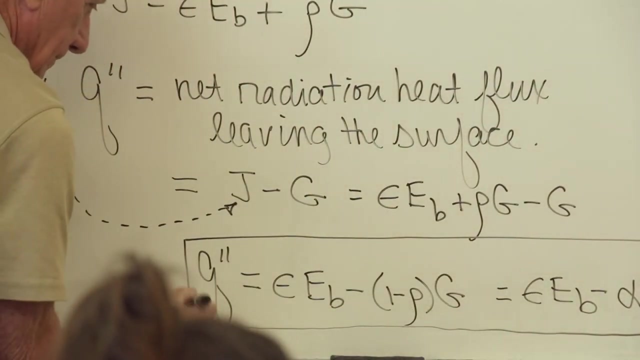 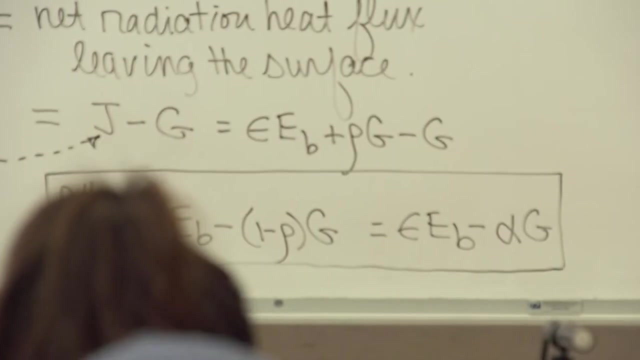 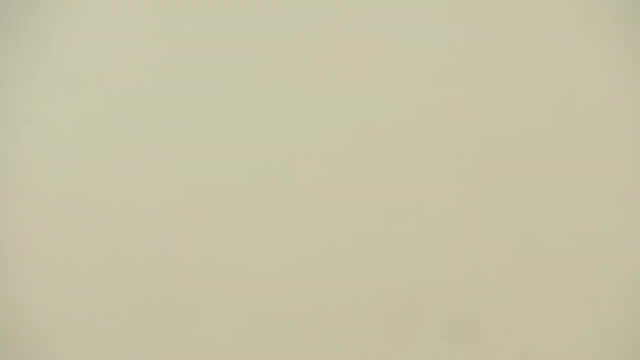 Rewrite it So it looks like that: Q double prime, watts per square meter. added to the list: Watts per square meter. So here they are: Capital E, capital G, capital J, Q double prime, all watts per square meter. 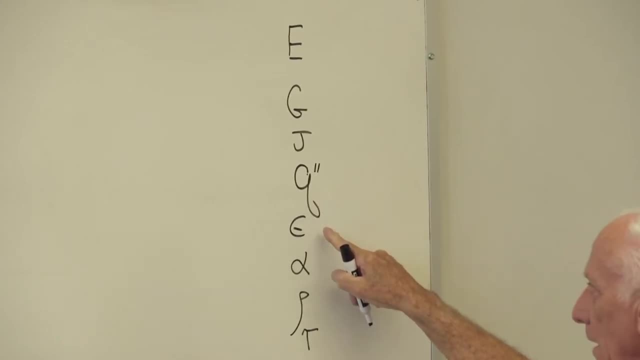 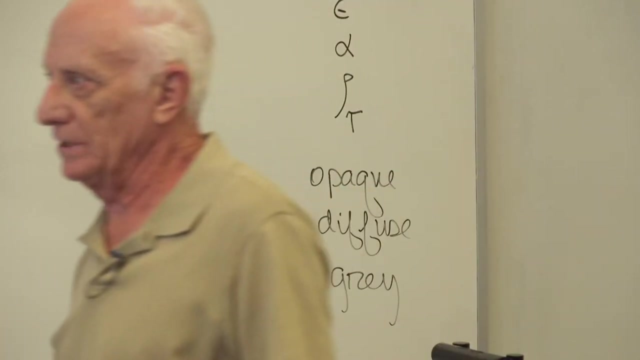 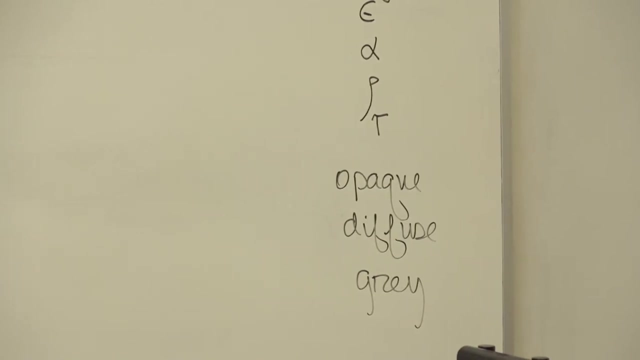 all mean different things. Epsilon, Alpha, Rho, Tau, opaque surface. Tau equals zero Black surface, Epsilon equal one. You have to understand the language of radiation. I'll put this over here. it's a sidelight. 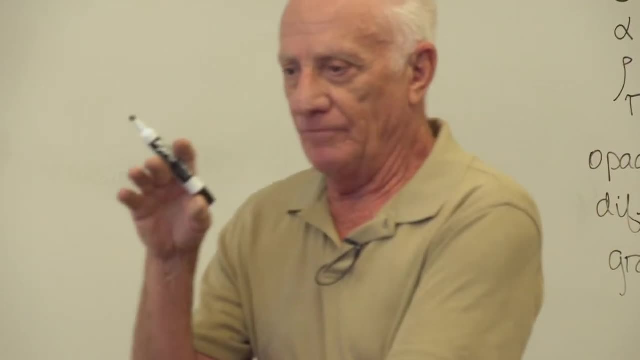 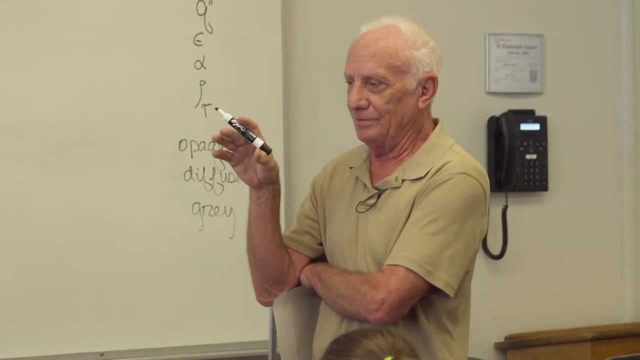 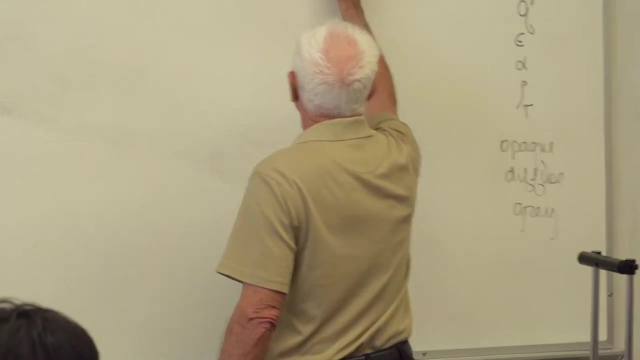 A black surface is a model of a perfect emitter and absorber. Can we get a black surface in the real world? Well, no, it's a model. We can get close to it. One way you get close to it is: you can take. 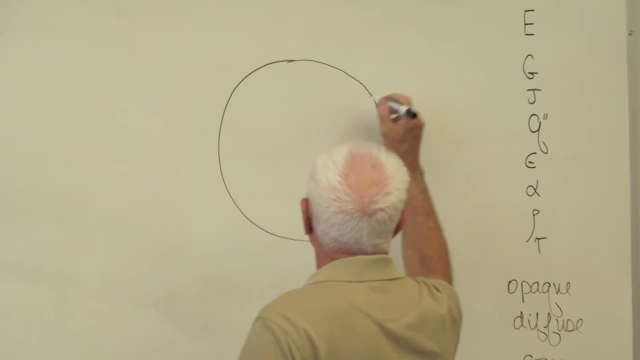 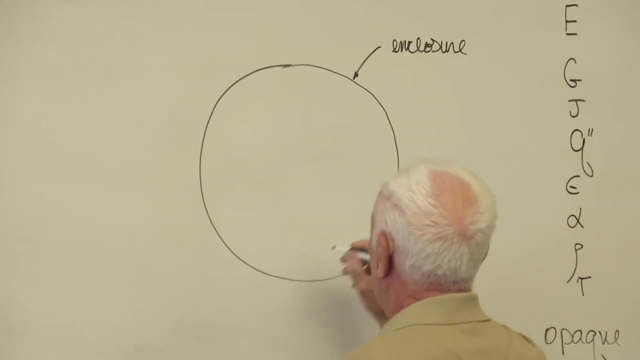 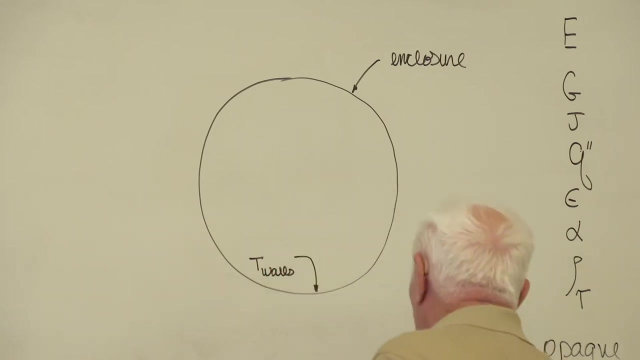 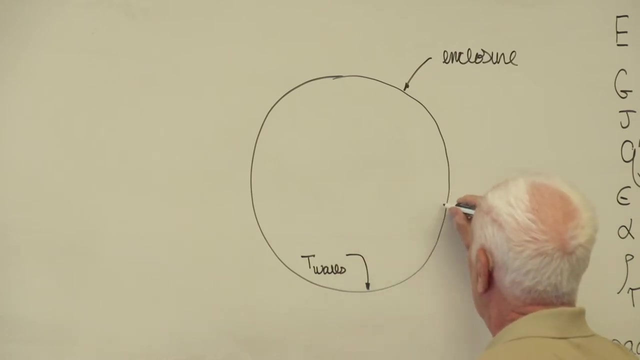 a large enclosure, for instance, and the wall temperature- T wall and the wall temperature- is the temperature of the wall. Now, when the walls will be emitting radiation, that radiation will bounce around there and be absorbed by the walls and reflected by the walls. 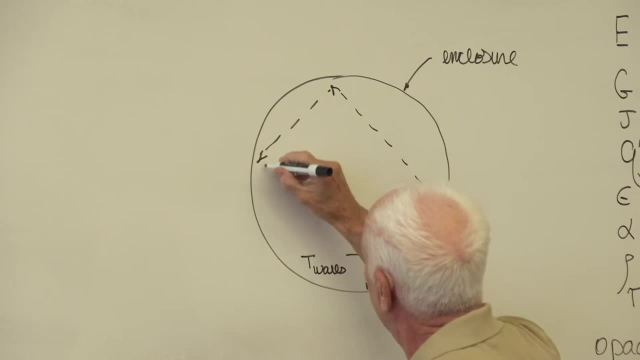 It depends on the wall properties. So it could be hit here, bounce off, hit here, bounce off, hit here. It can bounce around there from all these surfaces You can drill a small hole there. a small hole, It turns out the radiation emanating from. 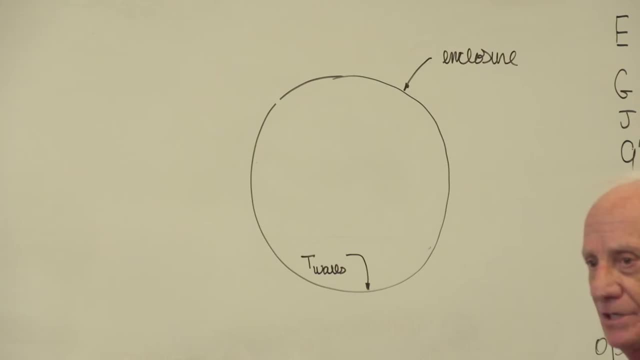 that small hole looks like black body radiation at the temperature of the walls- E b Lambda at the temperature of the walls. That's this radiation leaving the hole. That's what comes out of this hole. It has the same spectral distribution of black body radiation at the temperature of the walls. 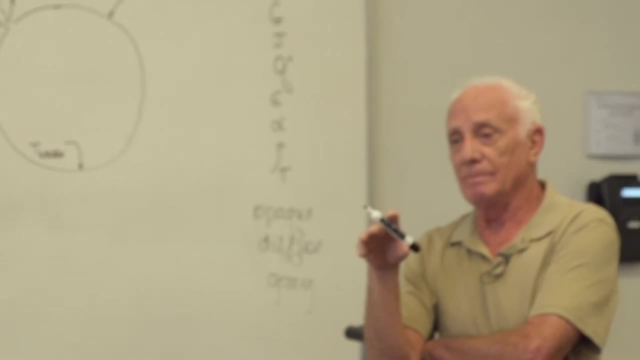 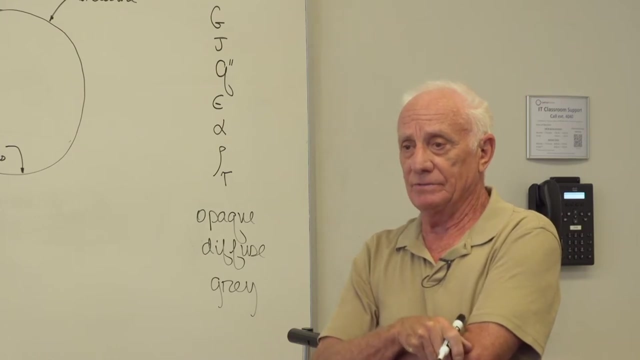 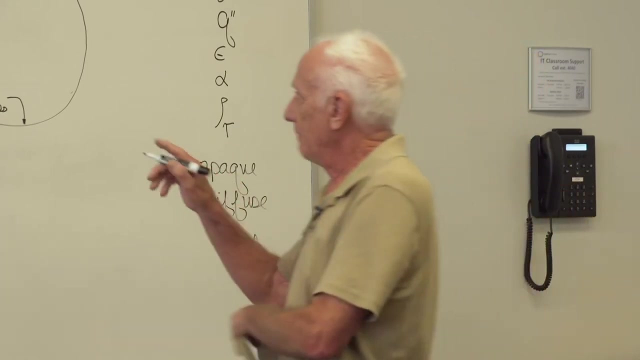 So that's how you could get close to a black body source of radiation. by doing that. People do that in the sciences. They have these in laboratories, so they do it. Now here's the other thing. This is different. The other thing is, if I put 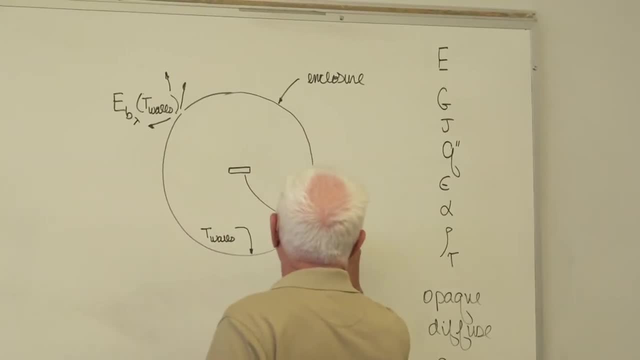 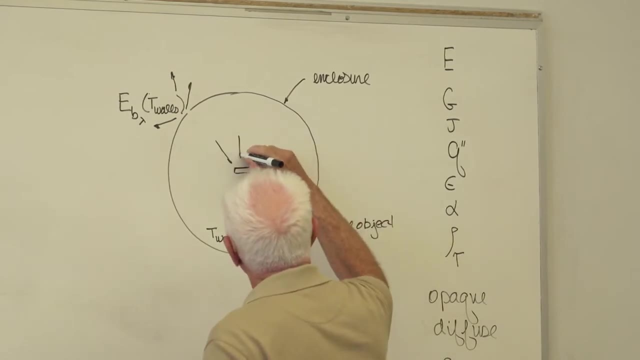 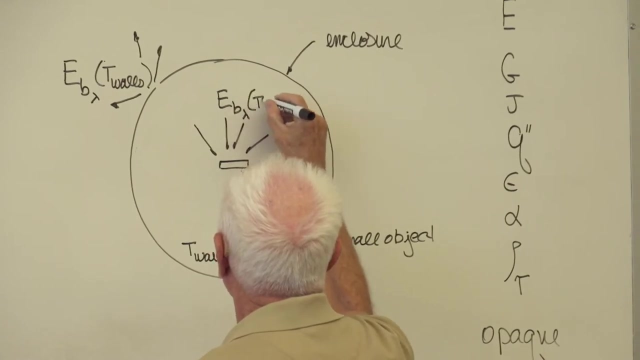 a small object in this enclosure. the radiation that comes into this from the walls appears to have come from a black body at the temperature of the walls. Go back to Chapter 1.. We said, okay, what if we have a small object in a large enclosure? 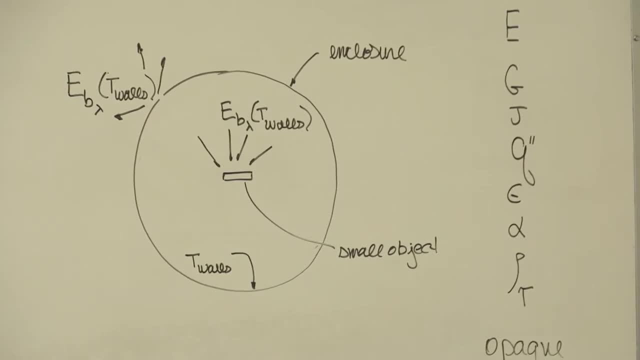 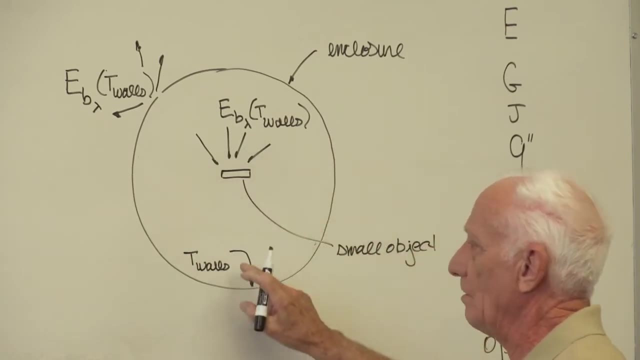 Here's the equation you use. We're going to prove that in Chapter 13.. But for right now this says: if I put a small object in this enclosure and heat the walls to a temperature T walls, the radiation approaching that small object looks like it has. 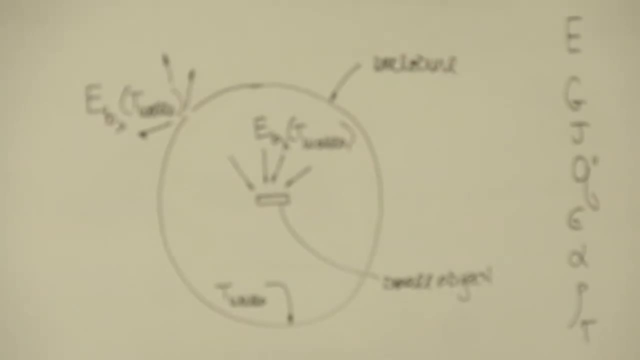 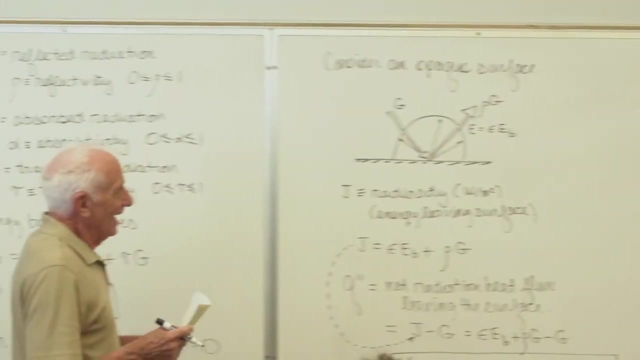 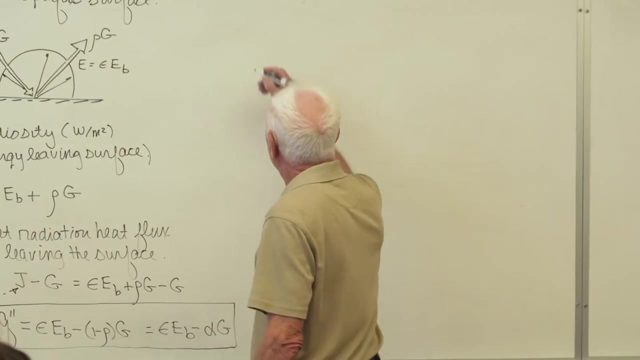 a spectral distribution of a black body at the temperature of the walls. Just so you know about that for Chapter 13.. That's the side light that can be put anywhere in Chapter 12.. There, it is right there. Let's take a look then at other properties. 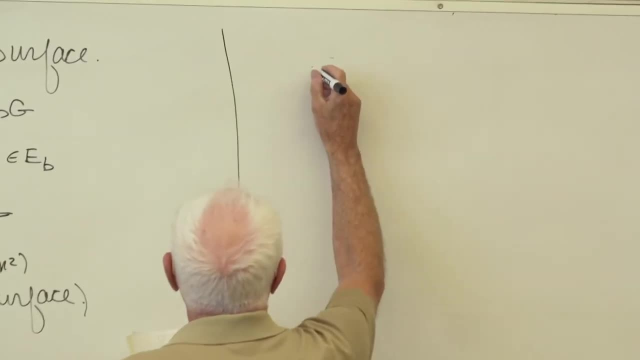 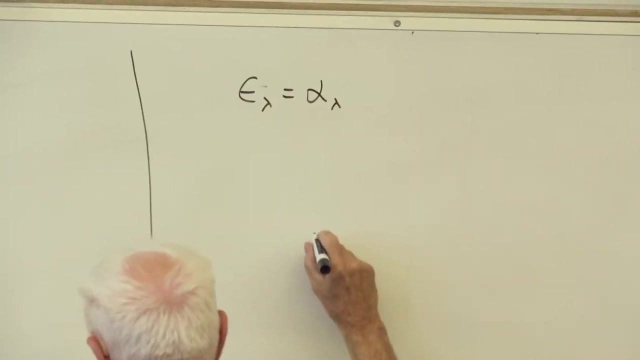 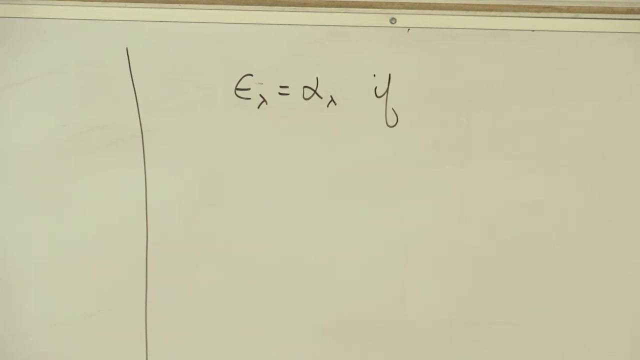 Well relating properties. Epsilon Lambda, equal Alpha Lambda. if now we can relate the two properties, The subscript Lambda means spectral. We can relate the spectral emissivity to the spectral absorptivity. So what I'm doing this morning is talking about properties. 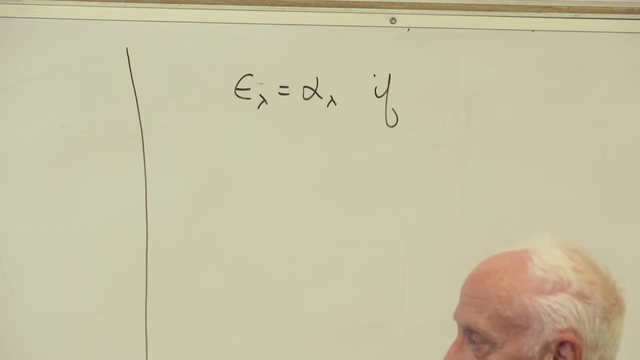 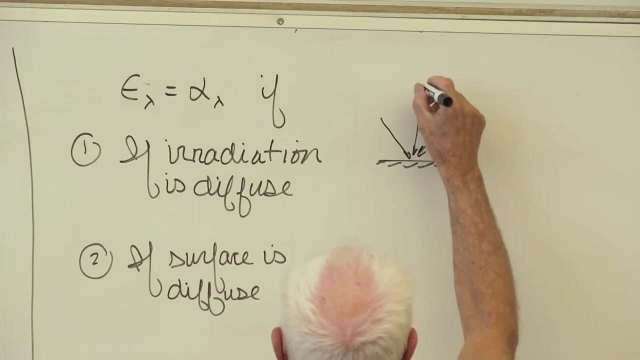 What properties? Epsilon, Alpha, Rho, Tau. This is true. two cases: Number 1, if the irradiation is diffuse. Number 2, if the surface is diffuse. Well, let's look at the first one. Number 2, if the surface is diffuse. 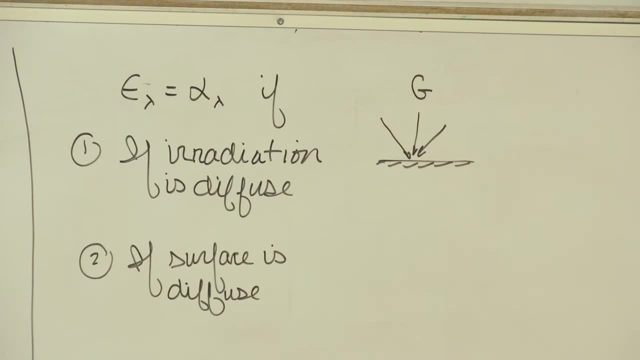 Well, let's look at the first one, Number 2, if the surface is diffuse, G coming into a surface. Diffuse means it's not a function of the angles, So every angle of radiation coming in is the same. This, this, this, this. 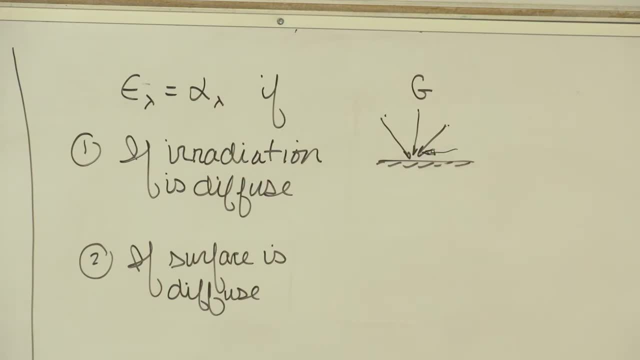 They're all the same. They're all the same, Matter of fact. you could like that If a surface is diffuse, let's say it's emitting radiation, It doesn't matter what the angle of emission is, It doesn't matter what. 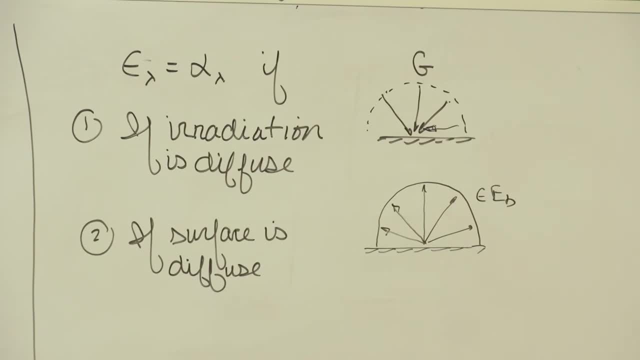 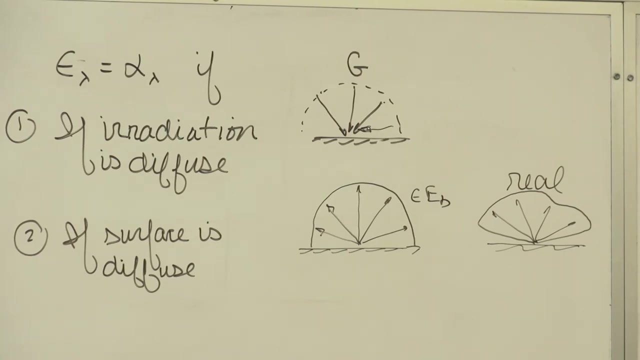 the angle of emission is: It's the same value. Now, a real surface, it might look something like this: Yeah, it's not the same, It depends on angle. But the definition of the diffuse surface is: it doesn't depend on angle. 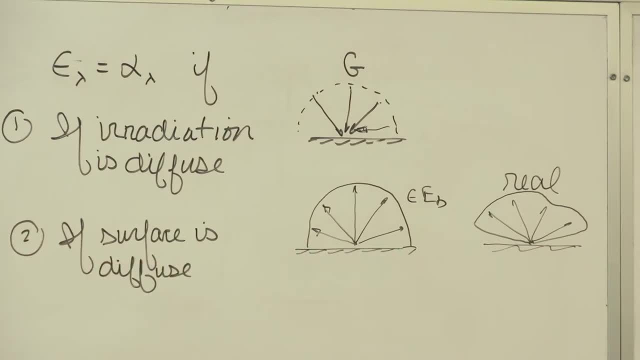 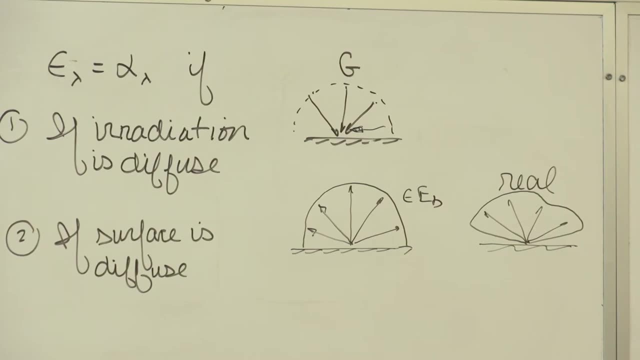 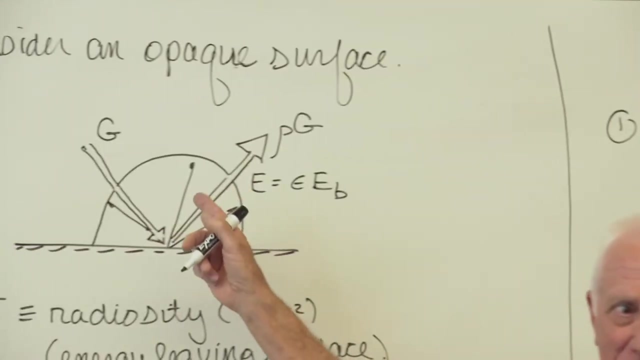 Whatever's leaving there, the reflected or the emitted, The amount of energy leaving. Okay, There it is right there. I drew that This is not diffuse. We'll get to that in a minute, But okay, that's not diffuse. 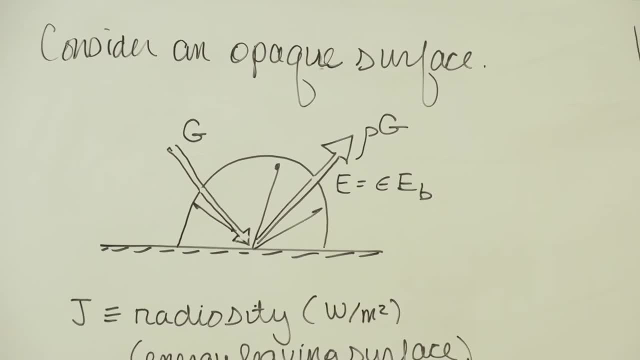 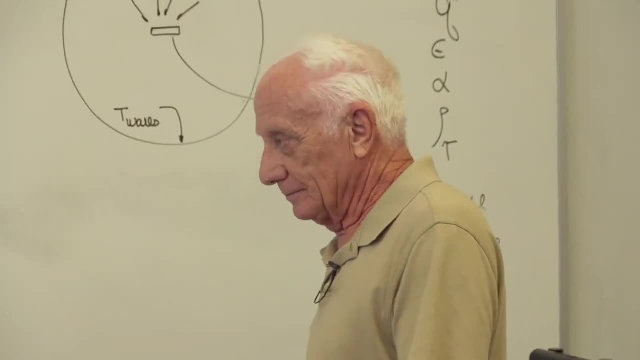 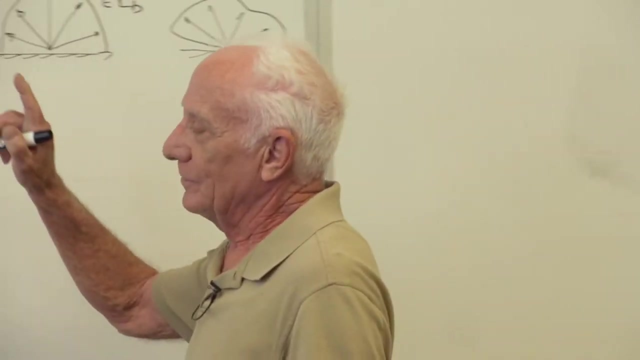 Now go ahead. I'm sorry, Say it. say it Just: the amount of energy leaving is the same at all angles. That's right. that's right, that's right. Now see, sometimes people will give you a graph of these properties. 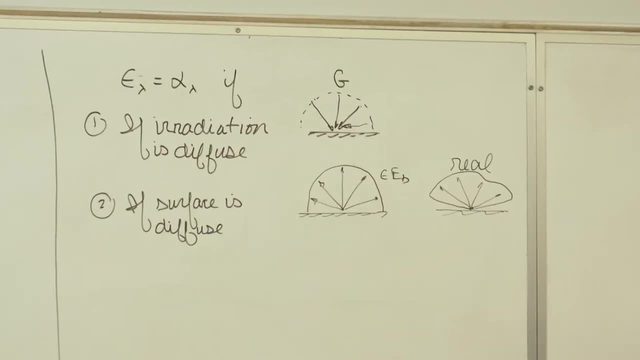 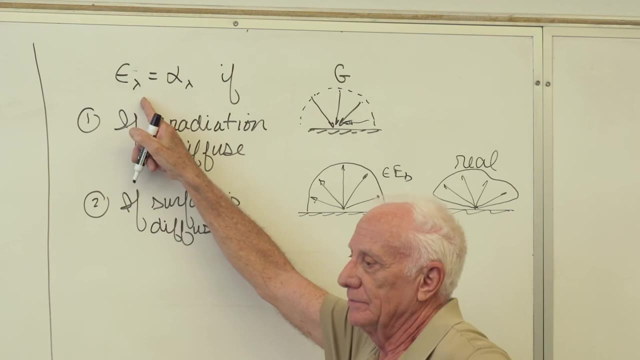 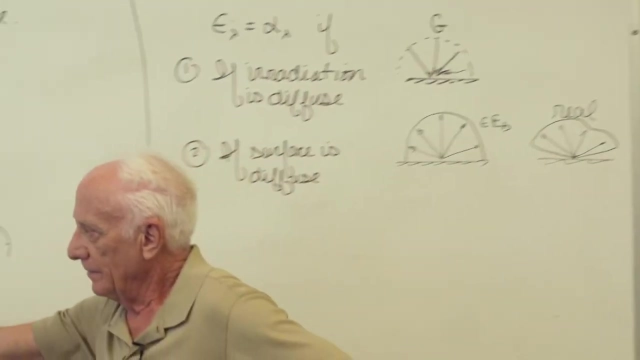 as a function of wavelength And this tells us we can equate these two guys. If we're given a graph of Epsilon Lambda versus Lambda, we can interpret that as a graph of Alpha Lambda versus Lambda. So it relates the properties. This relates the properties. 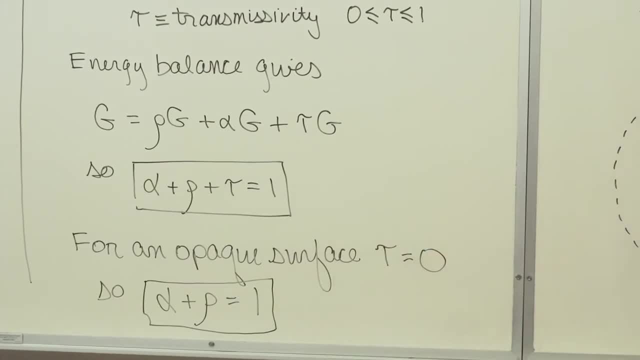 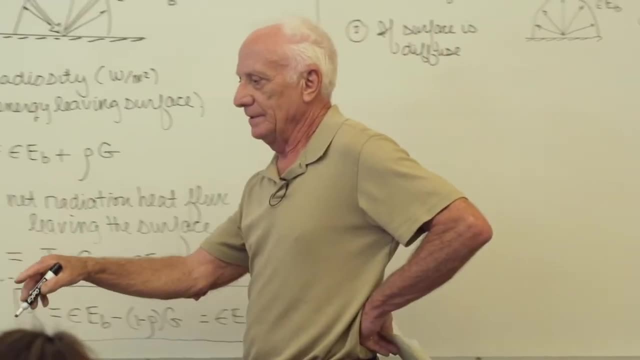 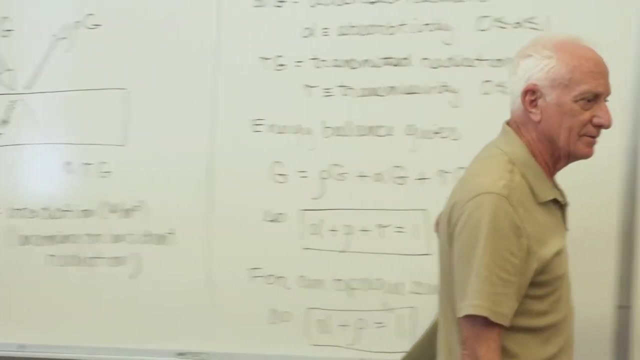 This relates the properties. If you want to find the emissivity of all kinds of surfaces, it's in the appendix: Stainless steel, copper, polished aluminum, snow sand, skin, whatever. It's all back there in the back of the book. 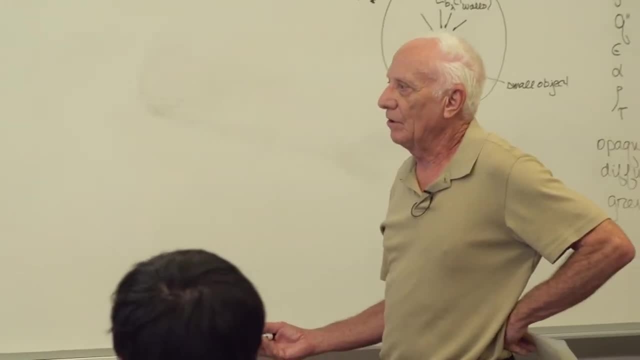 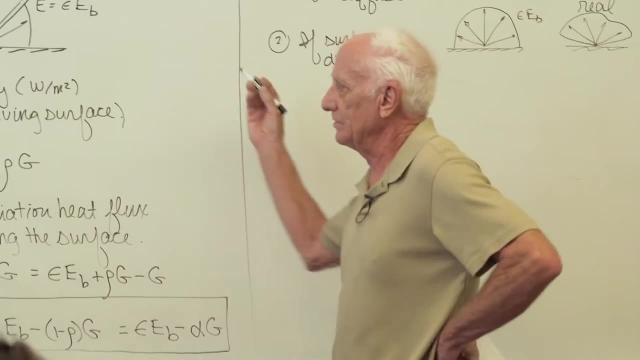 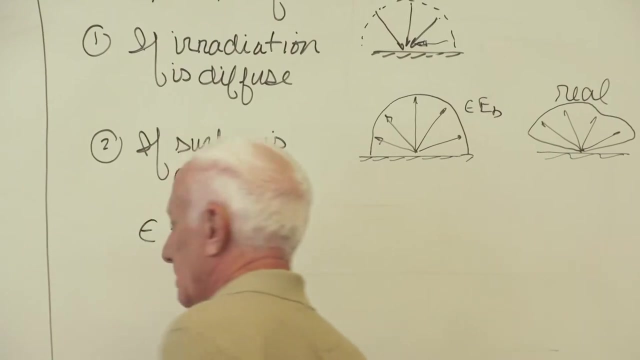 Epsilon. So that's where you can find some of the properties in the back of the book. Then maybe you can relate the properties by these equations. For instance, you can also say: Epsilon, equal, equal, Alpha, No Lambdas. now It's called: 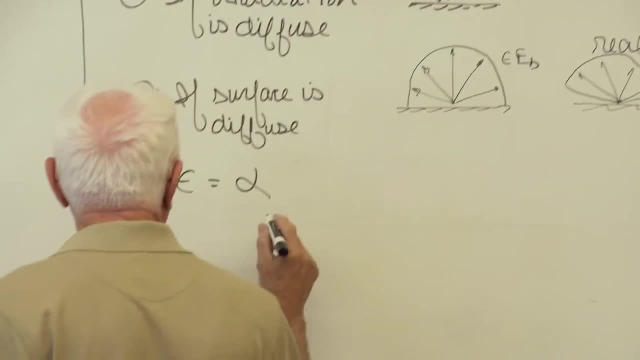 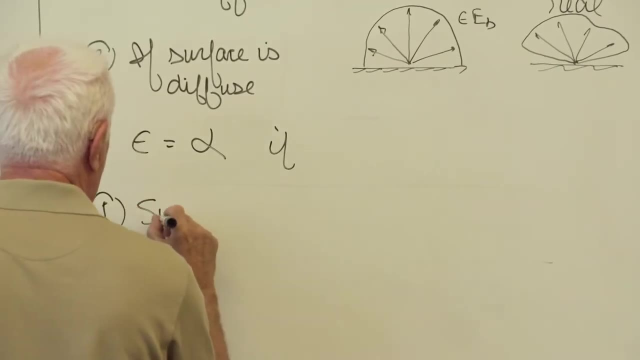 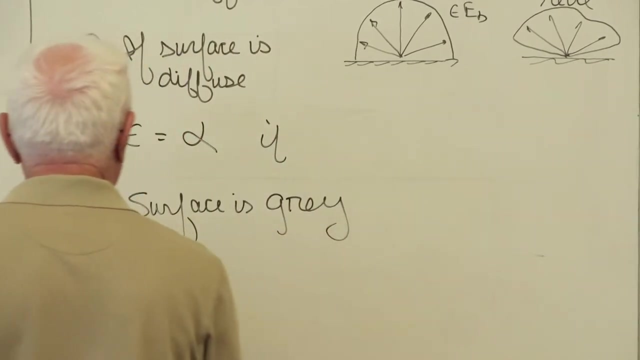 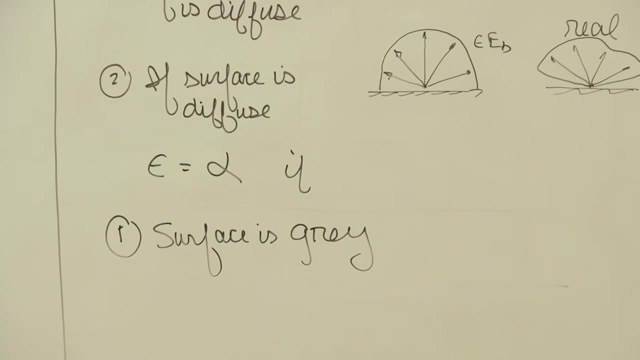 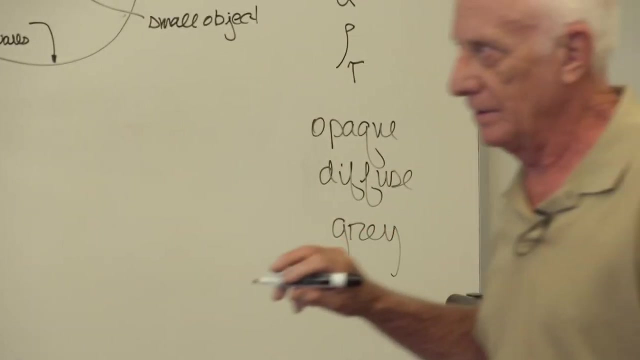 the total emissivity and the total absorptivity. If surface is gray, Add one more word to a vocabulary. A surface can be opaque, it can be diffused or it can be gray. What does gray mean? Well, if I'm given a property, 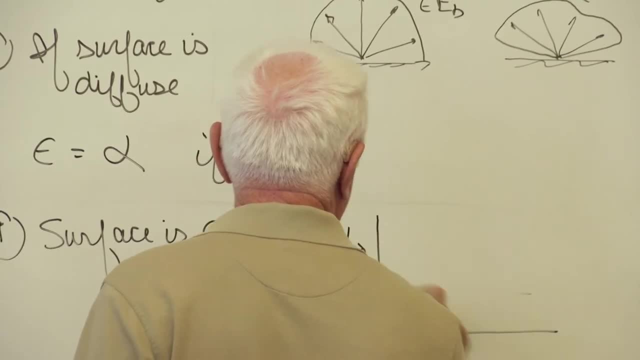 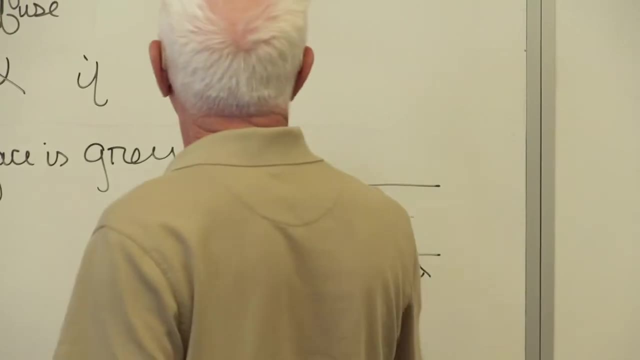 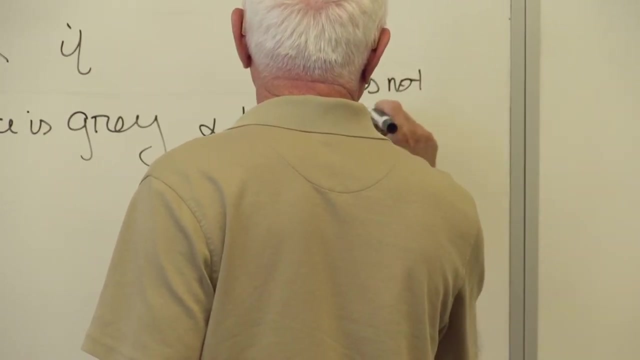 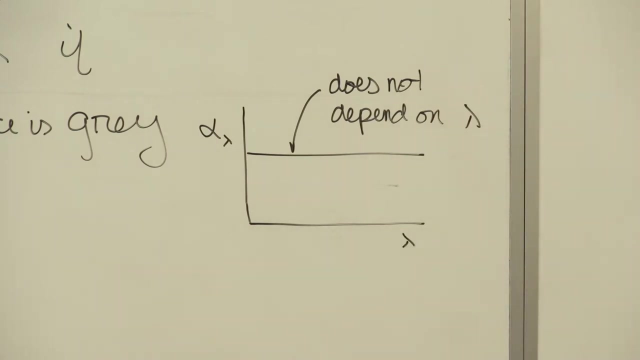 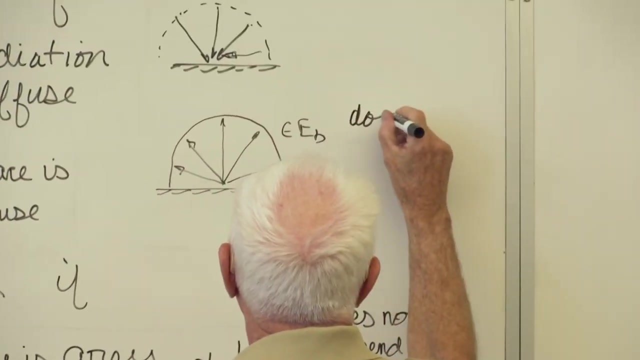 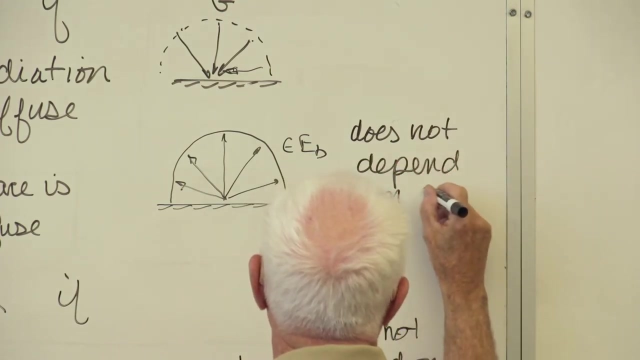 let's just say Alpha, Lambda versus Lambda, and it's constant. then that's a gray surface. Gray surface does not depend on Lambda. diffused surface does not depend on Alpha, on Beta, pardon me. So you look at the problem. 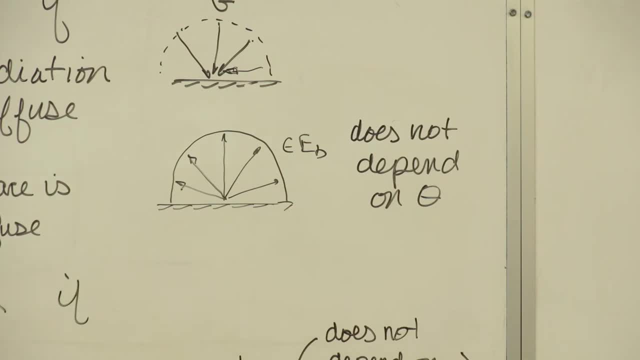 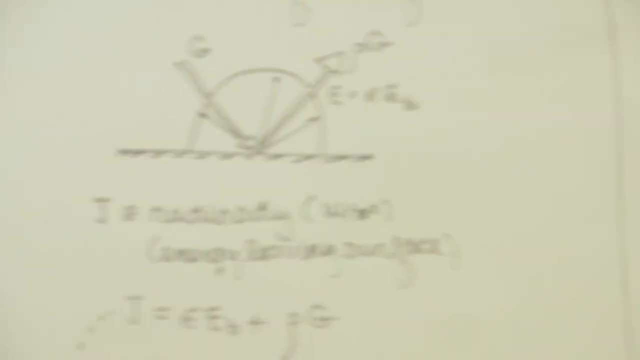 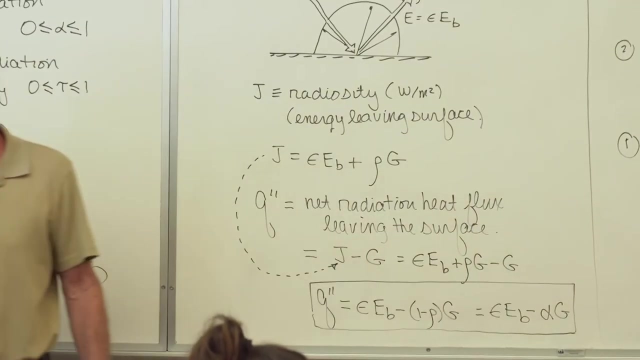 make sure you understand what you're being given In Chapter 13,. pretty much all the surfaces will be diffused and gray, Probably opaque, diffusing gray. But just so you know. those are the differences of the words. There's also a number two for this. 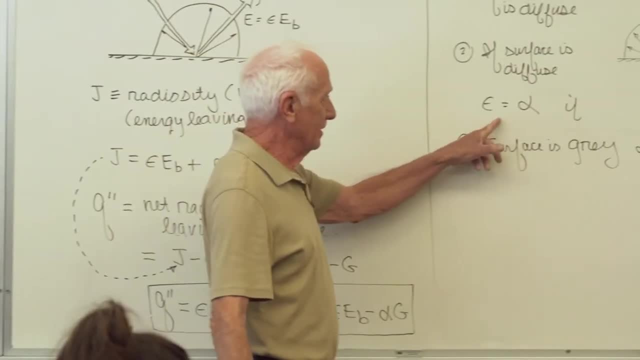 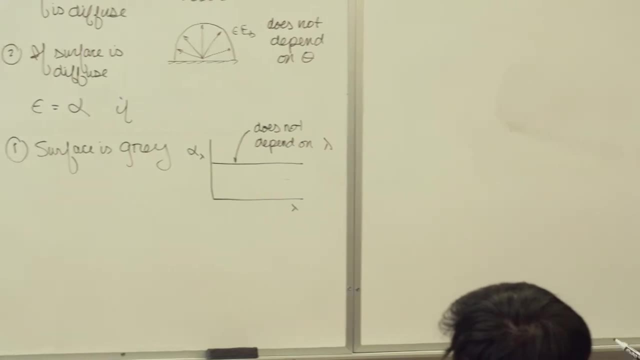 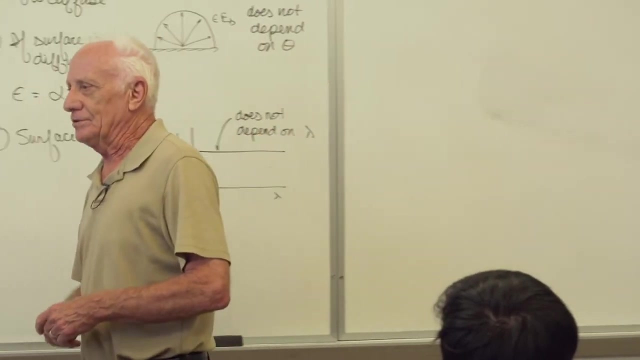 but it's not important for what we're doing, so I'm not going to cloud the issue. There's another one here, but don't worry about that. It rarely happens, Okay, Diffuse. the word diffuse means to spread out. 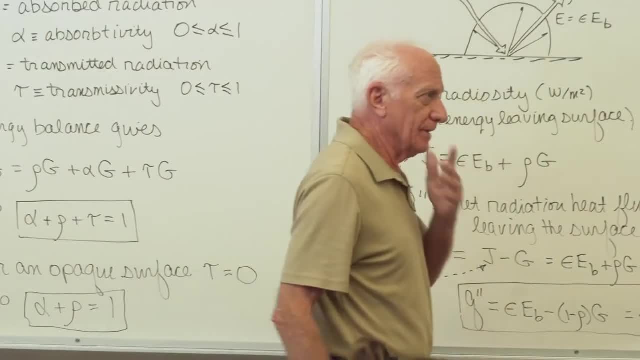 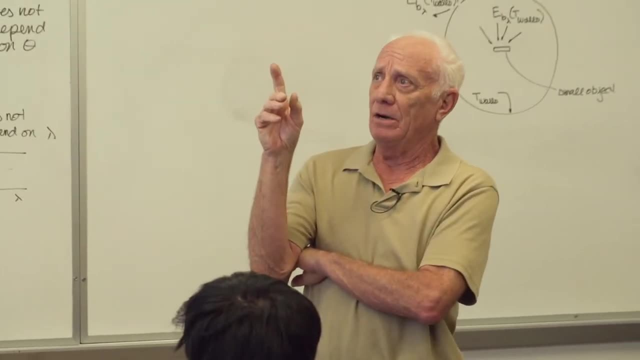 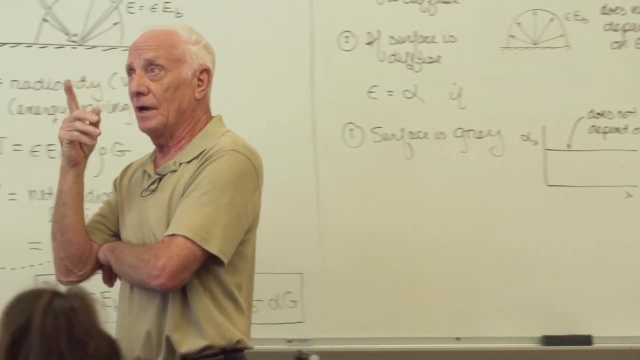 It means spread out. So if I look at how this room is lit, there's fluorescent tubes, but they're not bare, They're covered by some plastic. The purpose of the plastic is to spread the light out, so I don't get spots. 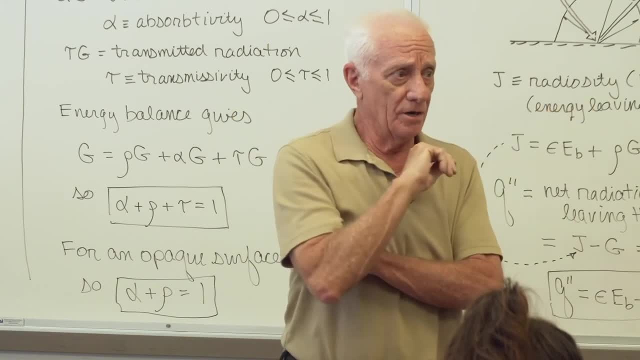 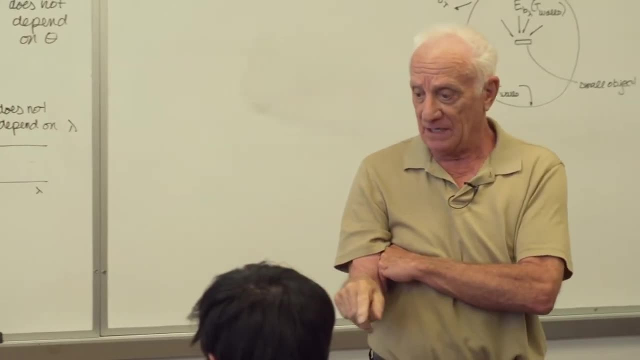 where it's dark in the corners over there or it's really bright in front here. If I put a light intensity meter on the desktop, I want that intensity to be the same up here in this front desk as that corner desk. So those guys' purpose in life is to 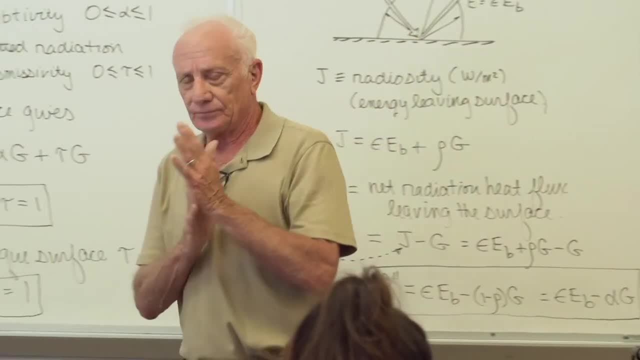 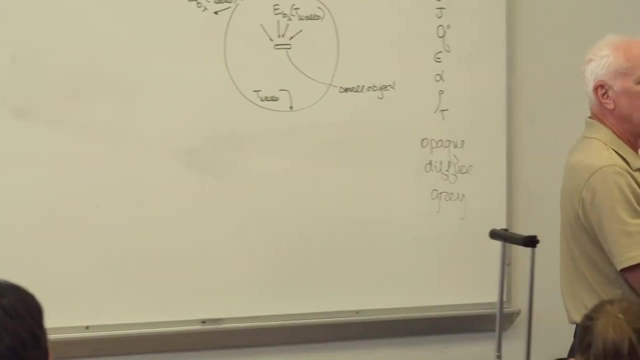 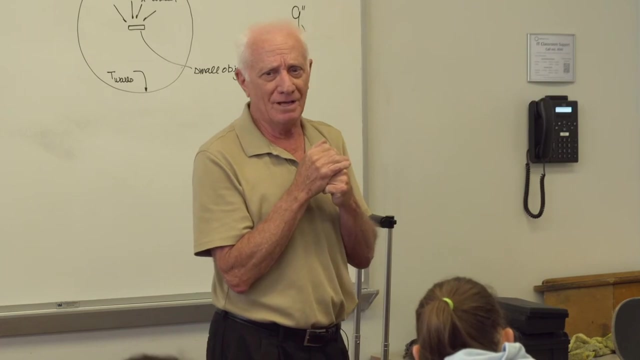 spread the light out evenly in this room. I hear the HVAC system on right now. I can hear it's working, There's air coming out of there, But it's just not a screen up there. No, that wouldn't be good. 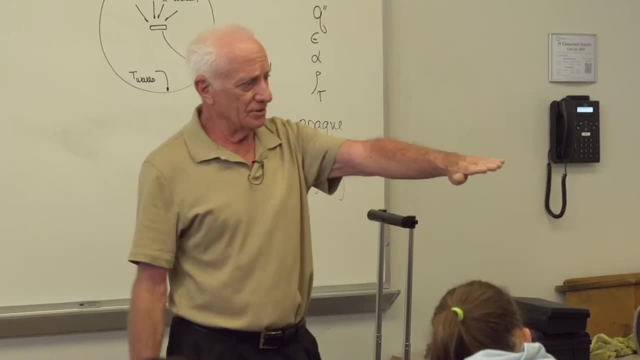 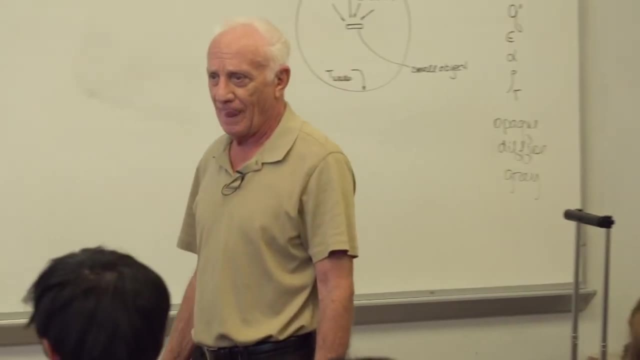 No, There's veins. Some veins are horizontal and they tilt like this. Some veins are vertical and they tilt like this, like inside your car, if you're air conditioning, heater, your air vents. What's their purpose in life? To spread the air out. 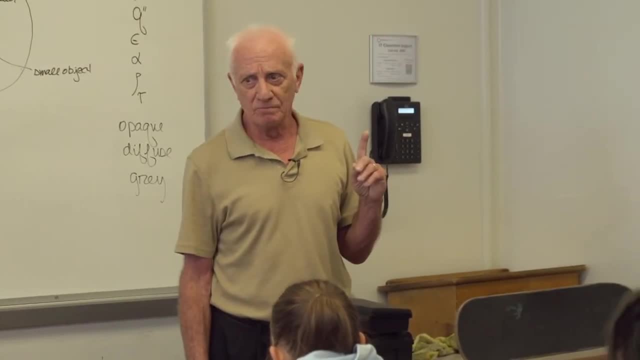 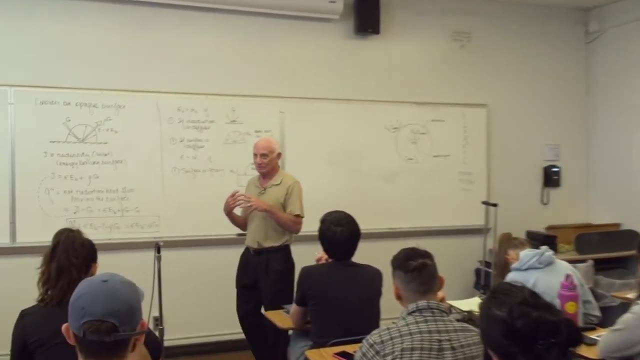 It's an air diffuser so that nobody's hair is moving. right now I don't see anybody's hair moving, but I'll guarantee you. there are some classrooms in the building which have been modified and split from one big room to a small room. 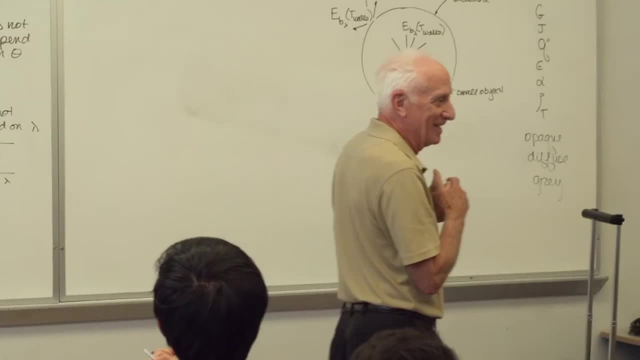 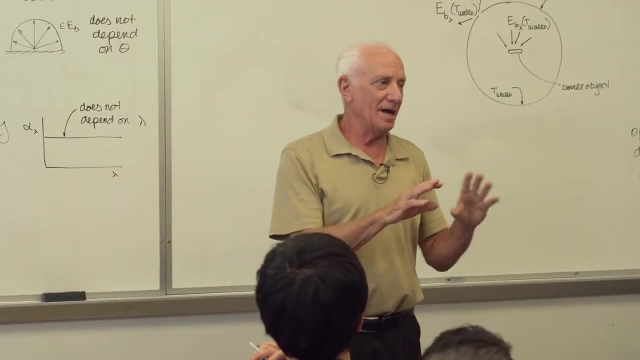 and by doing that they messed up the HVAC system. I've seen people's hair in the front row blowing, So that's not good. No, The purpose of that guy there is to make sure everybody gets a nice gentle breeze. You don't even know it's on. 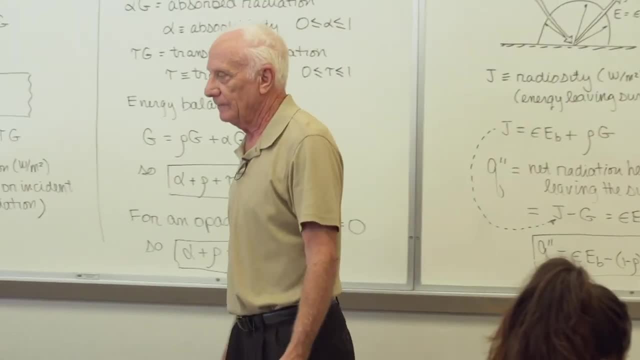 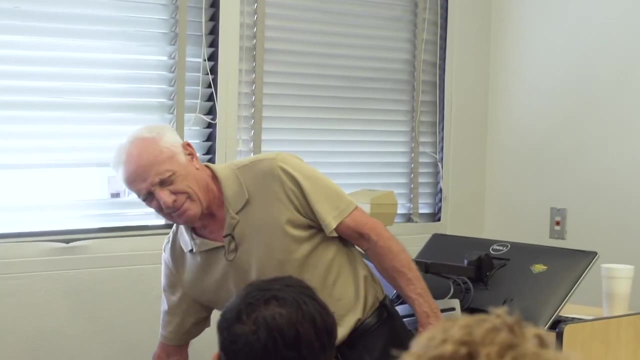 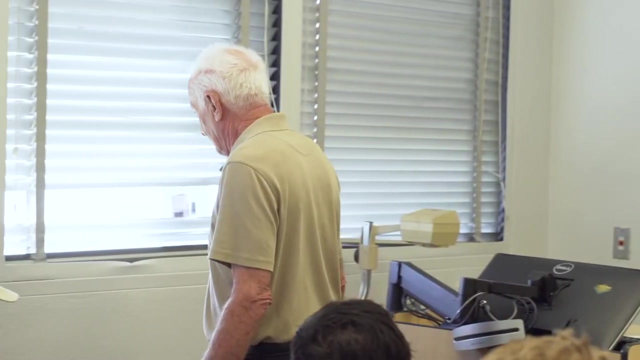 but it is on and it's working fine Here. this building was built- gosh, I don't know- sometime- I think it must be the early 60s or something, I don't know. But they have glass windows. Nice, I can see out. 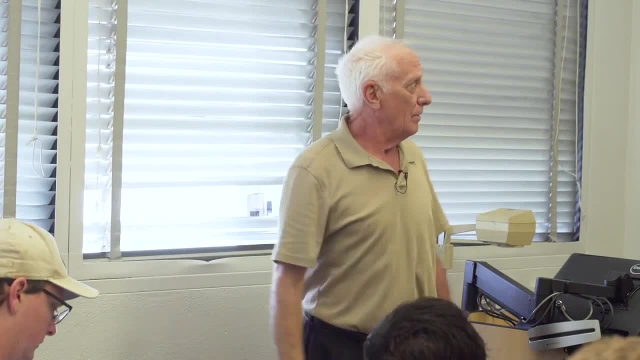 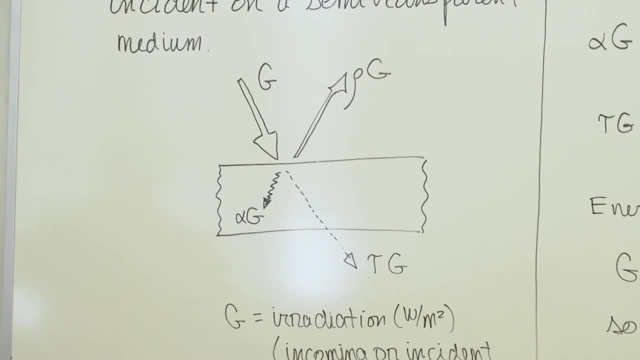 I see building 98 there, That glass window right there. Some of the sunlight G? G is the sunlight. Some of the sunlight is reflected off the glass. Yeah, a little bit. Sometimes you'll see that near sunset or sunrise. 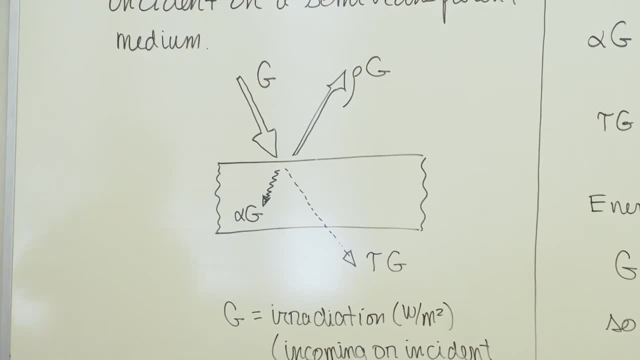 You'll see some reflection of the glass. Some of that goes straight through to my eyes. Yeah, sure does. Yeah, My visible spectrum 0.4 to 0.7 microns. Some of that solar energy is absorbed by the glass because the glass contains iron. 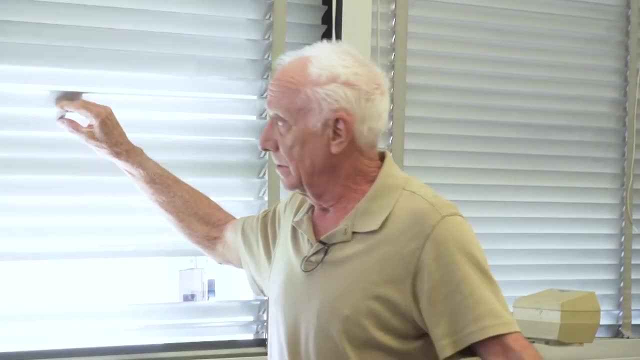 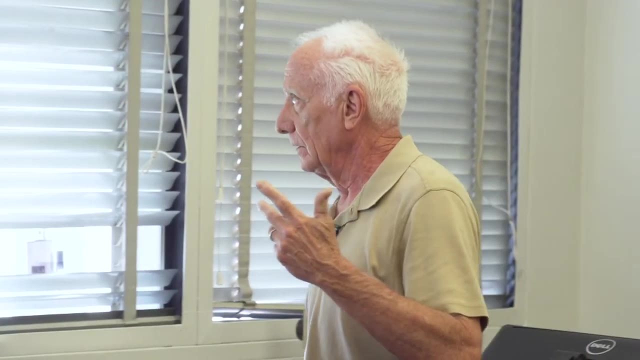 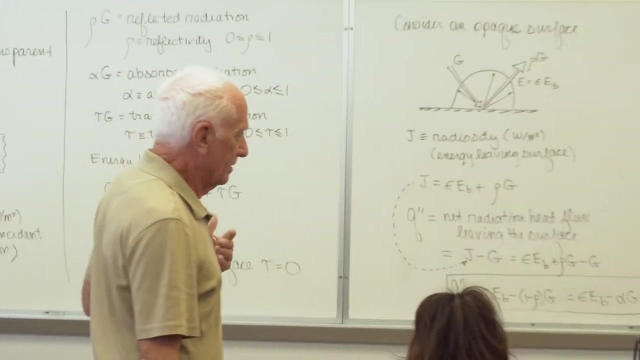 Iron and iron absorb. So there is reflection absorption and transmission in glass. Good glass transmits about 93 percent. You can buy really really good glass for solar collectors that transmits more, but of course it costs more. They take the iron out. 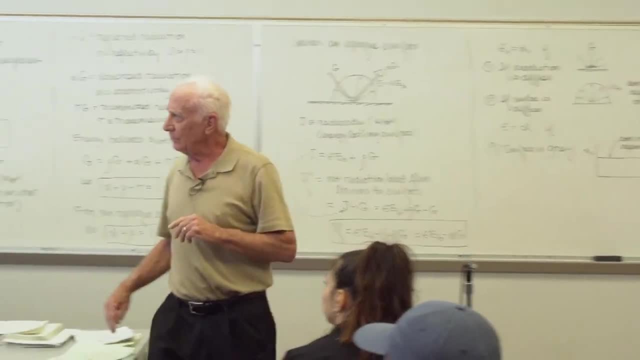 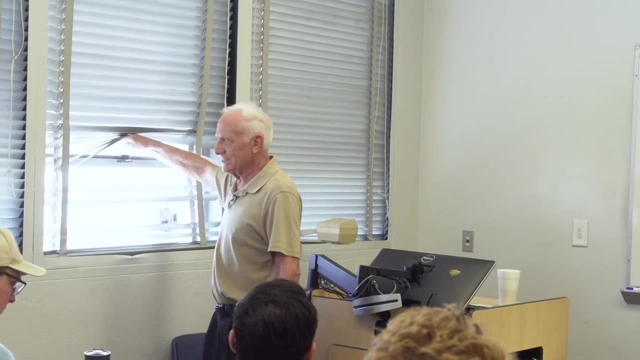 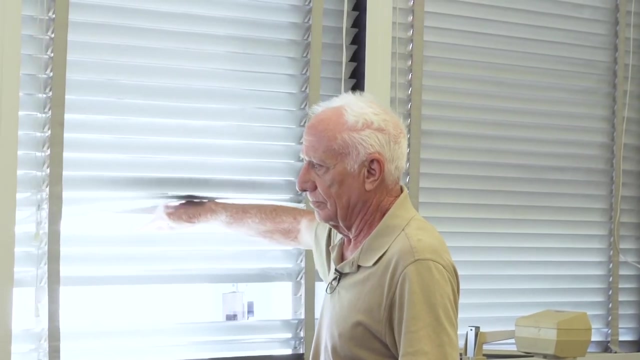 Yeah. Then you say: well, what did they do here? Why isn't this all glass like that? I'll take your fingernail, rub it on here Now rub it on here, It's like sandpaper. Yeah, it's dimple glass. 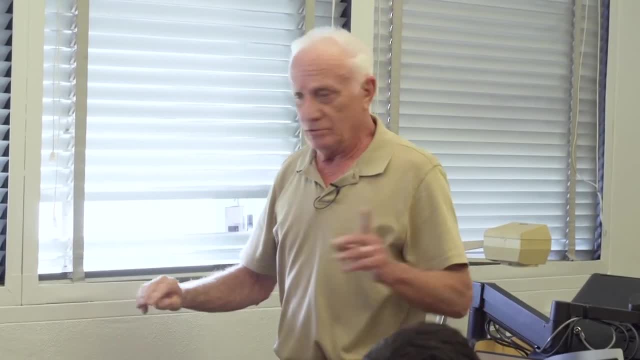 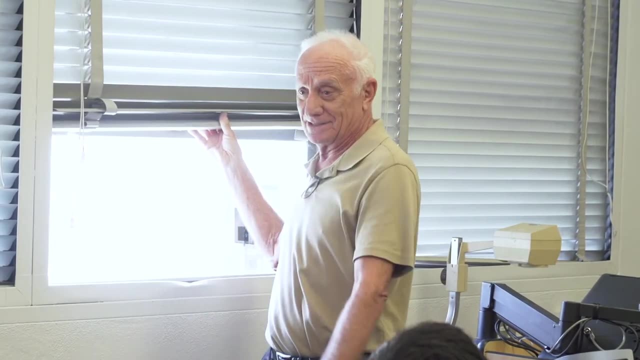 What's its purpose in life. If you want more light in the room, you can raise this up here Now. if this was plain glass, you'd be blinded this time of day. You guys in the front here have a bright light on your face. 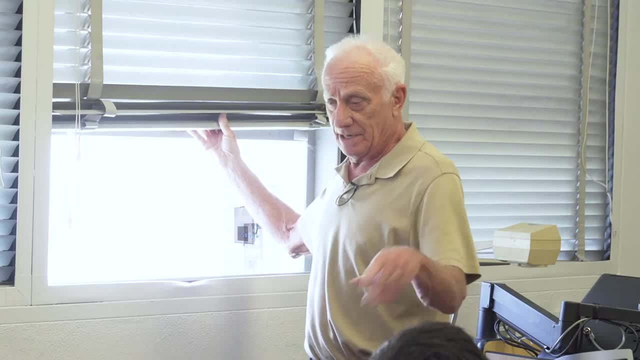 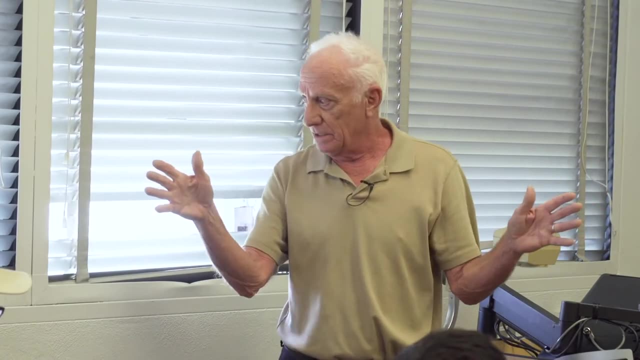 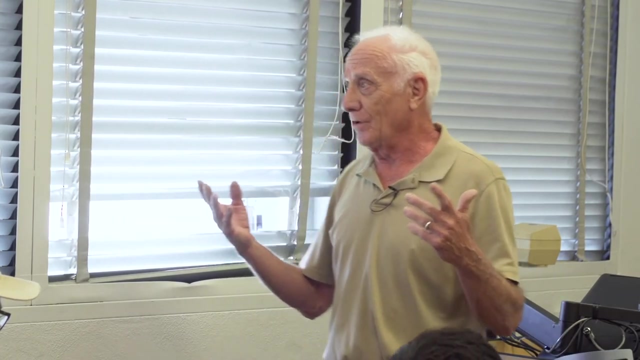 but you don't. right now It's a muted light on your face. So what's this guy's purpose in life? Purpose in life is to spread the light out evenly. It's a diffusing type glass- Very neat idea, So you can have natural light in this room. 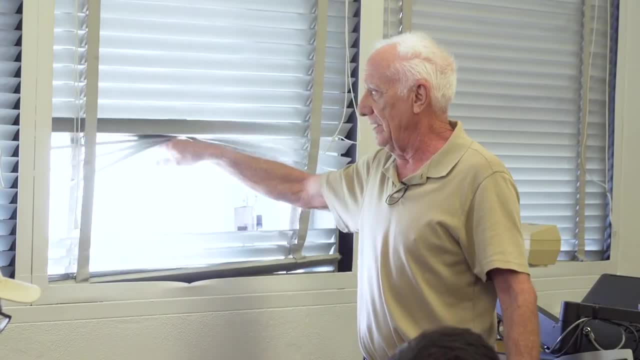 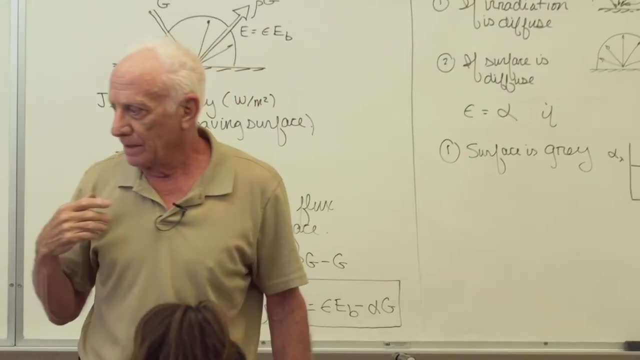 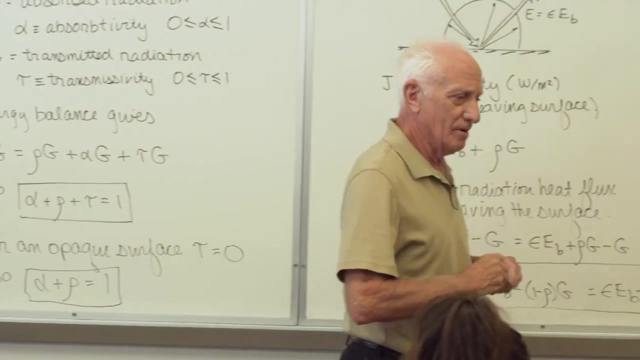 pull the blinds up to here, close these blinds and you'll still get nice light, but it's a diffused light, So it's not objectionable to anybody sitting over there by the windows. Now you say Jesus, I wouldn't polish my car. 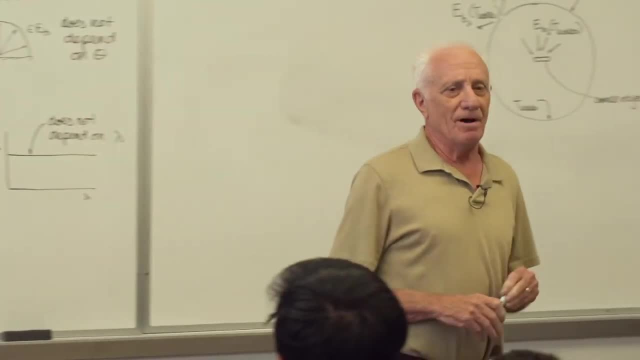 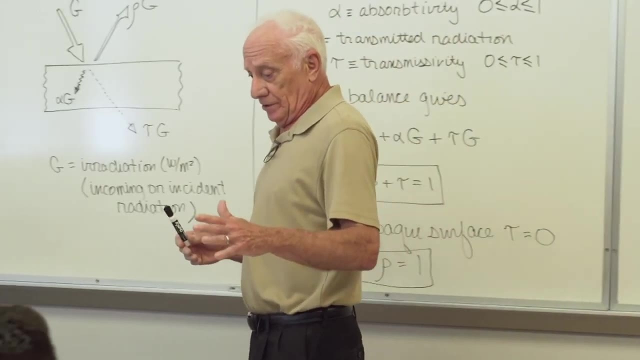 maybe not supposed to rain someday. But let the next Monday say: I'm going to polish my car next week. Okay, good. So you polish your car, you do a really good job, you're proud of it. You look at the hood and you say: 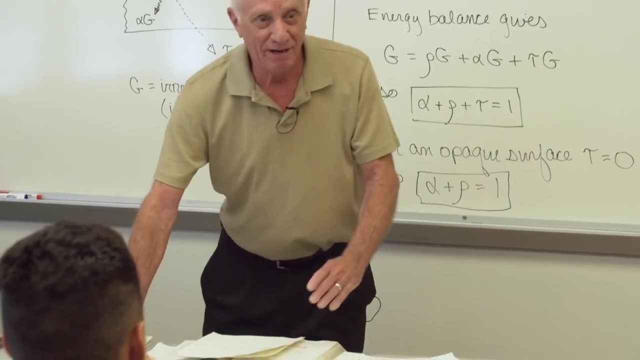 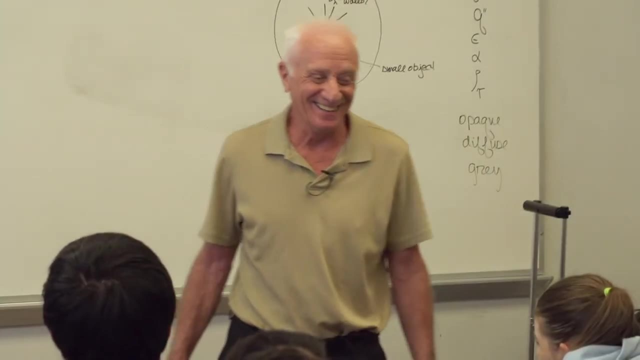 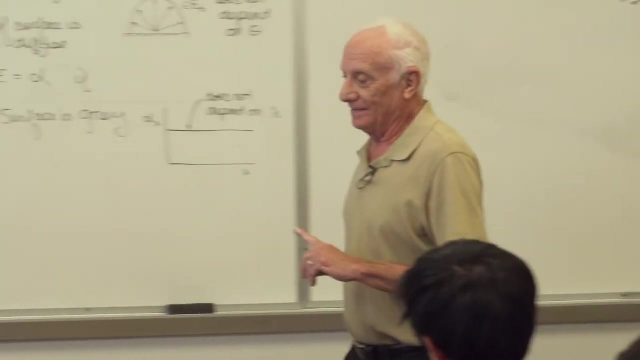 I did a great job. Look at my face. I can see my face. Yeah, you did a good job. Okay, congratulations. Now, yeah, but that's not diffuse. Now the next week along comes a Santa and a wind and it blows. 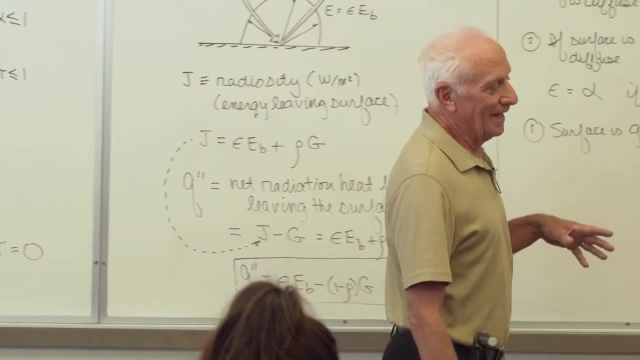 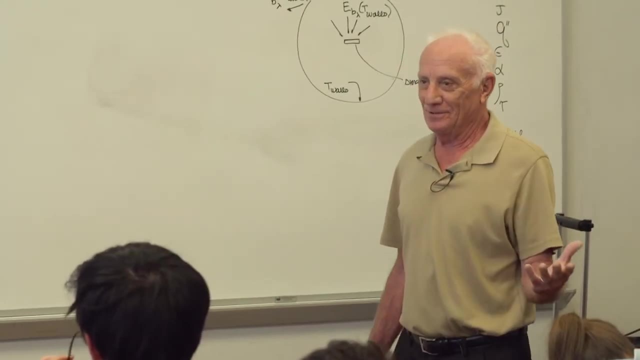 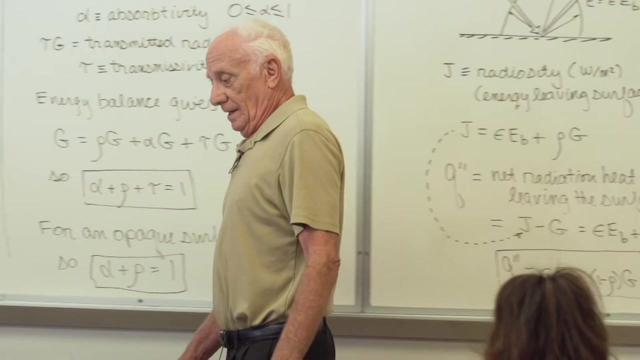 some dust and the dust gets on your car And then two days later in comes a morning fog. The water droplets go on the hood, They attach to the Santa Ana dust particles. You go out there and say: let me see my face again. 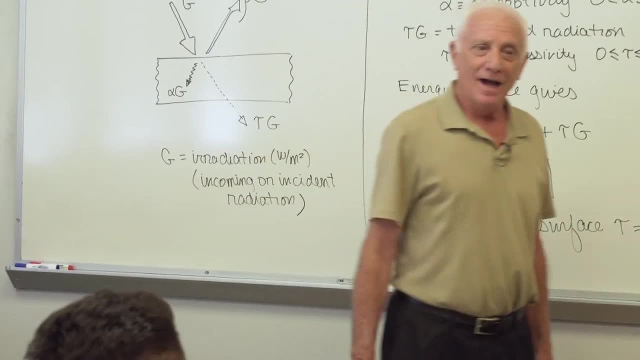 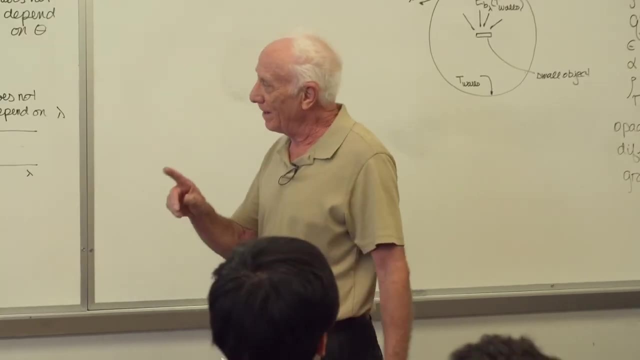 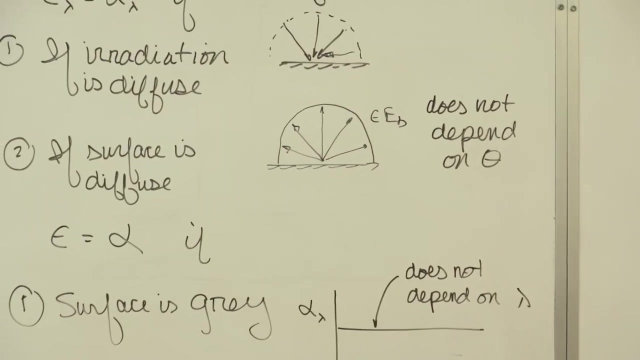 this morning. where did I go? How come I can't see my face? What happened? Well, when you polished it, when that light beam comes in from the Sun. now, when you polished it, let's do the polished one. When you polished it, it's over there. When, 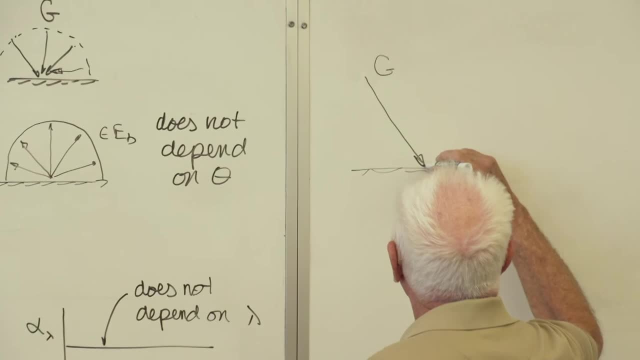 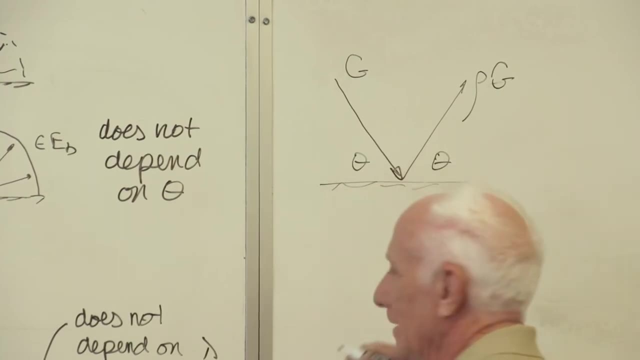 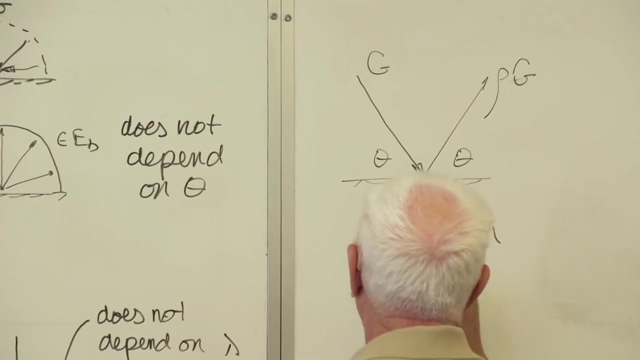 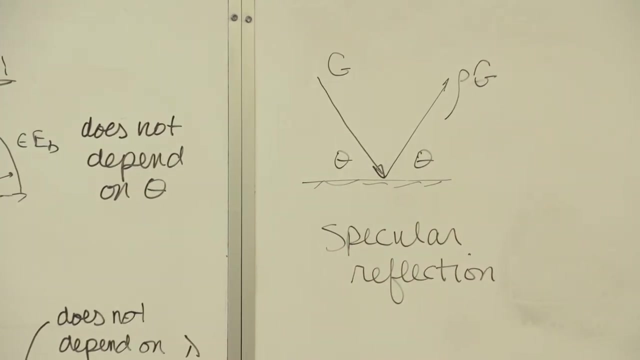 The light beam comes in from the sun: G. the reflected rho: G and the angle of incidence: theta equal the angle of reflection, theta specular reflection. You did a good job polishing your car. Everything is good. I can see my face. 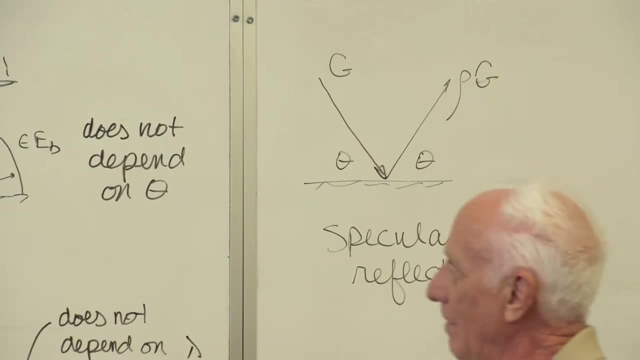 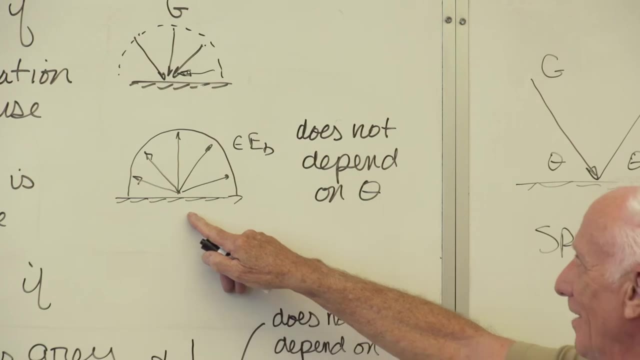 But along comes the Santa Ana and then the morning fog. All of a sudden, this is what happens. It looks like that window over there. That's what the dust particles do to it: It causes a diffuse reflection. So that's what the word. 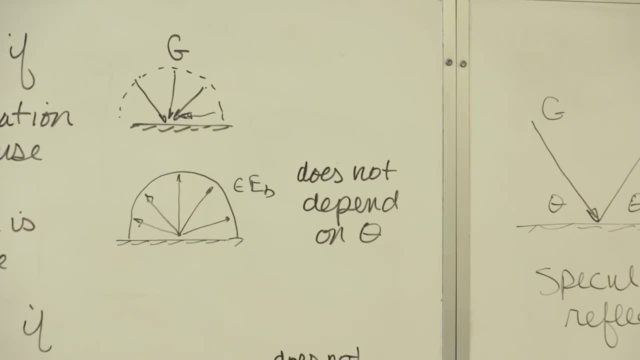 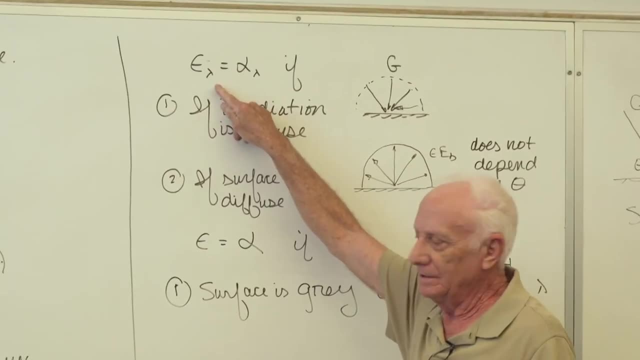 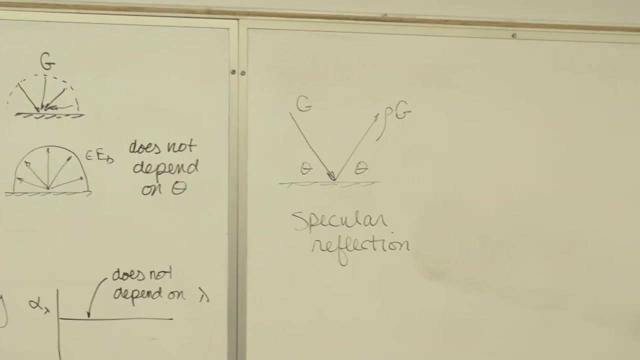 diffuse means, in common terms, Again, the language. What does this Lambda mean? Spectral, What is this sphere? Specular? Is it close? It sounds close. Is it the same thing? Of course not, But the language in Chapter 12 is very important. 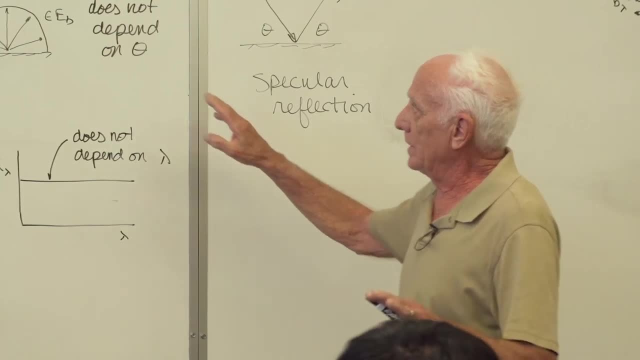 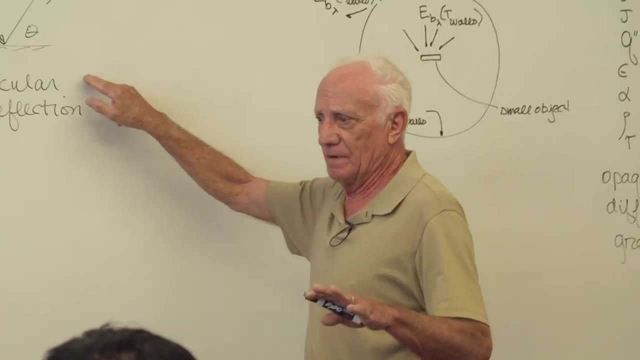 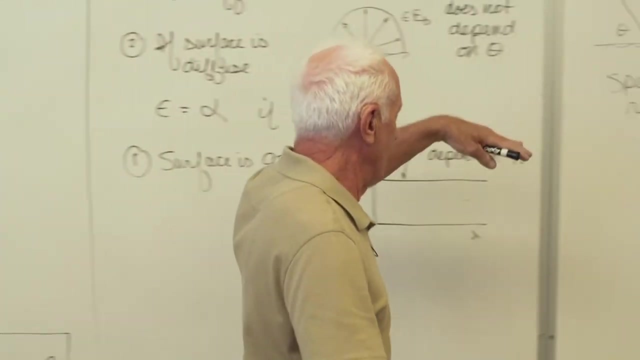 In this book we're only going to look at diffuse surfaces or diffuse irradiation, That's it. We're not going to tackle this guy. This guy is much more complex and advanced, So we're not going to tackle that. But just so you know. there's two reflections. 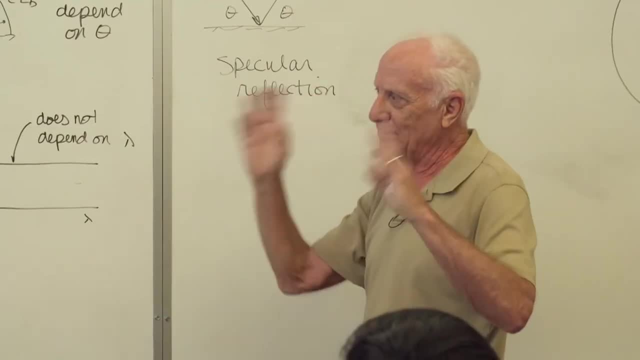 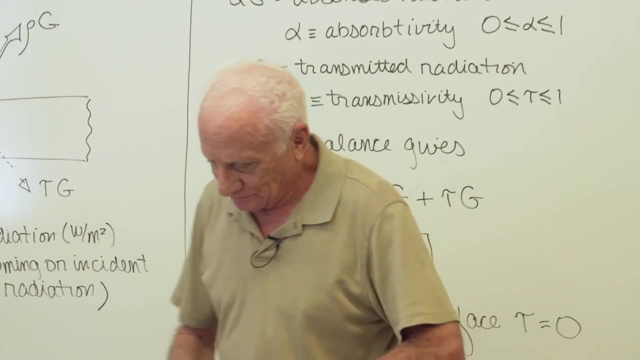 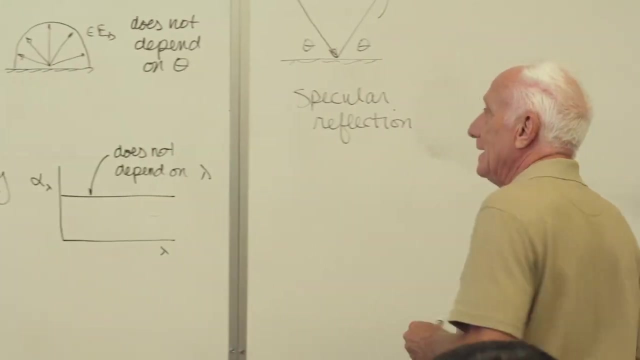 Most things in the real world are somewhere between these two, But in this book we're going to look at, let's say, diffuse irradiation or a diffuse surface. Okay Now, Spectral means, at that wavelength, Spectral Spectral. Yes, it does Exactly. 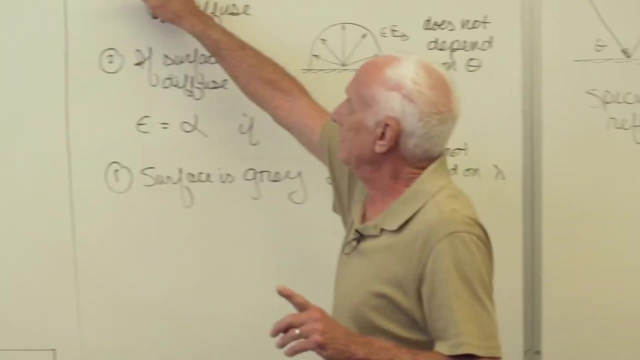 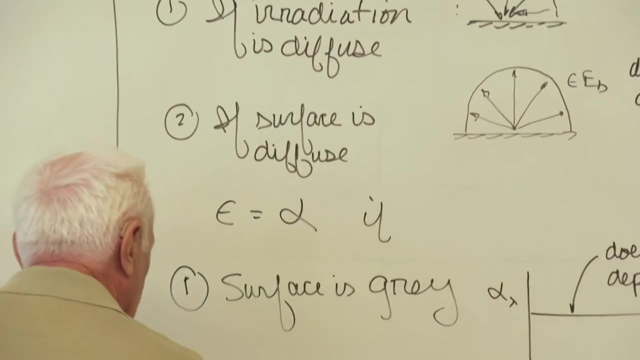 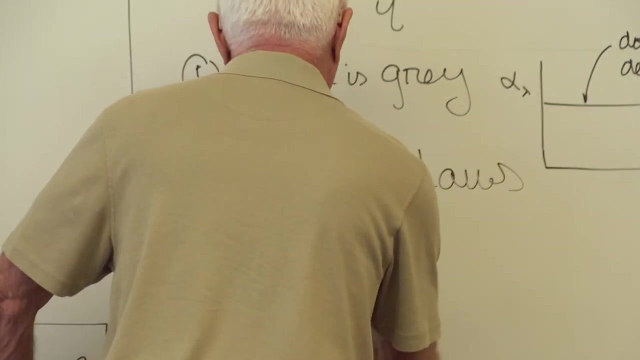 And here's what it means. It means it's a function of wavelength. This is emissivity as a function of wavelength or at one wavelength. Take your choice. These laws, by the way, are Kirchhoff's laws. Okay, Now let's mix it a little bit here. 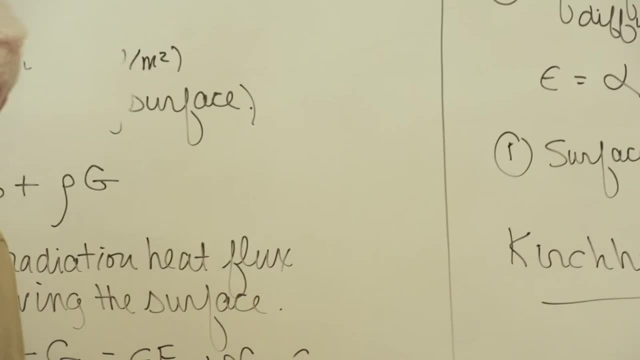 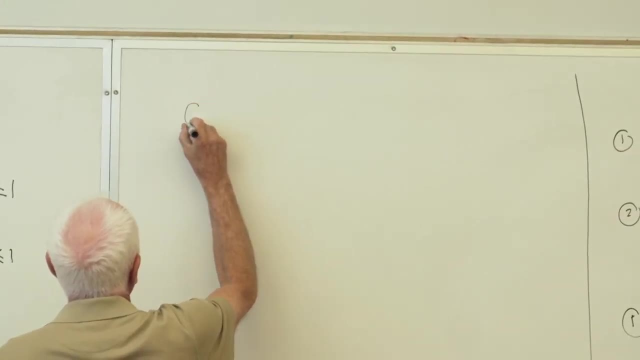 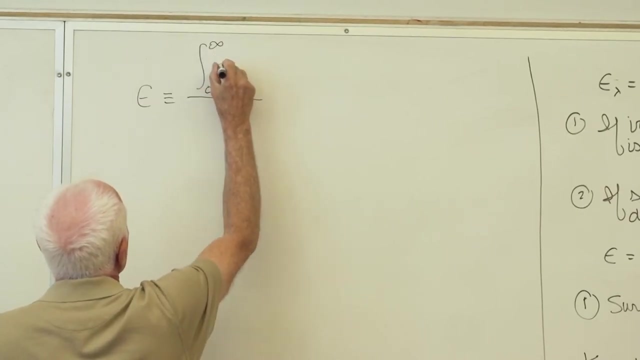 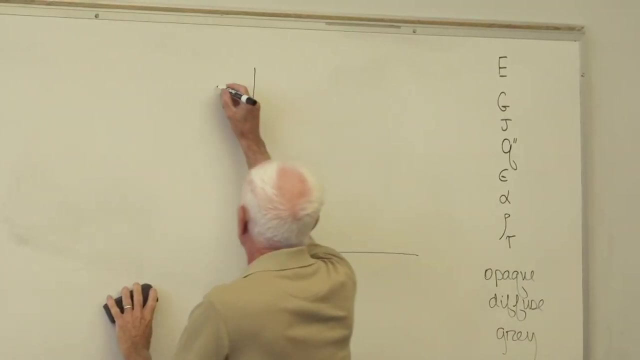 Now we're going to take a look now at how we get these properties- Epsilon, Epsilon- defined like this. Let me draw you a picture over here. Let me draw you a picture over here. Okay, Okay, Okay, Okay. 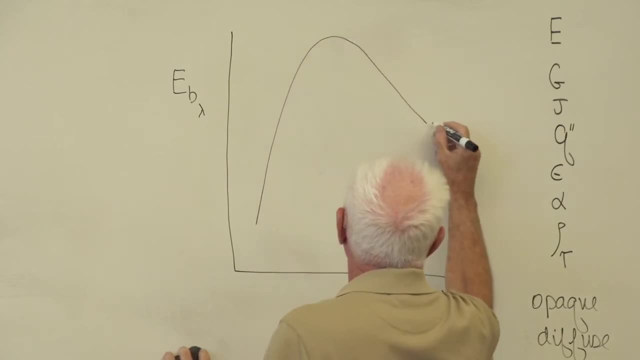 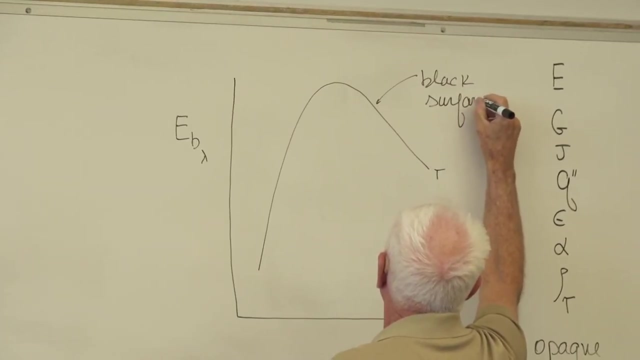 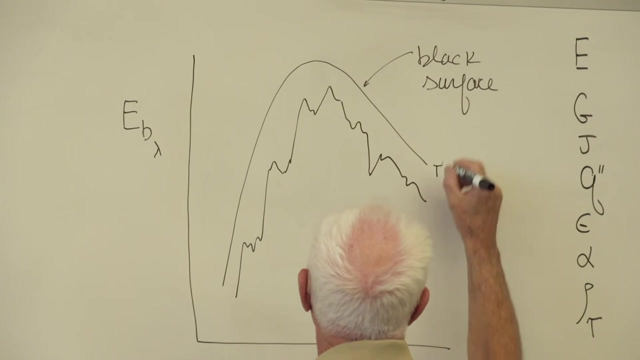 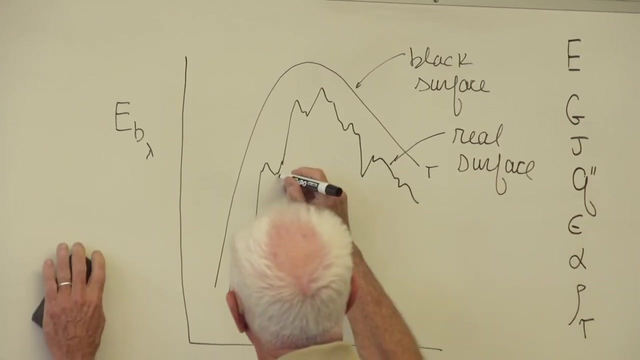 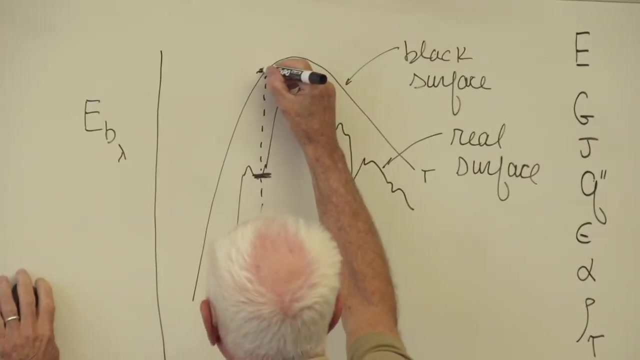 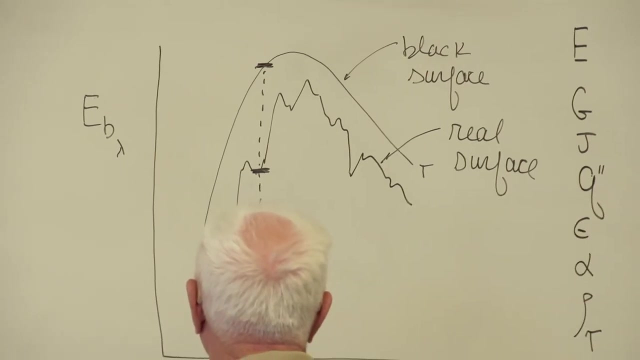 Okay, Okay, Okay. Black surface, real surface. If I take the ratio of these two guys here, If I take the ratio of these two guys here, If I take the ratio of these two guys here, Let's put lambda there. 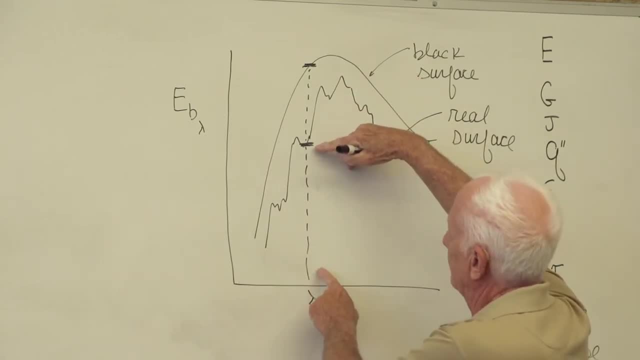 Let's put lambda there. Emissivity is this value divided by this value, Both of those same temperature, but one. the black surface here, the real surface here. So that's what that quotient is giving me. So that's what that quotient is giving me. 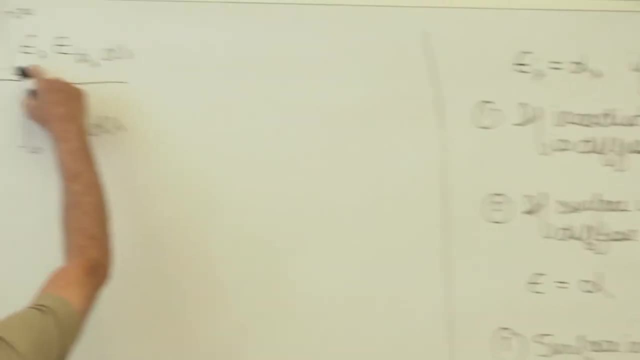 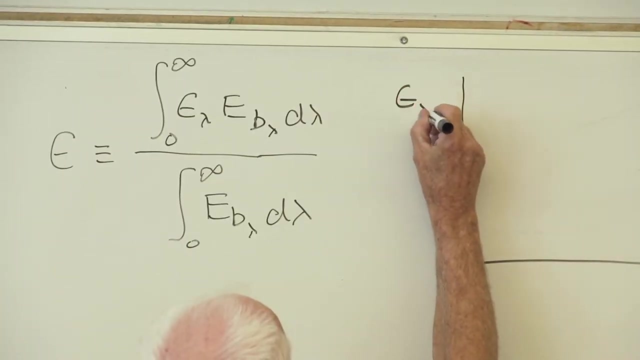 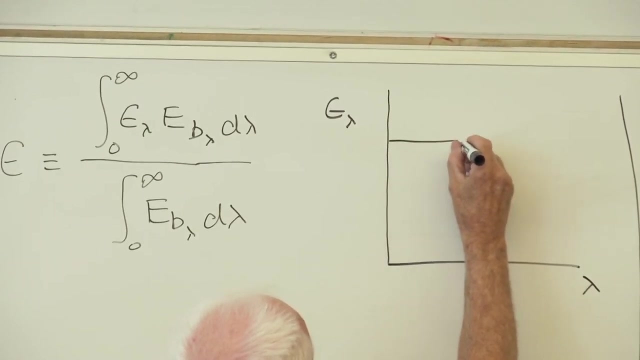 So that's what that quotient is giving me. Okay, That's where I get this guy here. I can get a graph then of this Epsilon Lambda- spectral emissivity versus Lambda, and maybe it looks something like this as a, for instance: 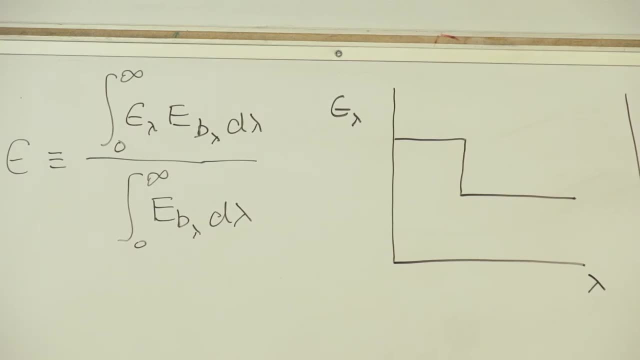 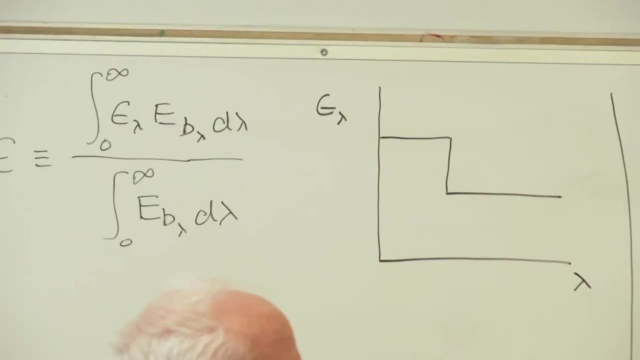 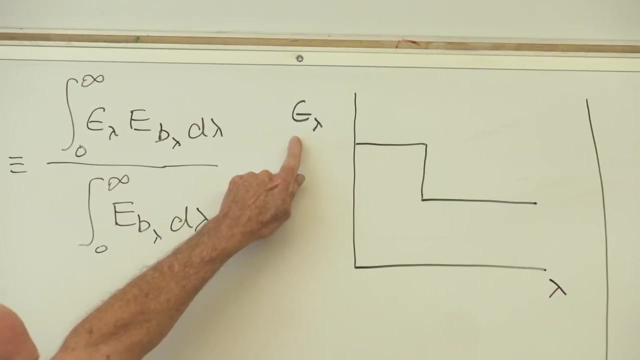 So somebody is going to give me a graph of that. maybe They found it somehow, Maybe by something like over there, from that graph over there. So they give me this and they ask me: I'm going to give you spectral emissivity, but I want you to give me emissivity. 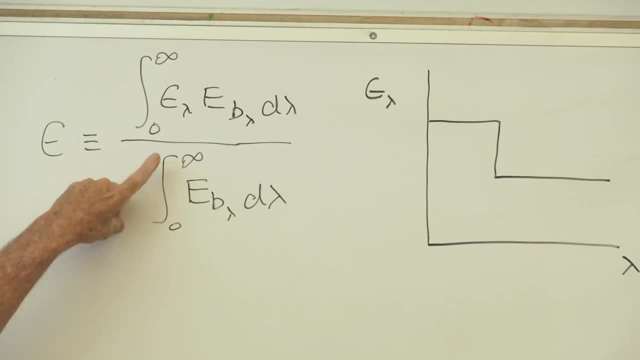 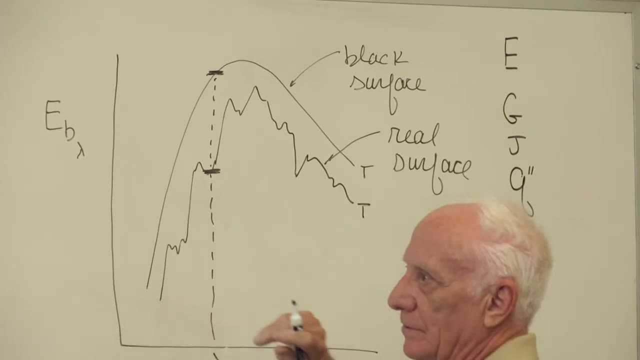 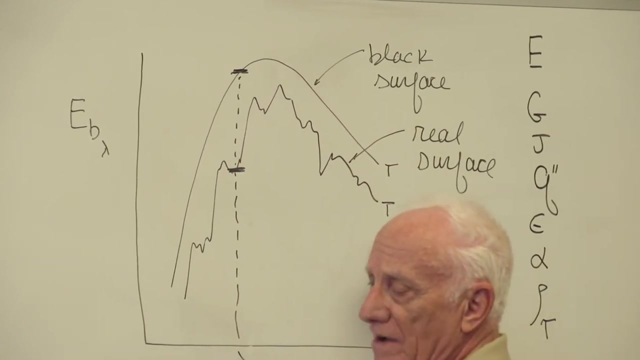 There it is. What is the numerator? It's like the area under this jagged curve. What's the denominator? The area under the black body curve integrating from zero wavelengths of zero to infinity. So it's the ratio of two areas. 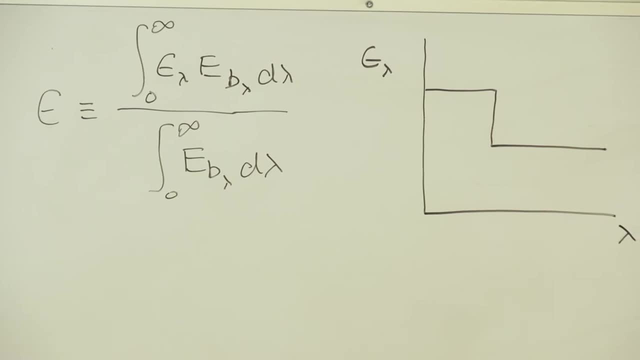 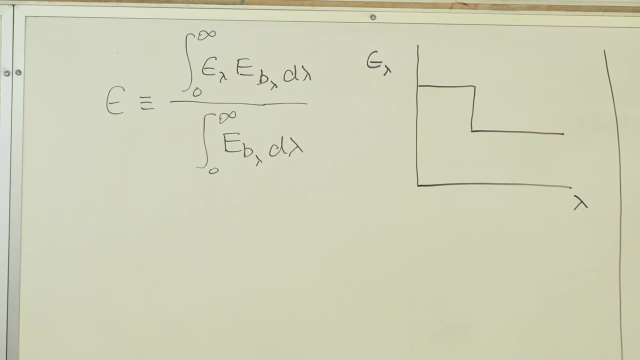 That's what we need there. I think that might be all we need there. Oh yeah, What equation? Because it's such a busy chapter, I'm going to give you the equation so that you know where to look in the chapter to find what I put on the board. 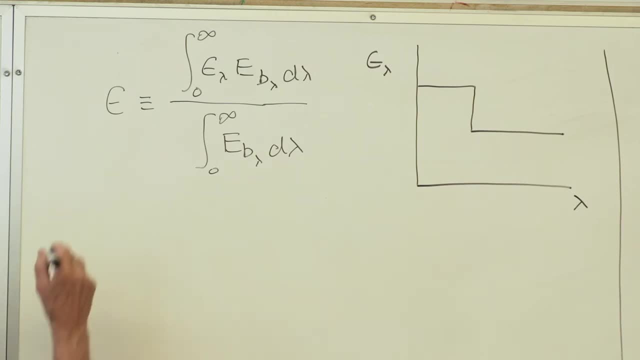 Equation 12.43.. Now, let's say you're trying to find Alpha. It's very similar to what we just did: spectral absorptivity. We don't use E anymore because absorptivity depends on the incoming radiation, So it depends on G. 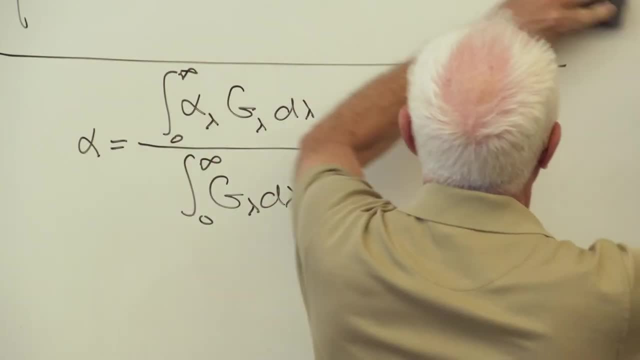 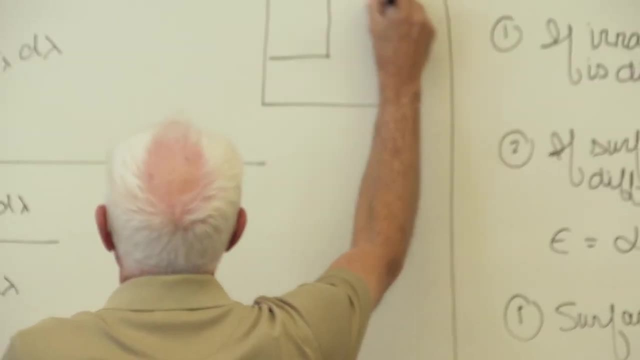 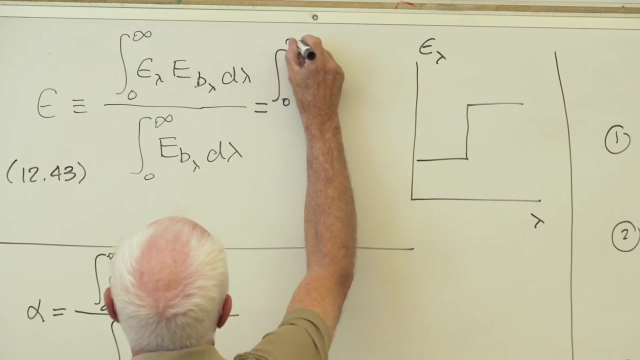 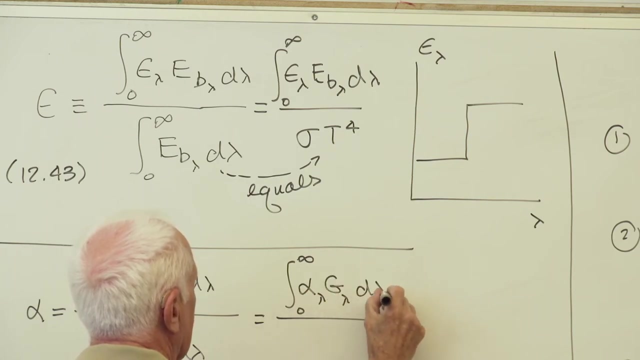 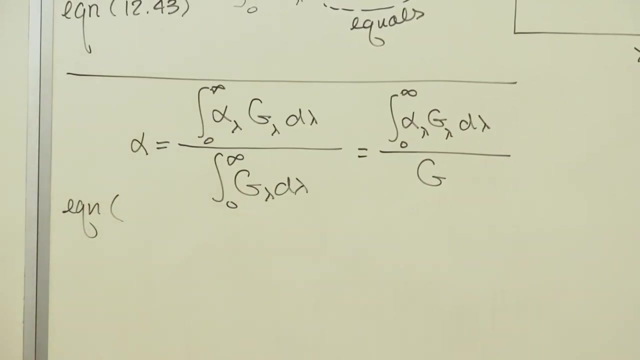 I'm going to move this over some. This guy is equal to Eb, Sigma t to the fourth, Sigma t to the fourth. Okay Now, this guy here then becomes Over G. Over G. Equation 12.52.. Over G. 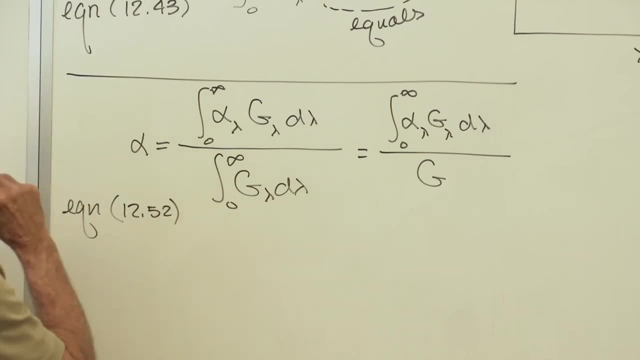 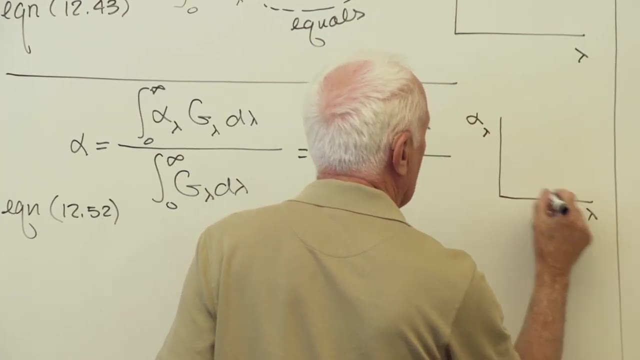 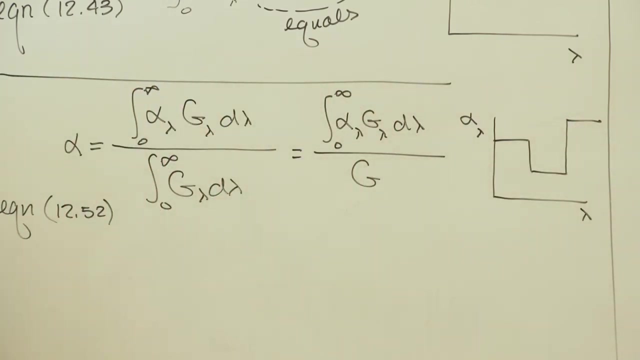 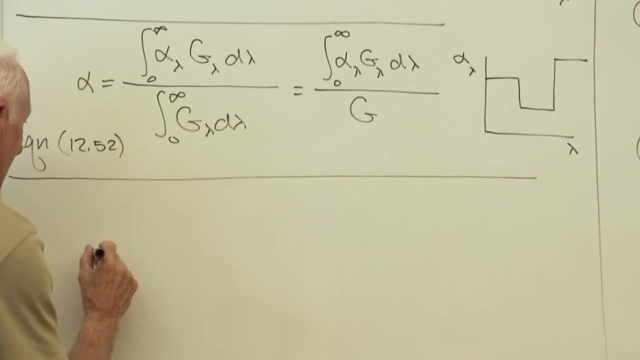 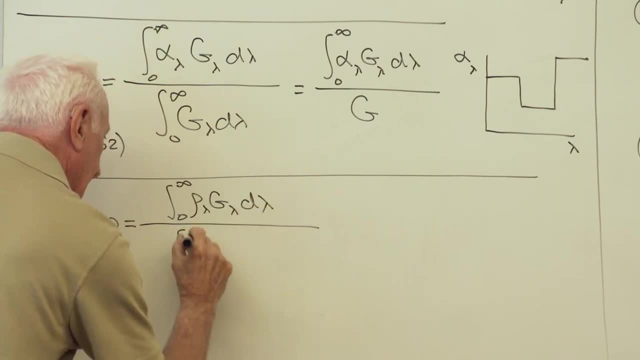 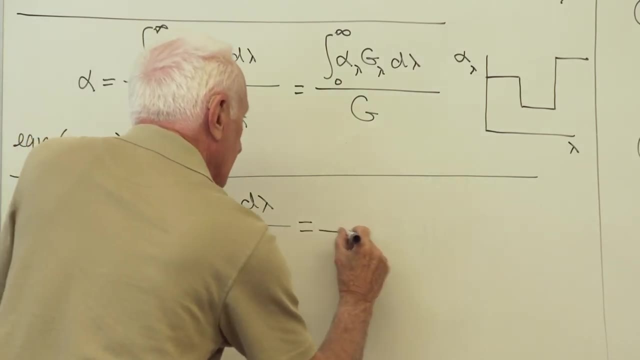 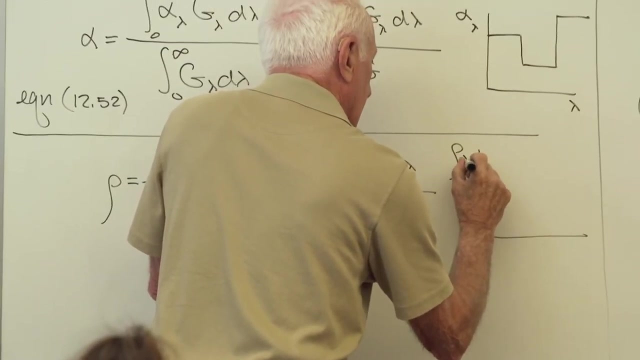 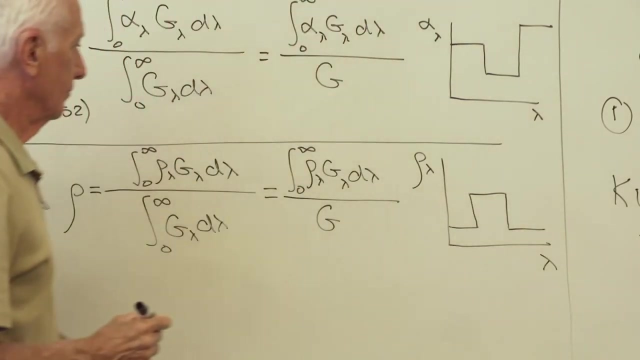 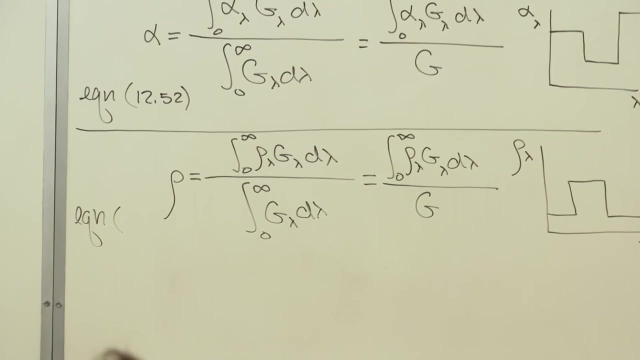 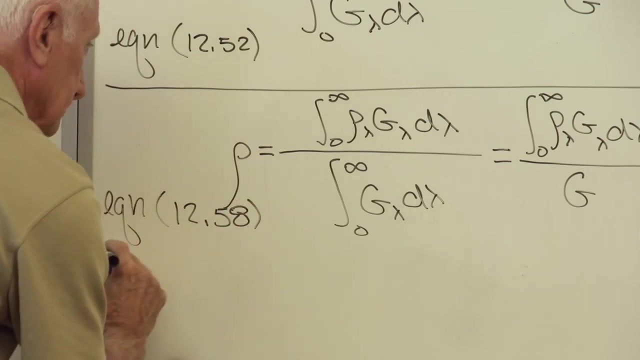 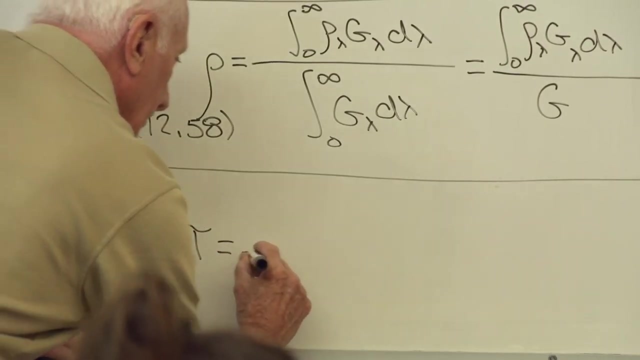 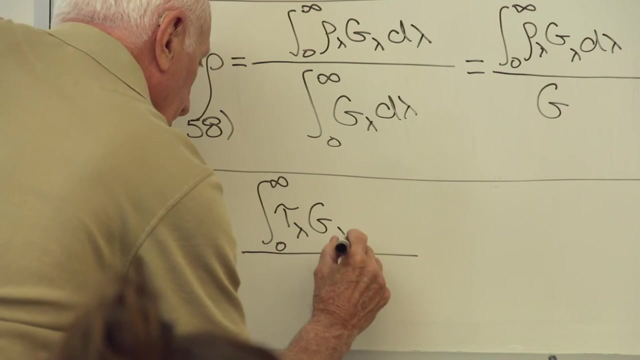 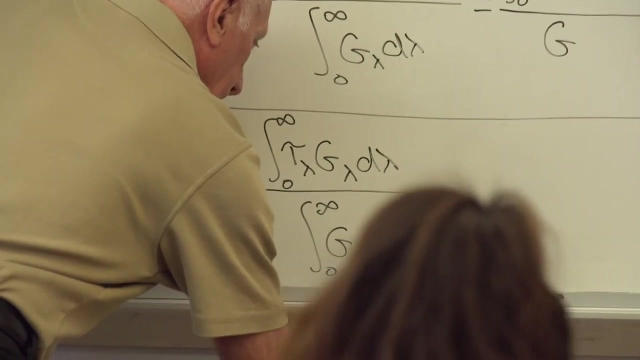 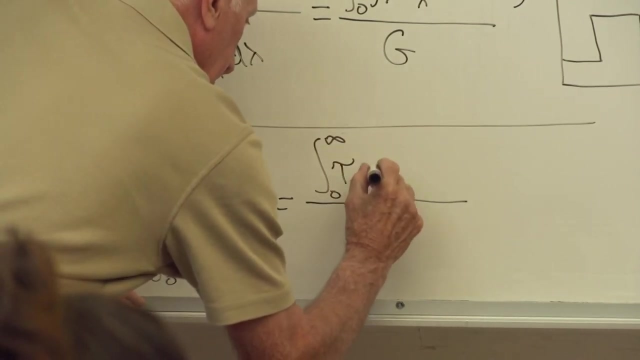 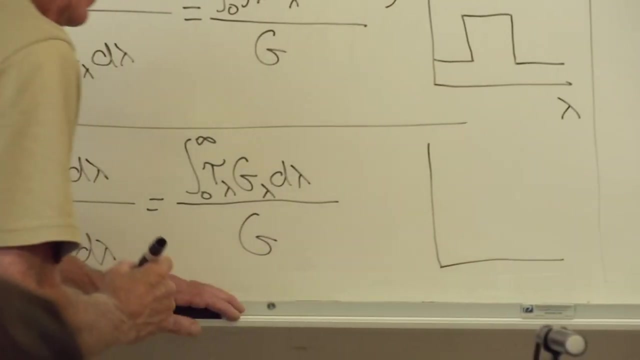 So that equation looks like this. You would use that if somebody gave you a graph of this. That's the equation for row 1258.. Then maybe you want to find the transmissivity tau. The person giving the problem gives you tau as a function of wavelength. 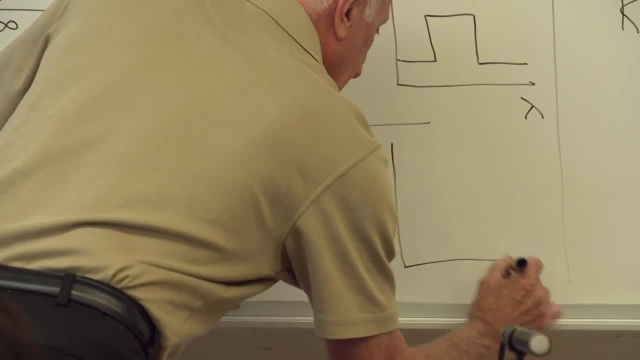 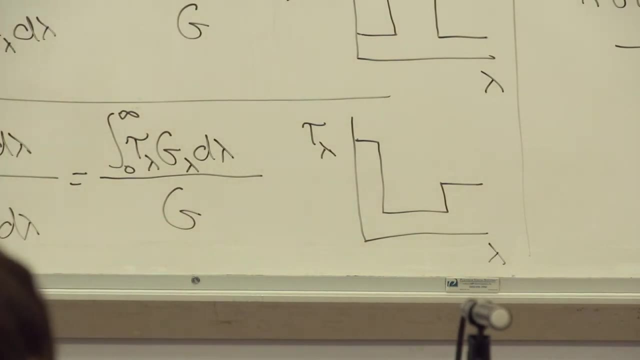 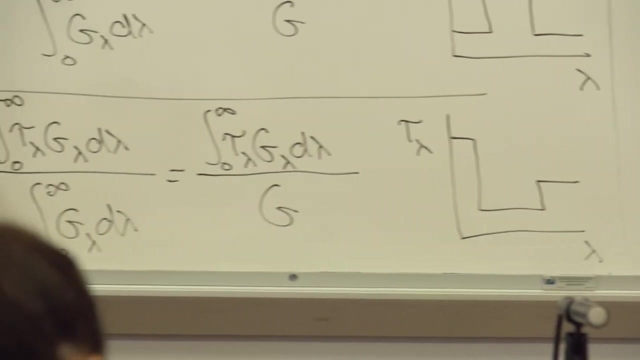 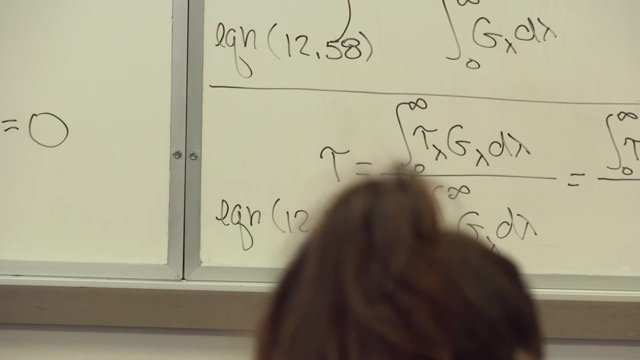 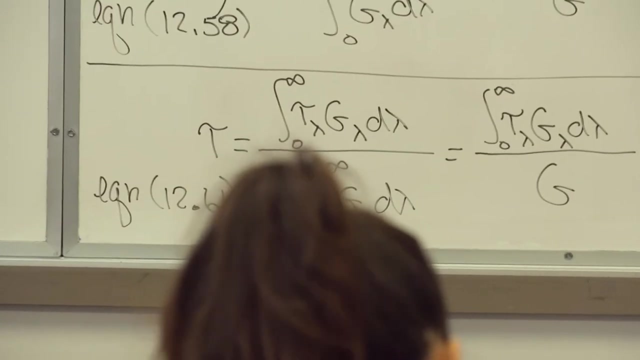 the spectral transmissivity as a function of wavelength, and it might look like this. So now equation 1261.. So now you have four different equations relating the properties epsilon, not relating but giving you the properties epsilon alpha, rho and tau. 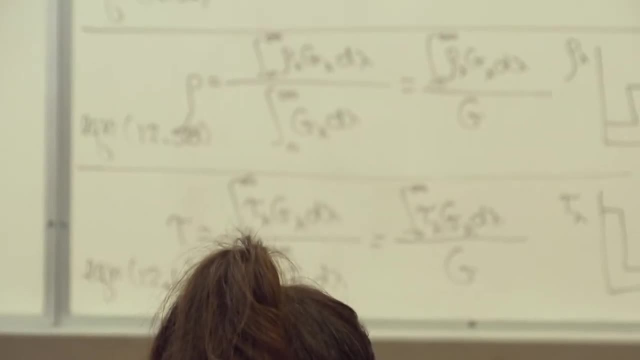 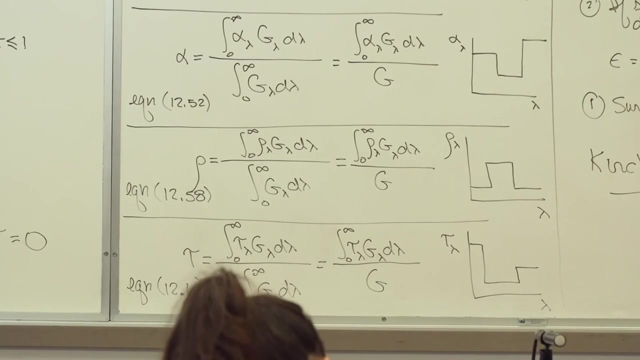 If you're given a graph of the spectral emissivity or the spectral absorptivity, the spectral reflectivity, the spectral transmissivity, you could then find those values of epsilon, alpha, rho and tau. Notice the g's in some equations. 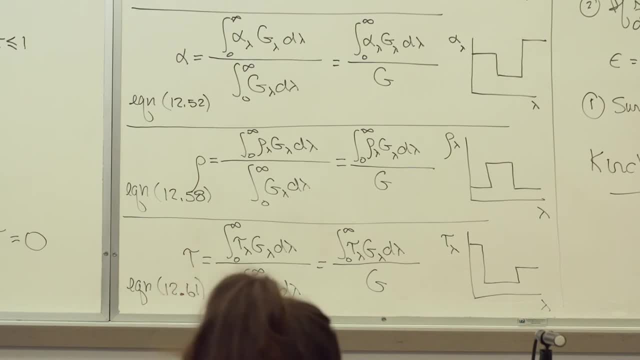 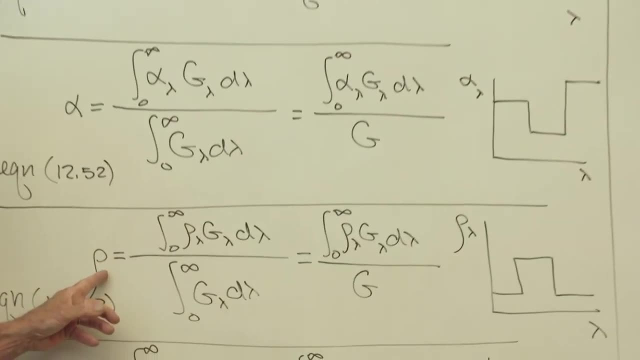 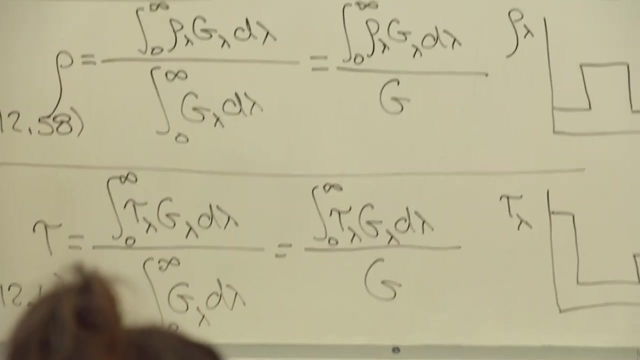 and the e b's in other equations. Absorption depends on what comes in g. Reflection depends on what comes in g. Transmission depends on what comes in g. Emission depends on the temperature of the object. e b. 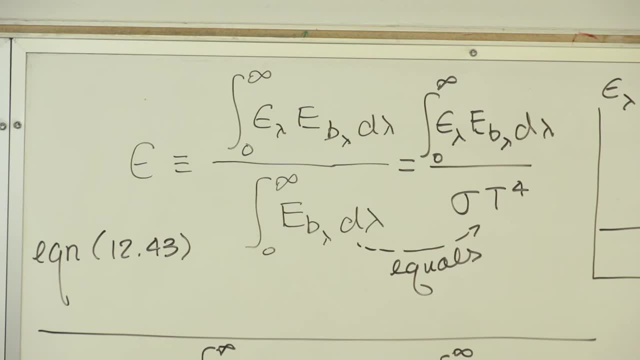 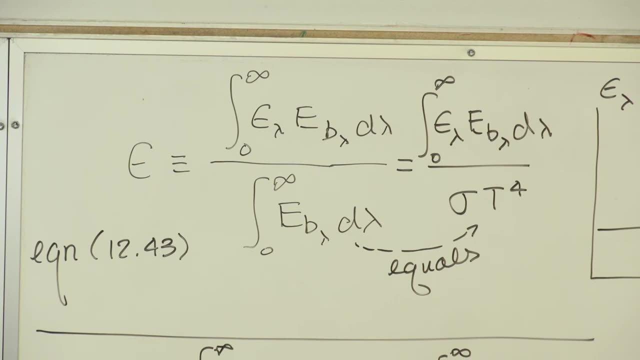 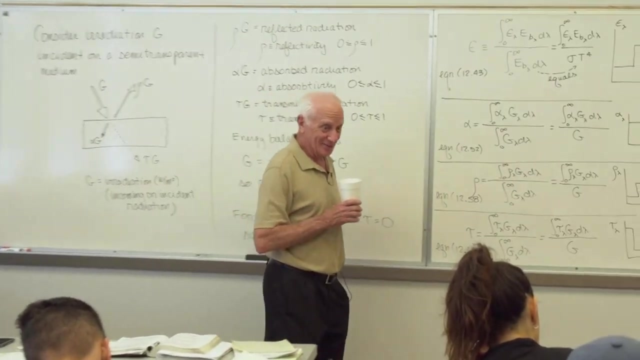 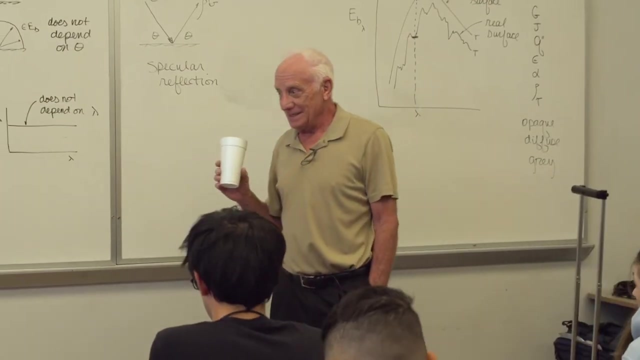 Emissivity depends on e, b. So now we have all those important equations. Now we've condensed what's in Chapter 12 now I did it on the board for you. Two days it took to condense it. But what was on the board last time and this time? 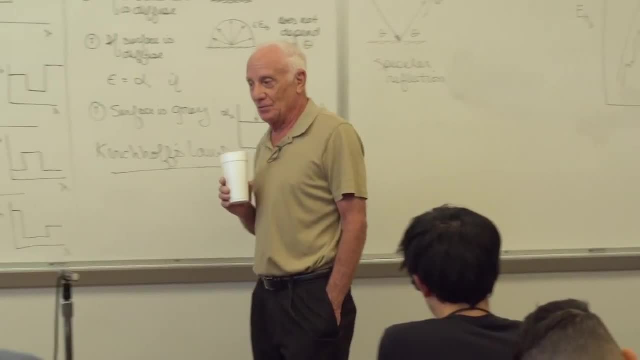 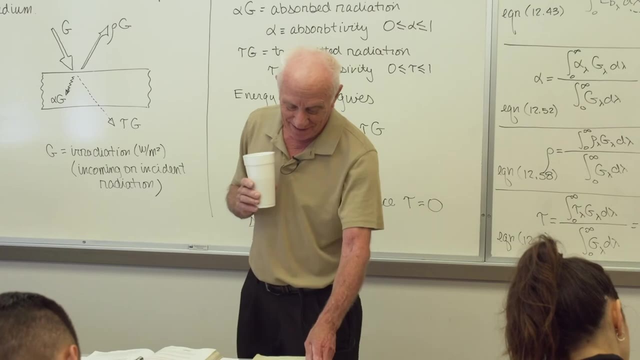 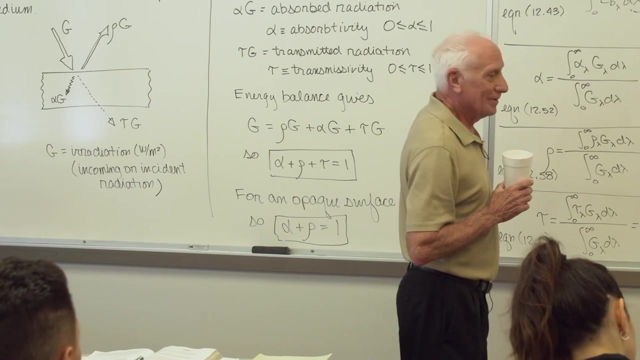 Wednesday and Friday. these are the important equations we're going to use in Chapter 12.. Chapter 12 is hard to read So, like I said, depend on your notes a lot, because that's what you need to focus on. Any questions on that then? 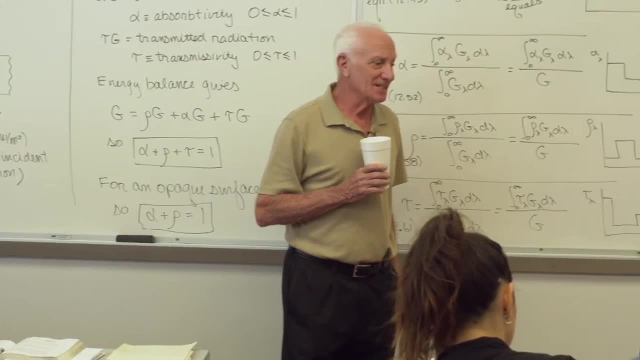 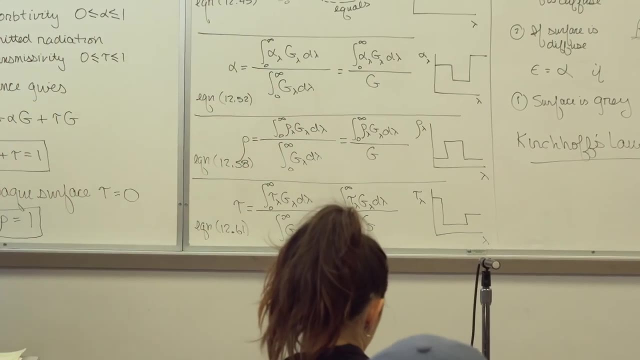 We're going to work examples, the next class being using these guys, So it's going to take the whole class meeting. So let's go over the homework that I passed back. right now. I have one question. When you wrote epsilon lambda equal to alpha lambda? 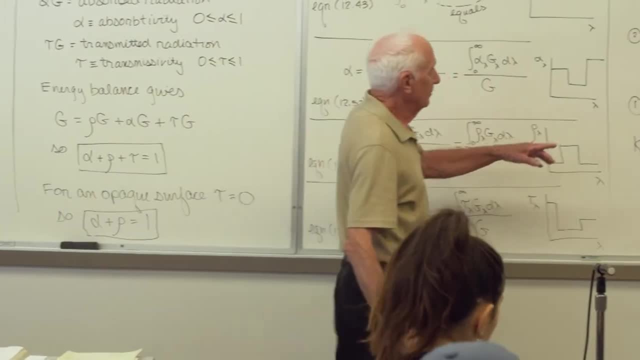 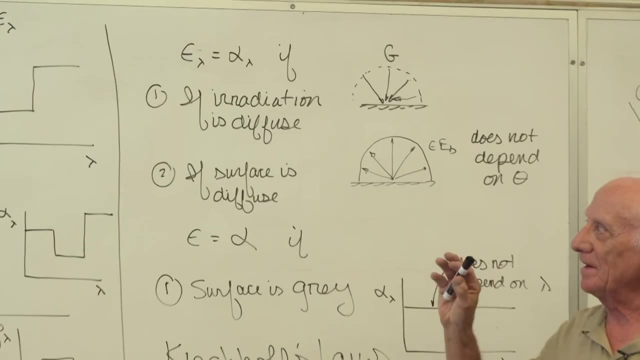 is that the whole function? Which one now? This one About that That one? yeah, What about now? Would that be the whole graph of epsilon lambda? Yeah, I'll give you a quick idea here. Let's say, the problem said: 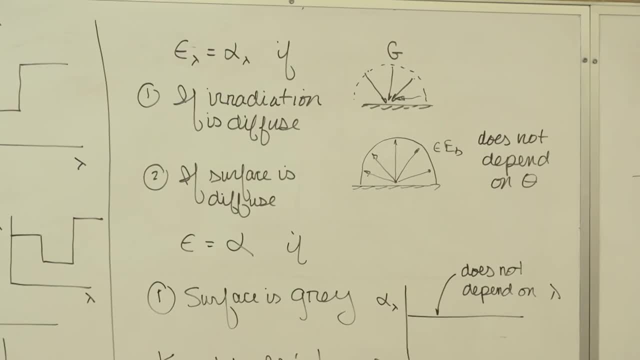 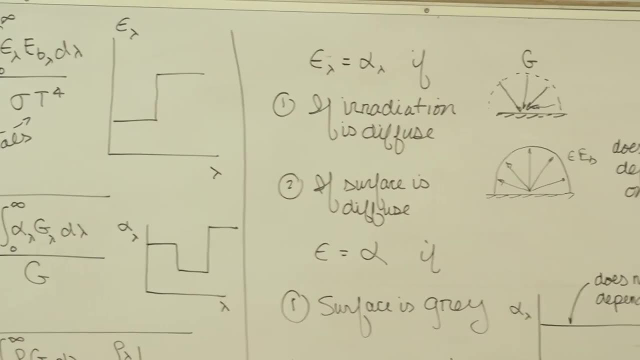 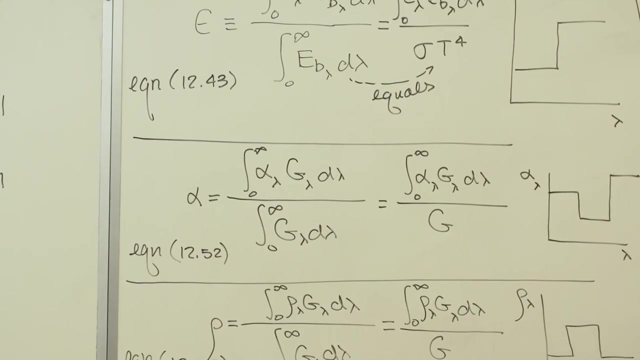 an opaque, diffused surface has a spectral emissivity graph like this: What is the absorptivity? What's the absorptivity? He gave me that graph: emissivity. If he tells me the magic words, the surface is opaque and diffuse. 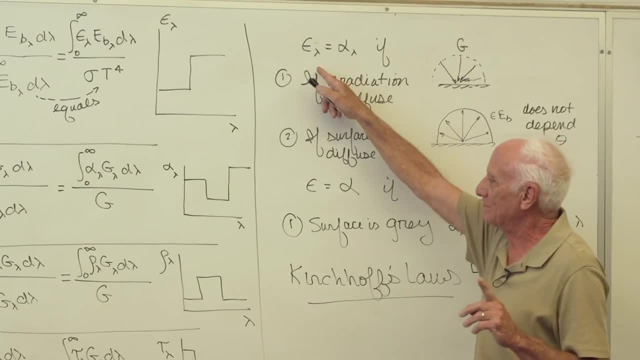 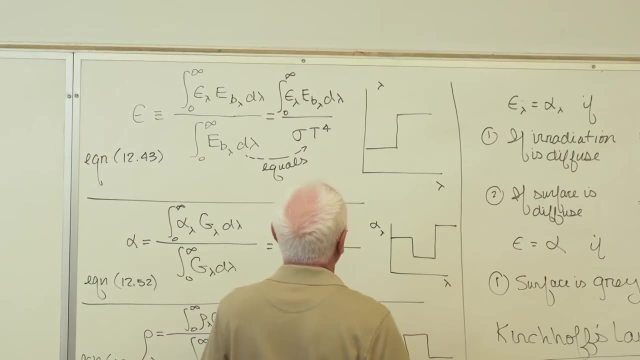 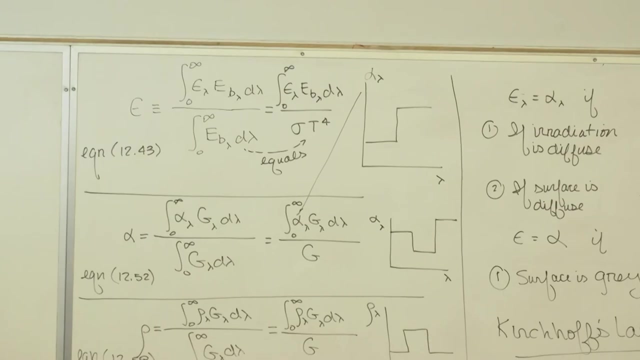 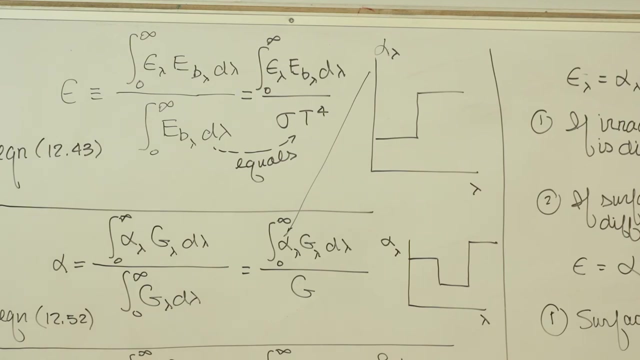 Surface is diffuse. If I have a graph of epsilon lambda, guess what I do? I erase this and I make this Alpha lambda. Now I put that guy in there. That's what I do, Anything else. then, on that, Let's take a look at the homework then. 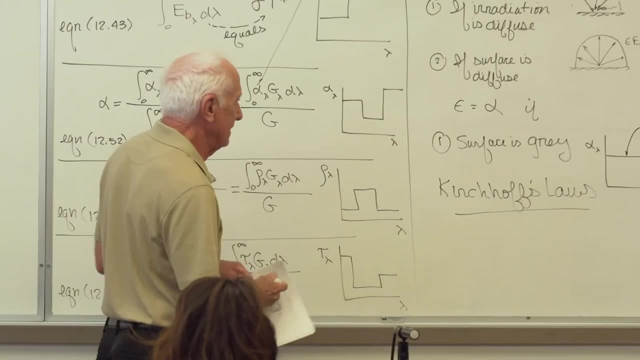 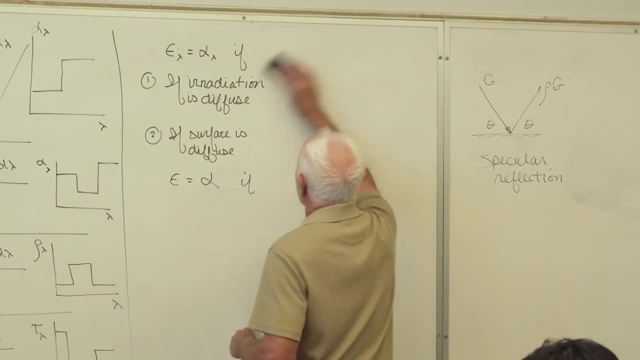 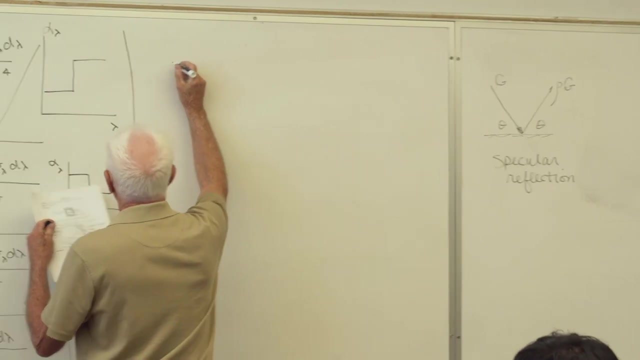 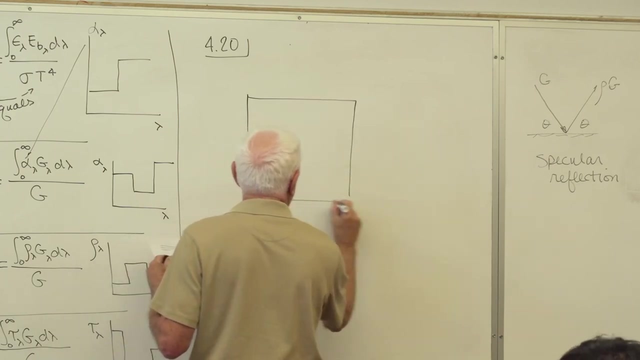 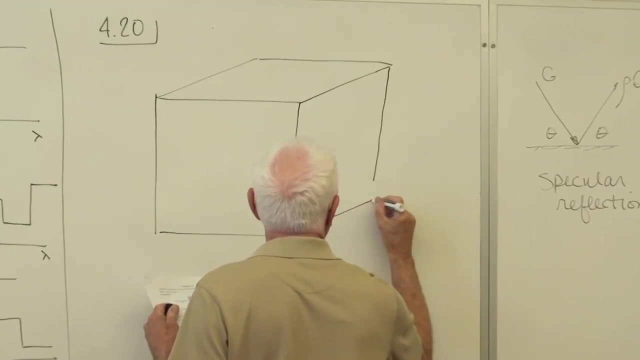 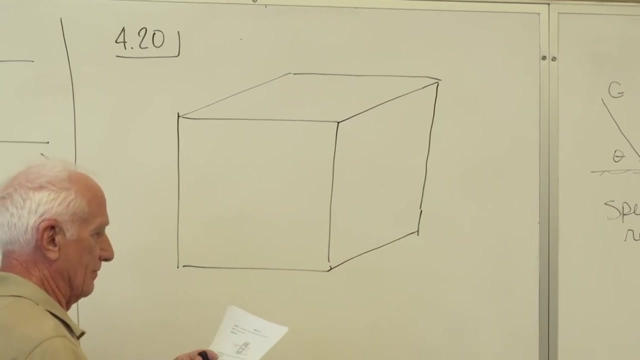 This was homework from Chapter 4, which was 2D, heat transfer, So I'm going to look at that first problem that I graded. It was a cubicle furnace. yeah, Okay, Let's do the outside first: 35 centimeters. 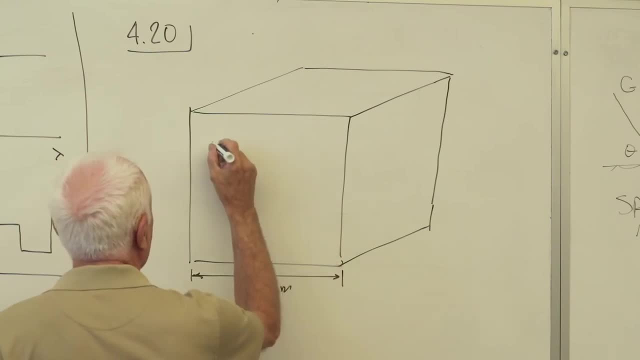 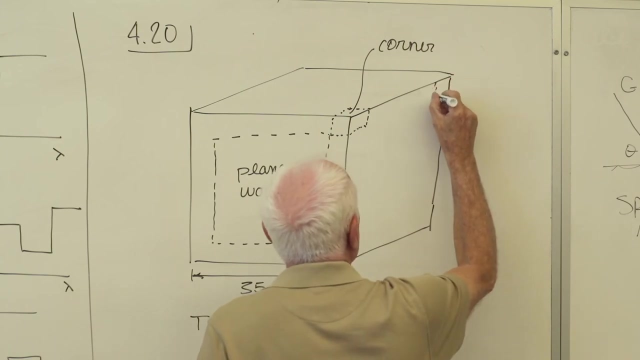 Okay, I'm going to break it down using Table 4.1.. Okay, This is a plain wall. This is a corner. Here's a corner. Here is an edge. Okay, Table 4.1,. I want to get S values. 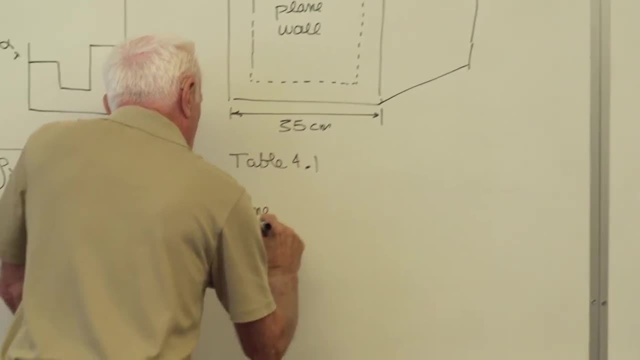 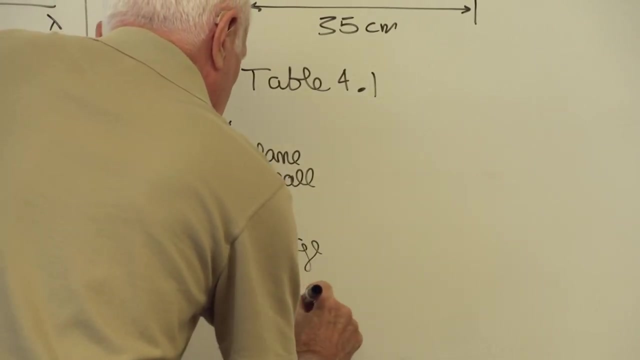 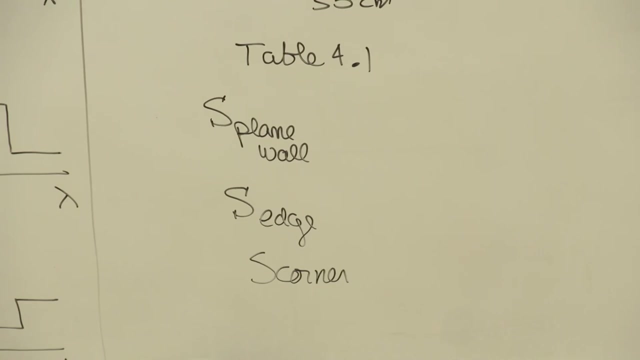 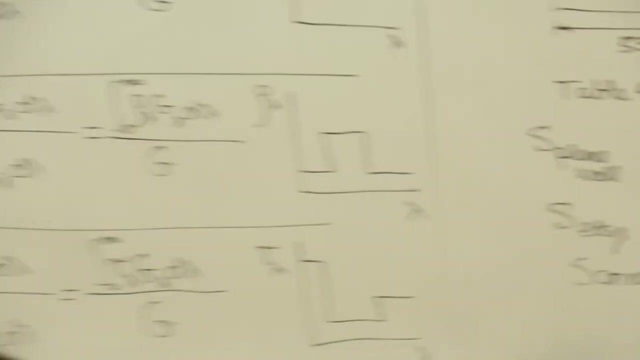 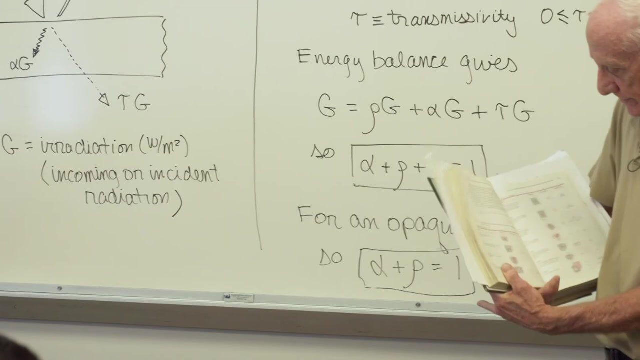 I want S for a plain wall, I want S for an edge and I want S for a corner. I'm going to use Table 4.1.. In Table 4.1, plain wall. I say I don't see plain wall in Table 4.1. 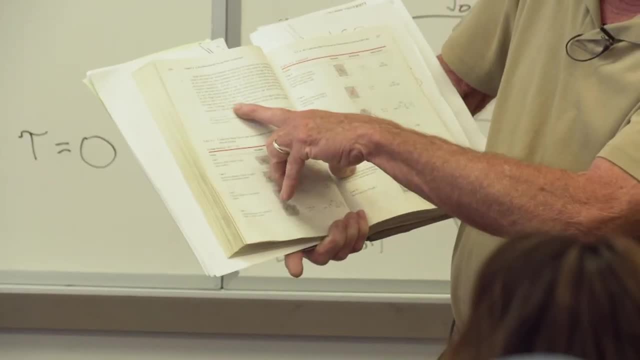 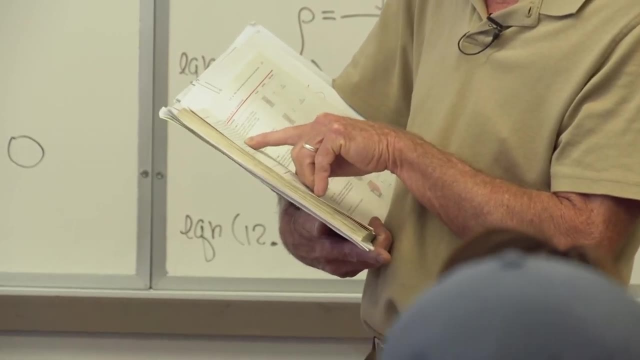 No, you don't. You got to read the words Above Table 4.1, here it is in the paragraph. The S value for a plain wall is A over L. The S value for a cylinder is given. The S value for a sphere is given. 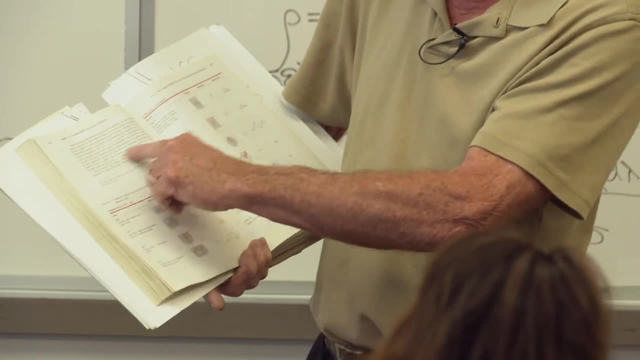 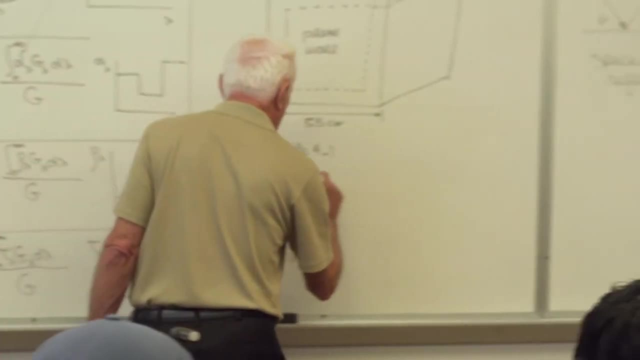 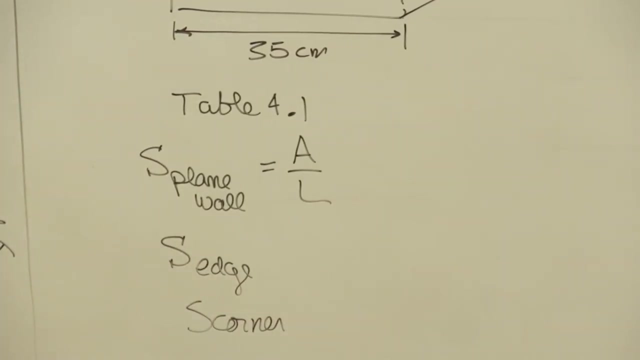 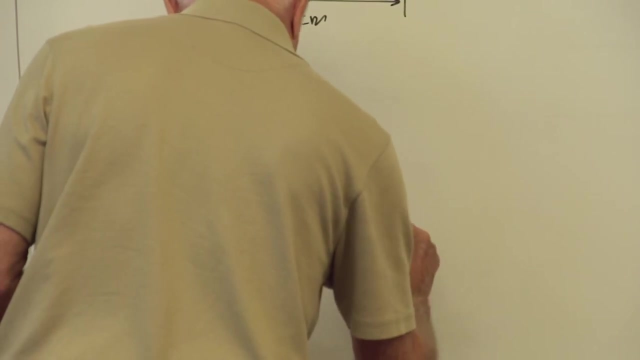 They give you three S values in the paragraph above, Table 4.1.. So for a plain wall, he says it's A over L. Okay, Let's get the edge. The edge is 0.54D, The corner 0.15L. 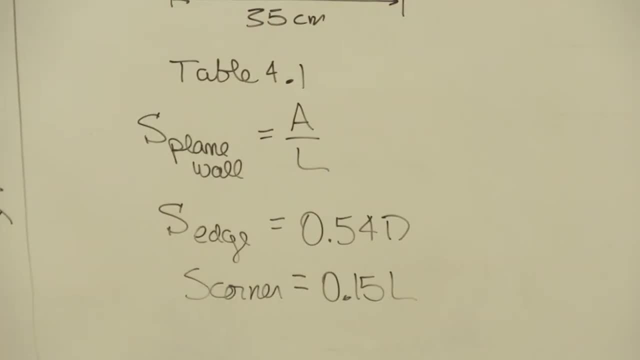 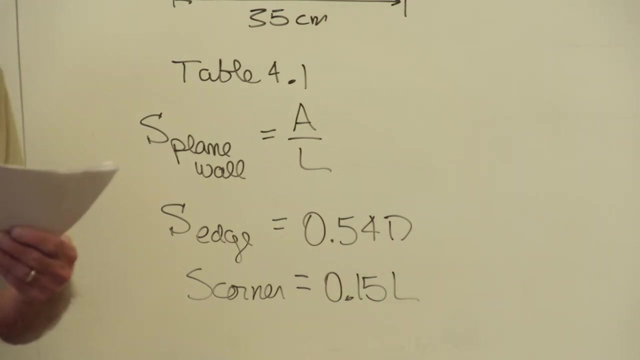 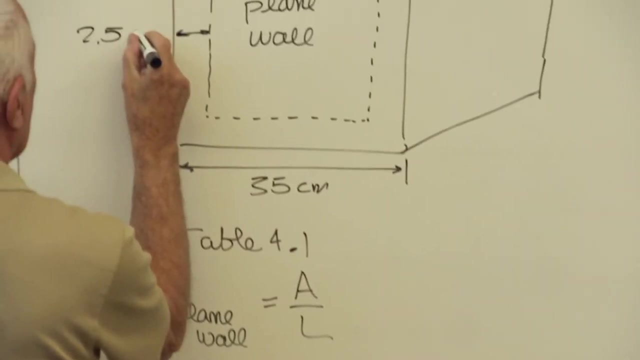 You have to check where it says the restrictions, So it makes sure the restrictions are satisfied. Yeah, they're satisfied. Change the problem. I said So. wall thickness: 2.5 centimeters. Two and a half centimeters all the way around. 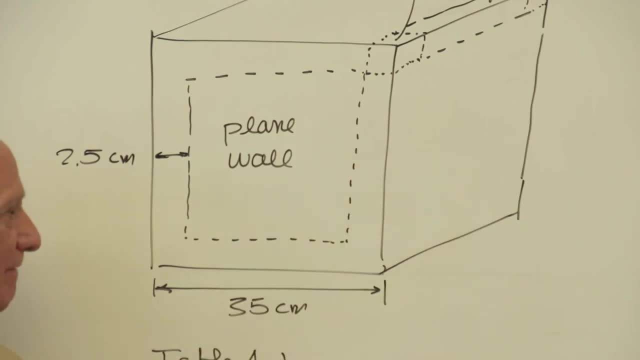 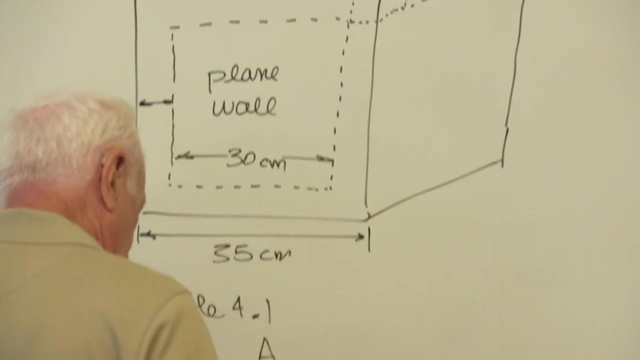 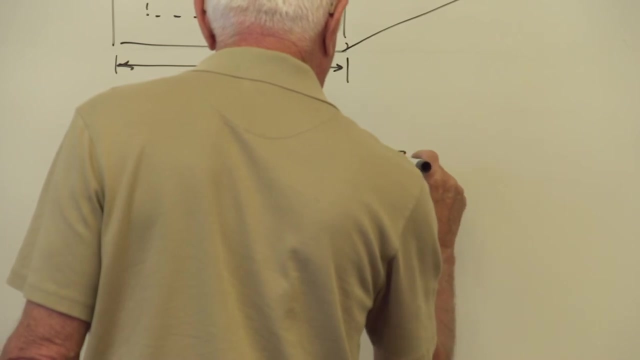 Thirty-five minus two and a half, minus two and a half 30, this guy, 30 centimeters, Thirty by 30.. Thirty by 30.. This guy is 3.6.. L is a thickness: 0.025.. 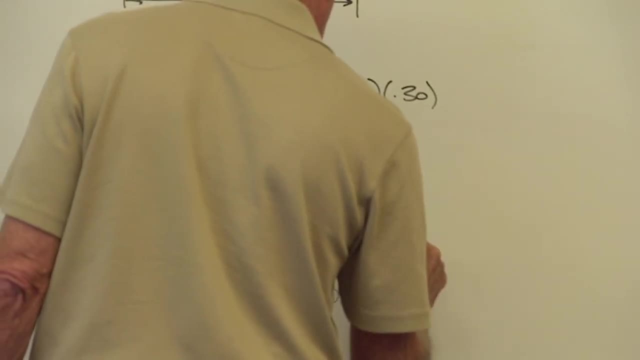 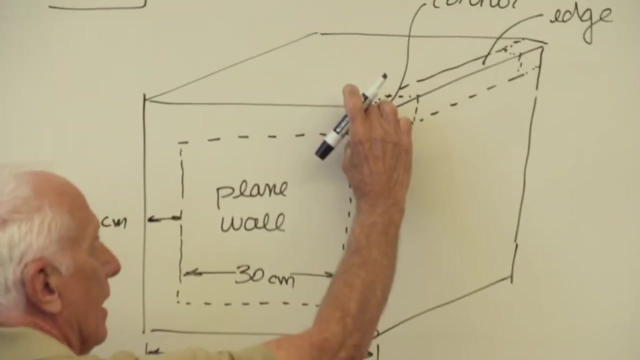 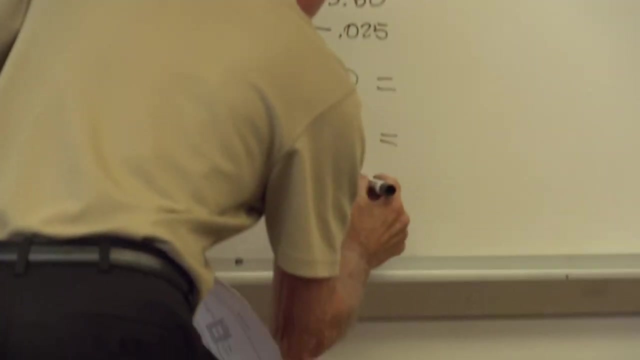 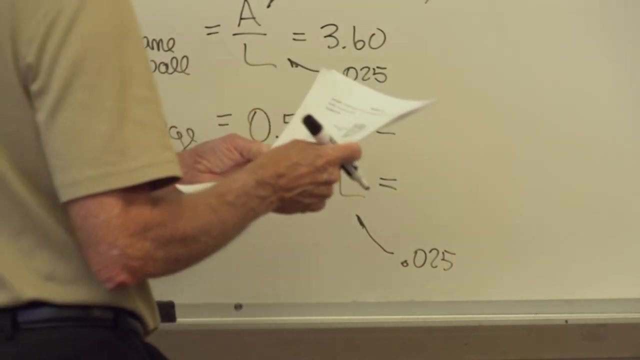 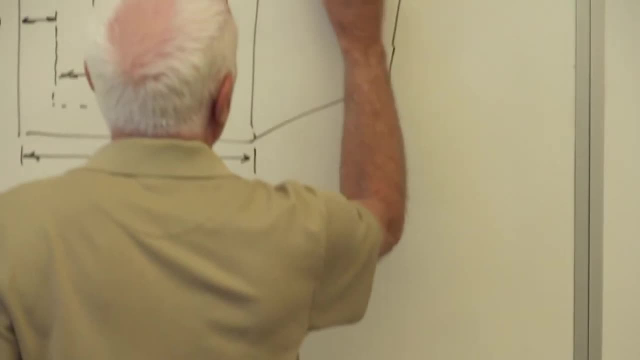 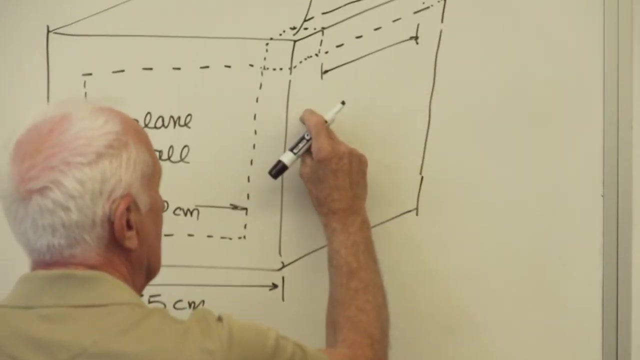 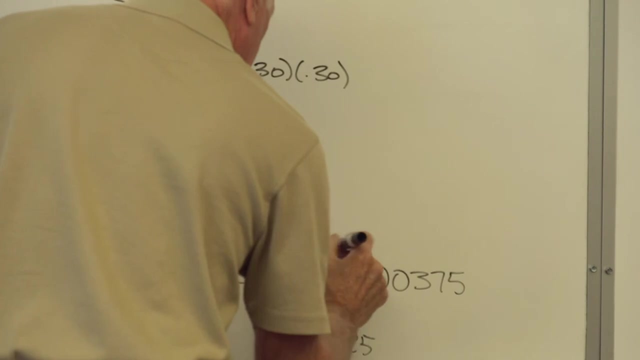 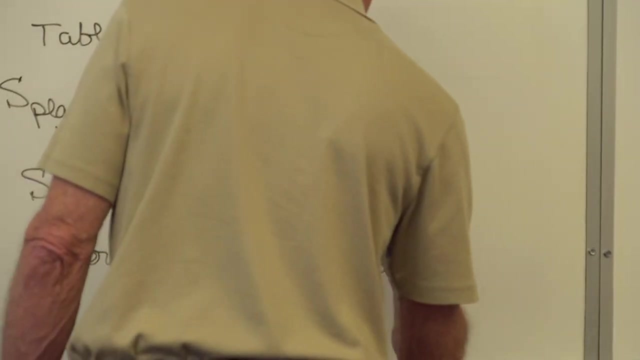 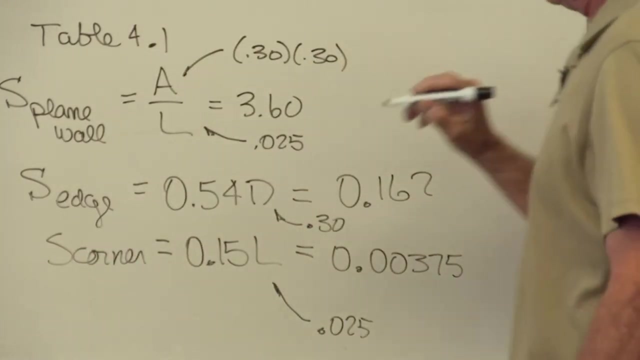 Okay, Edge, add distance there to there 0.35, or 35 minus two and a half. minus two and a half he's 30.. D is 30 centimeters and that is 0.162.. Okay, There are six plane walls. 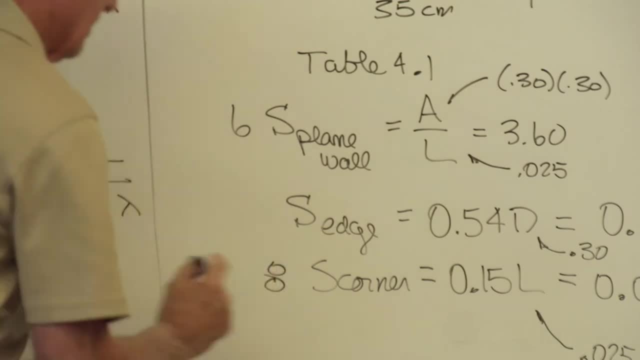 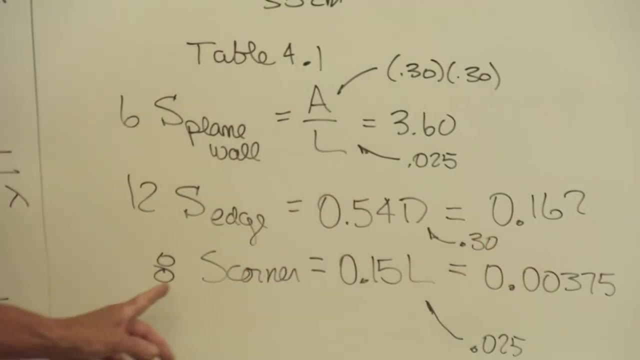 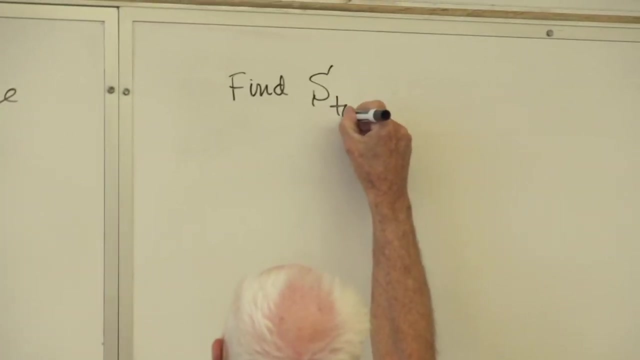 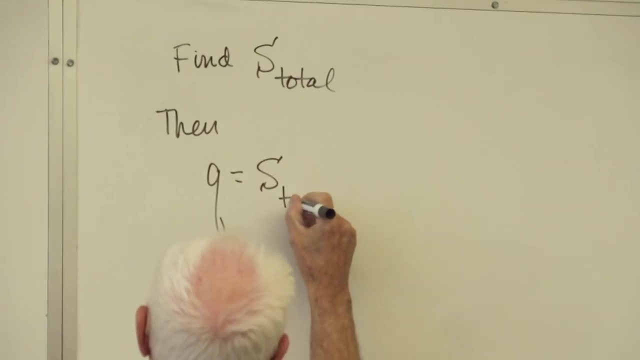 There's eight corners, there's 12 edges. Okay, Six times that number plus 12 times that number plus eight times that number equal S total. Okay, Okay, Okay, Okay. Then Q equals S total times K Delta T. 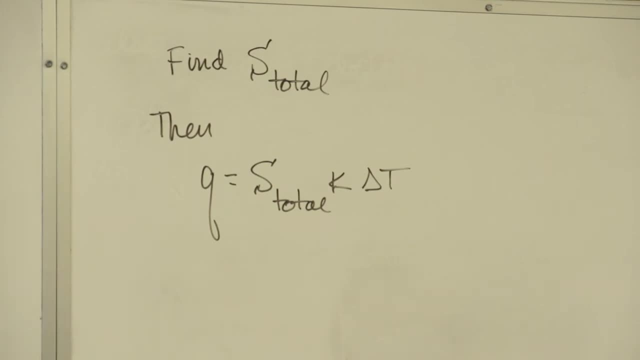 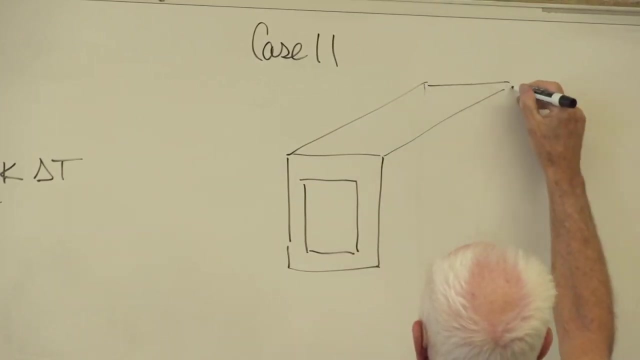 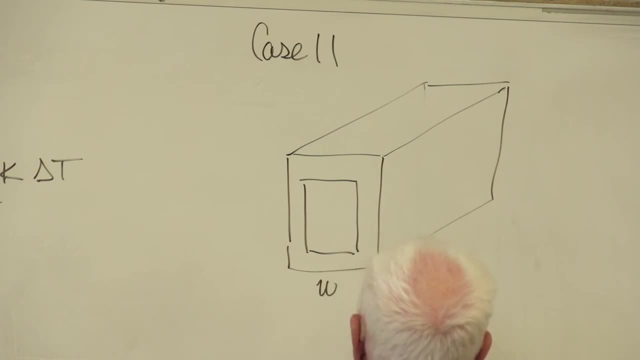 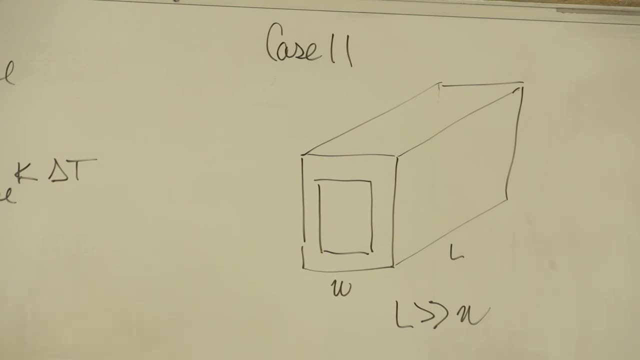 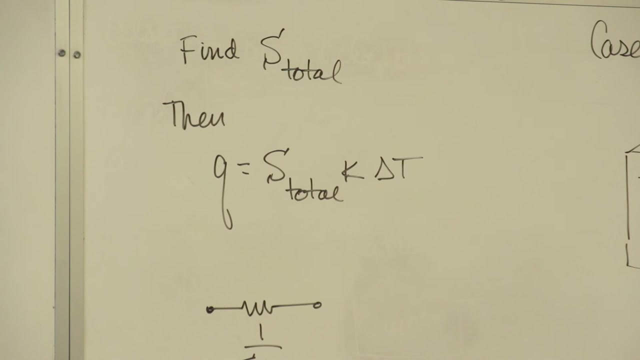 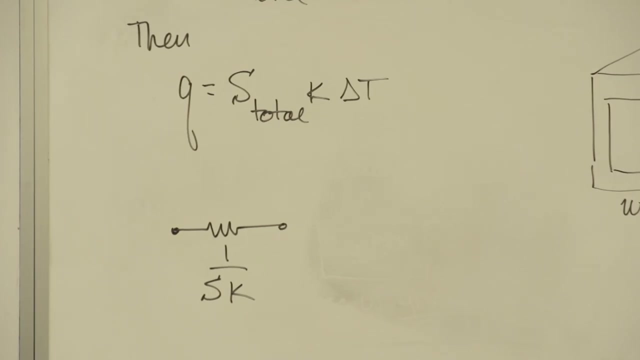 Okay, cannot do. No, No, No, No, No, No 1 over SK. Why would you want it? Well, I hate to give away good problems for exams. I won't say anything. but what if there was convection on? 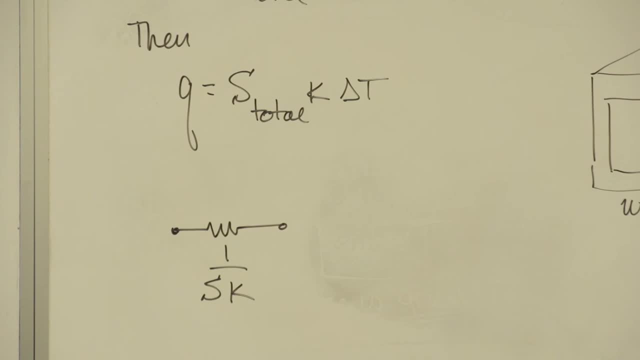 the inside, the outside, Hot gas on the inside, room temperature on the outside. Now find Q: How many resistors? Three, two convection, one conduction. Yeah, that's why you use resistors sometimes if you need to. 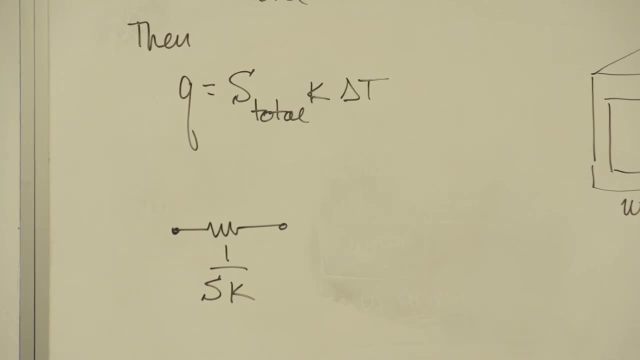 If you need to. Second problem: it's pretty straightforward. I'm not going to put that on the board here. There's two resistors there, one for the soil and one for the insulation. Just add them together and it's pretty straightforward. 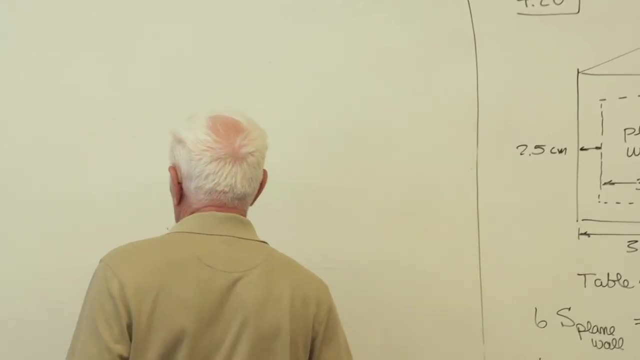 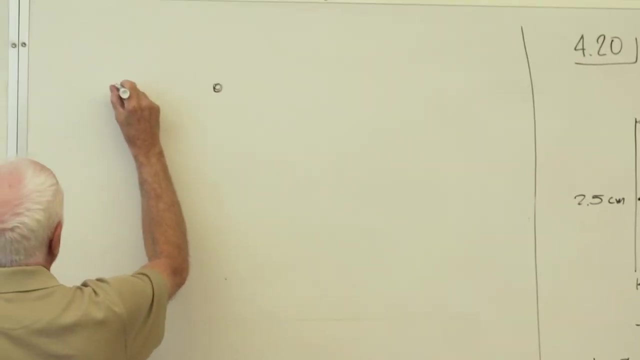 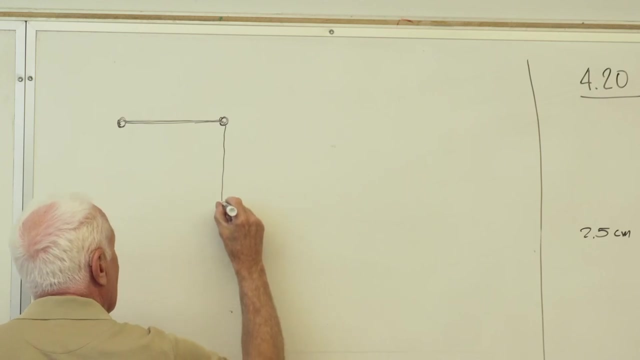 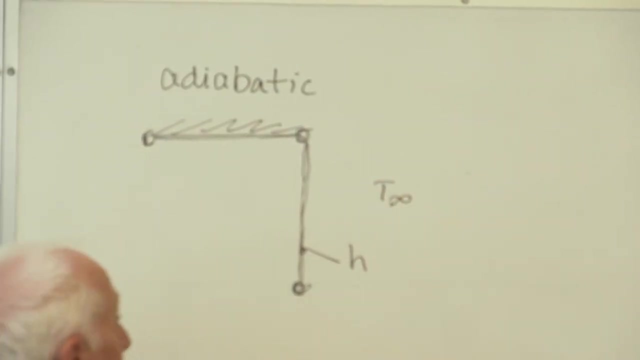 But I look at the third problem, which is derived, the finite difference equation for a corner node. So here's my corner node. This side of it is adiabatic. This side has convection to fluid temperature T infinity. I'm not going to. 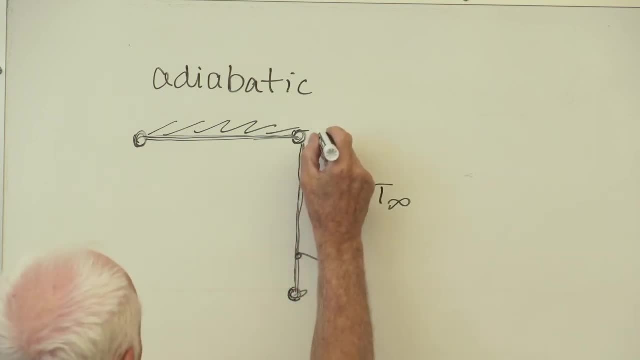 to use. I'm just going to call these guys node 1,, 2, and 3.. I don't want to make double subscripts for that simple case, but for the problem for homework you got to use double subscripts. 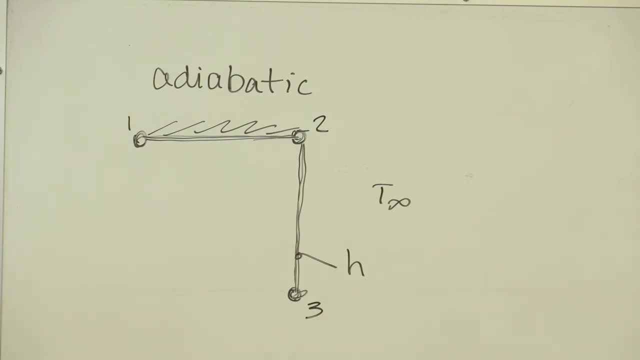 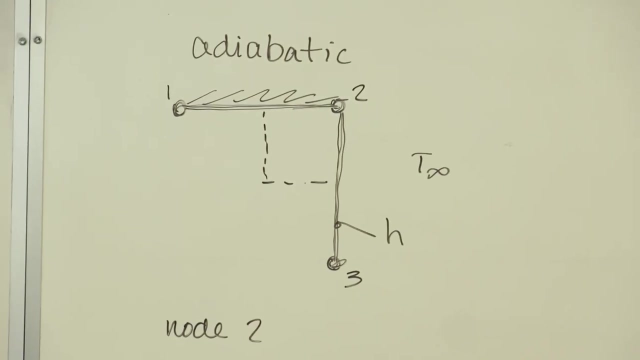 Okay, fine, but I don't want to make it more complicated than it is. All right, node 2, here is the material that node 2 replaces. There it is. Tell me where the heat goes. Don't forget the rule now. 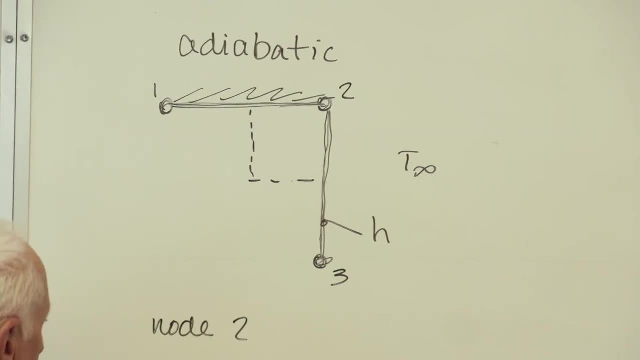 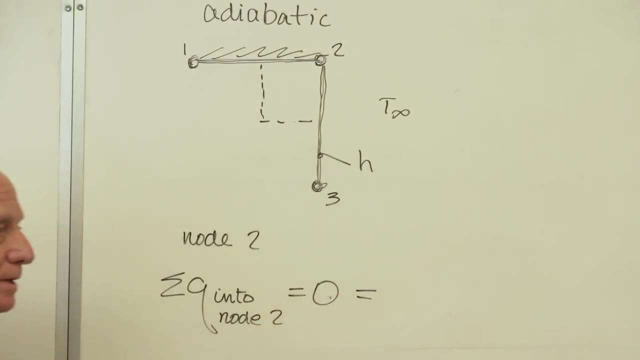 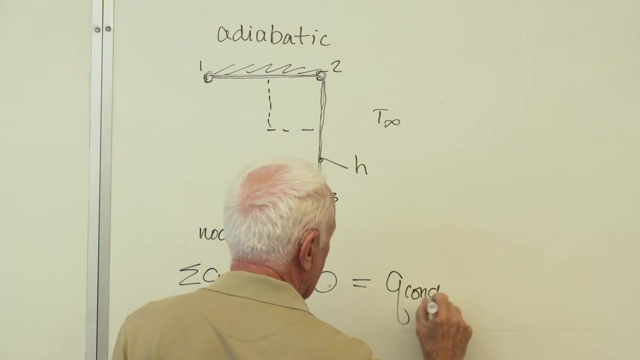 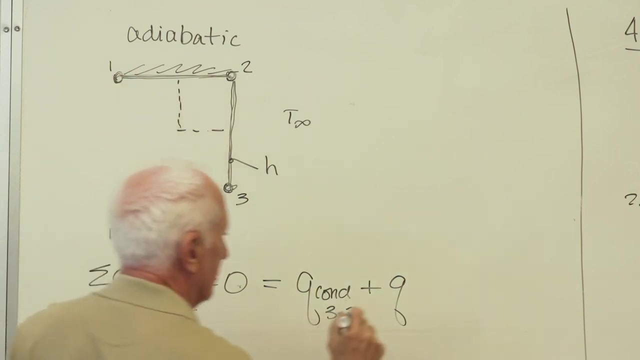 Summation of the q's into node 2 equals 0.. What comes into node 2? Conduction from 3 to 2.. What goes into node 2? Conduction from 1 to 2.. What goes into the wall here? 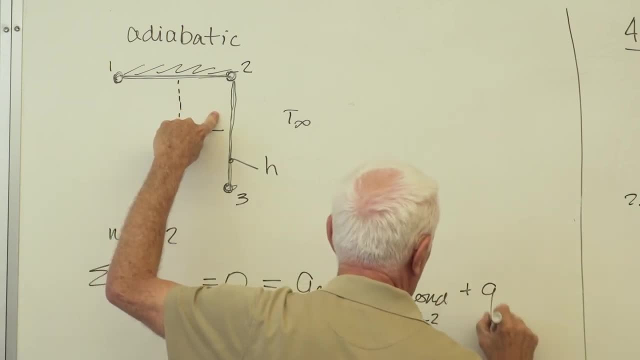 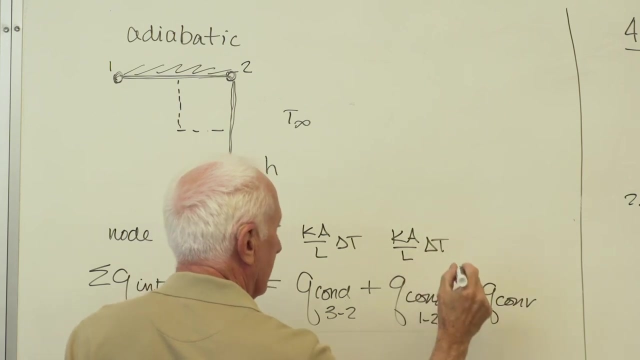